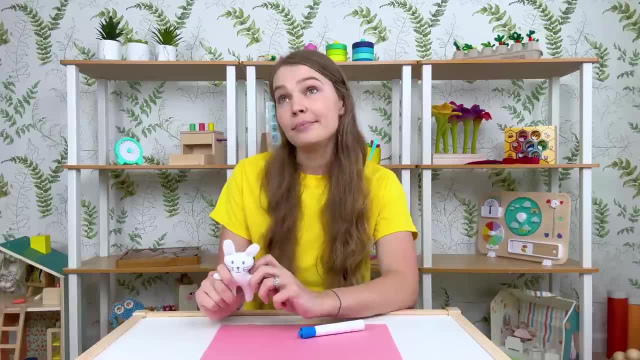 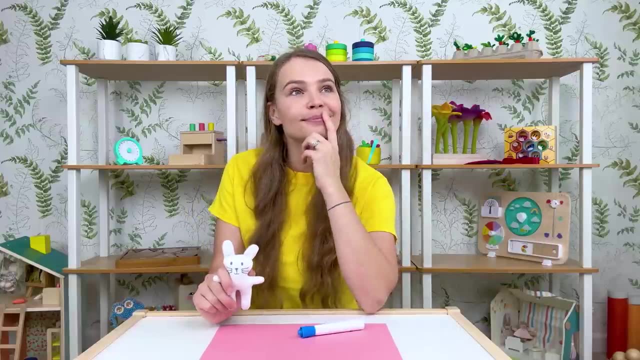 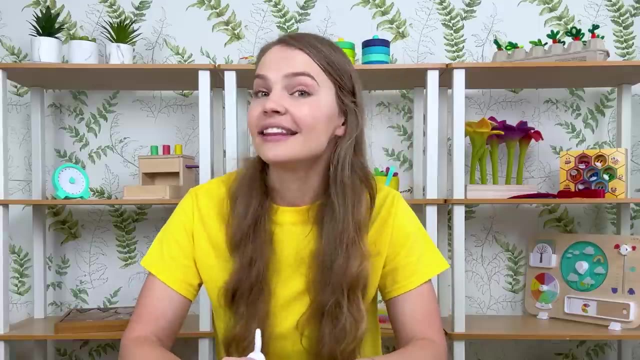 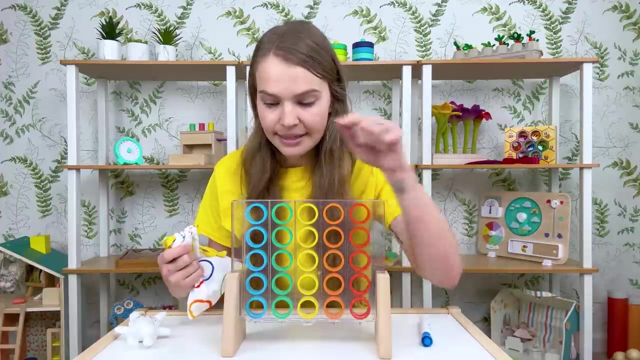 you can find shapes anywhere you go, Like some pillows look like squares and a door looks like a rectangle. Hmm, A cup kind of looks like a circle. huh, Let's learn about some shapes together. First, let's learn about circles. I've got a fun circle game for us to learn. I've got this fun game There's. 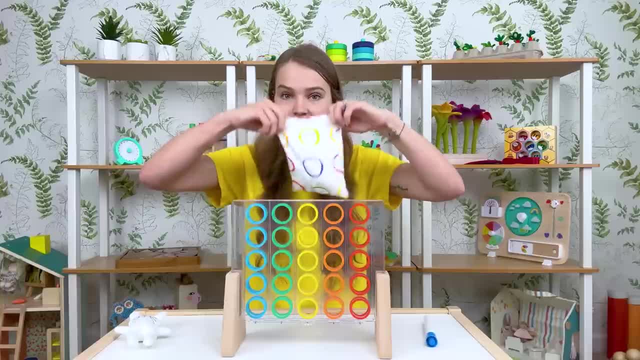 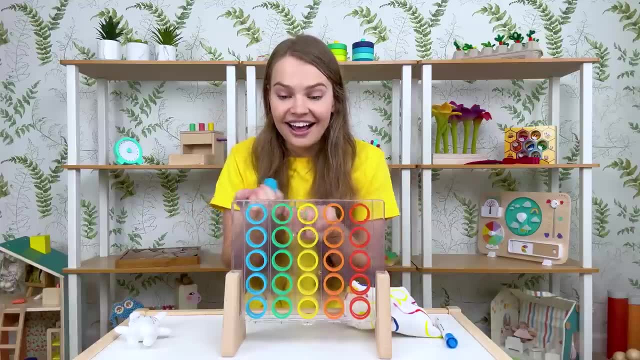 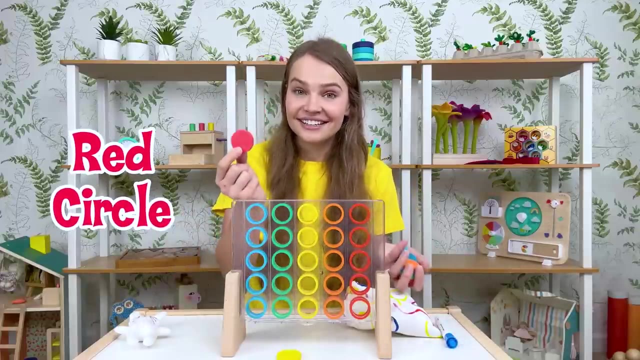 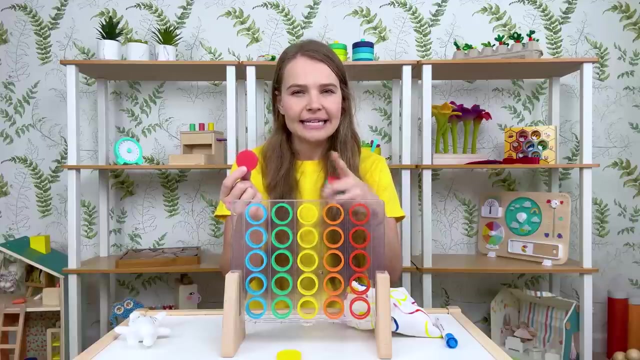 different color circle spots And I've got a fun bag of circles And they're all different colors. Wow, Let's see, I'll put the red circle. Hmm, Should I put it in the blue, green, yellow, orange or red, Red? All right, 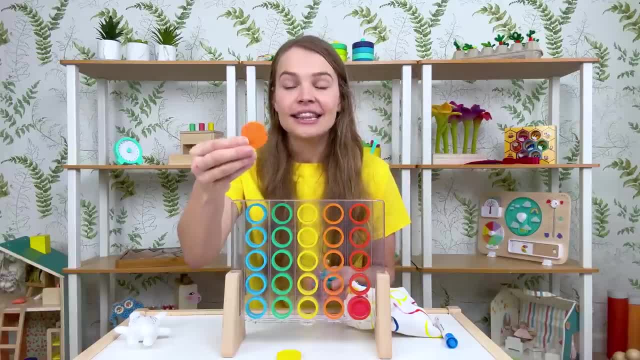 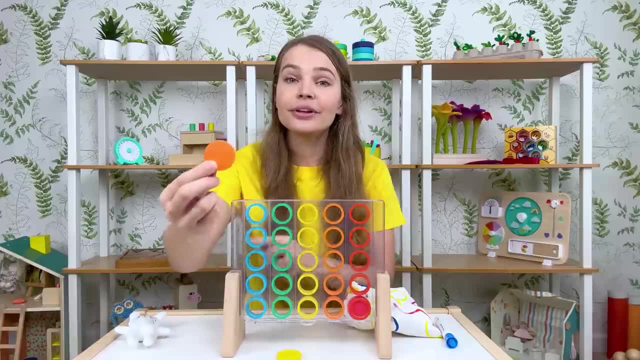 here we go. Now it's your turn. This is an orange circle. Should we put it in the red, orange, yellow, green or blue? Where should we put it In the orange? I'll put it in for you. Here you go. 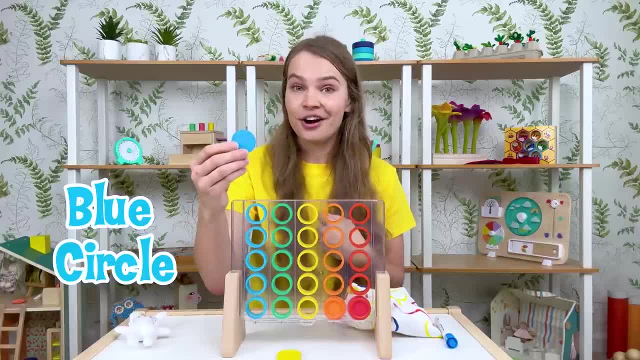 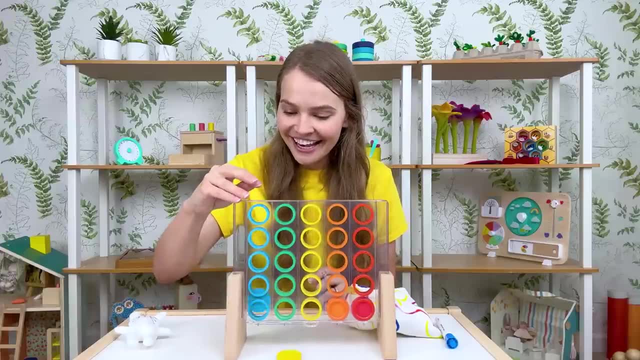 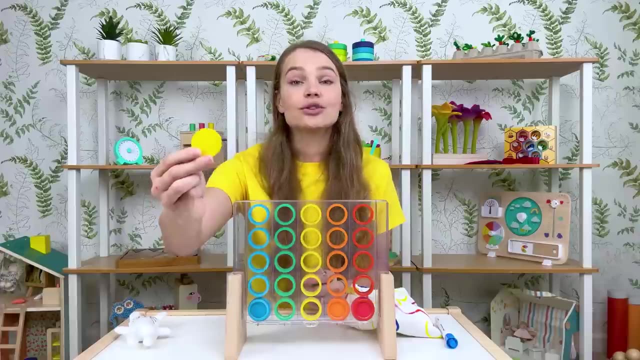 All right, How about a blue one? Now it's my turn. So I'll go and I'll put my blue circle right here in the blue, And it went: bounce, bounce, bounce. Oh, how about this yellow one? Now it's your turn. Where? 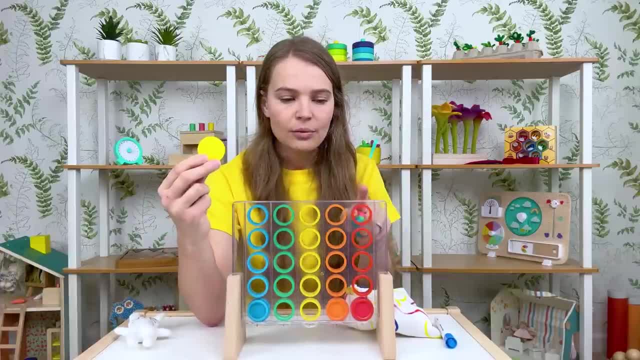 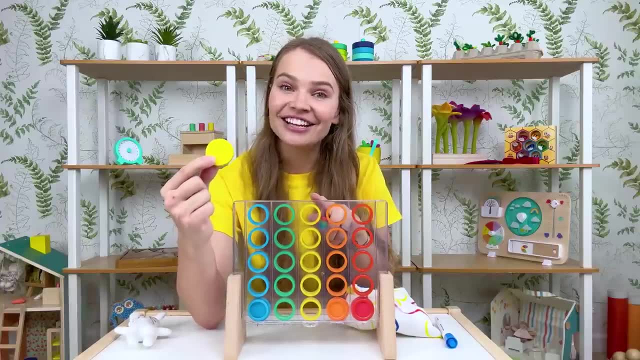 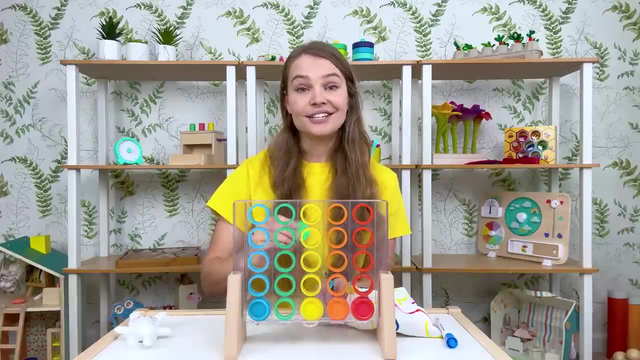 should we put the yellow circle? Hmm, We already have one in the red, orange, yellow. Oh, this is yellow And this is yellow. Let's put it in. I'll help you. Ready In, Now it's my turn And I've got a green one. Where should I put the green circle? I've got 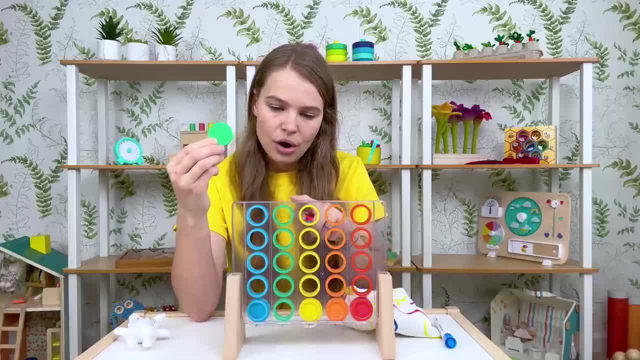 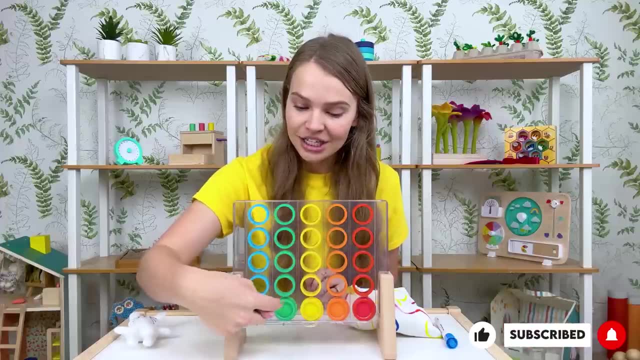 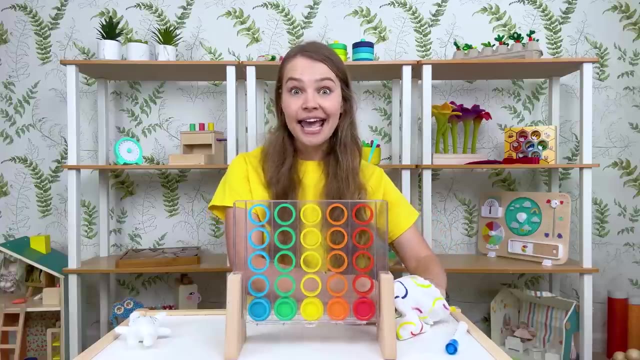 red, orange, yellow. Oh, look, right here in the green. I'll put it in: All right, Now we've got each colored circle in each of the spots. We can keep filling it up together And then at the end. 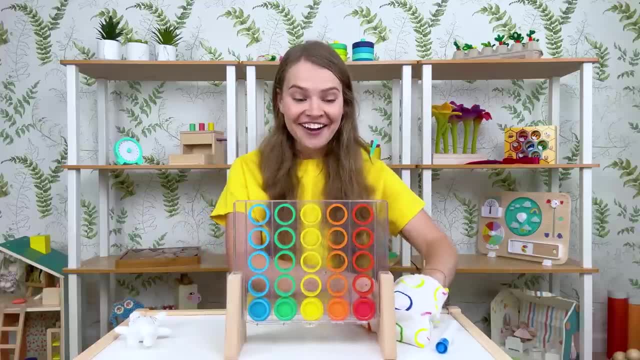 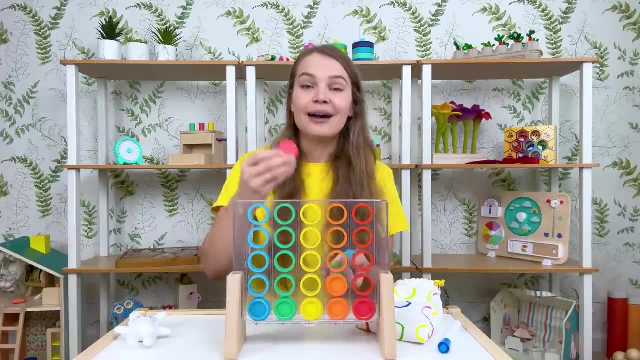 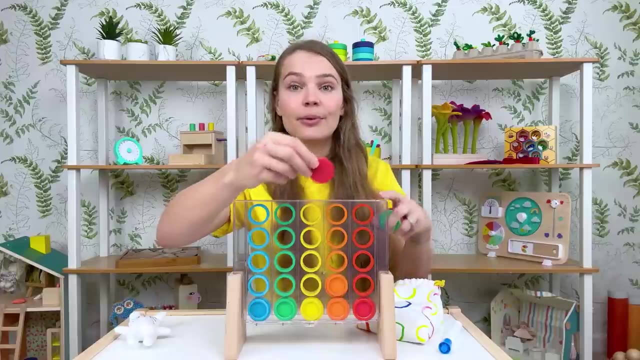 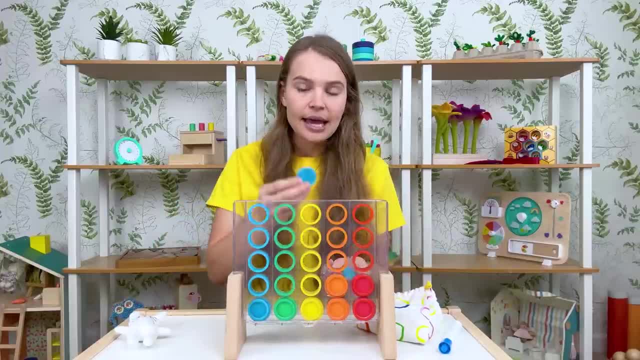 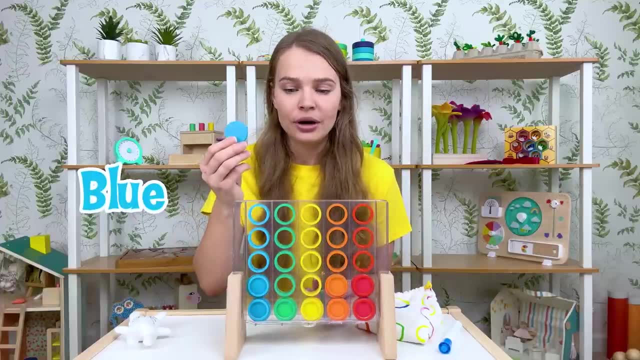 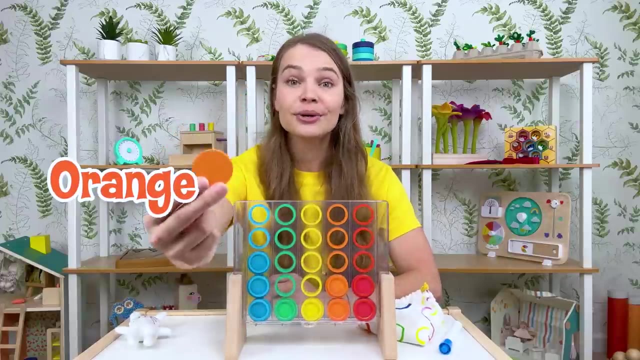 you. I'll put it in for you. Here we go, Got more blue. Hmm, In the blue I've got another blue. We just put a blue one in. It was right in here. Here we go. I got an orange one And it's your turn. Where do you want to put the orange circle? 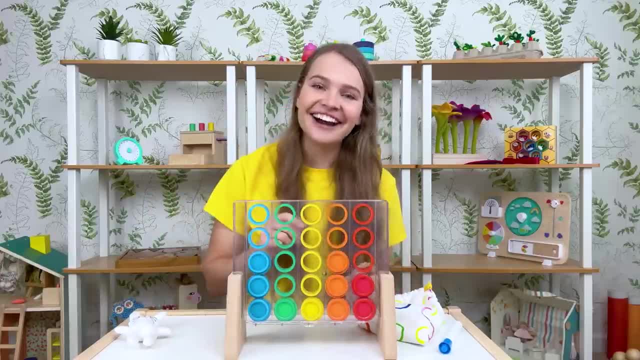 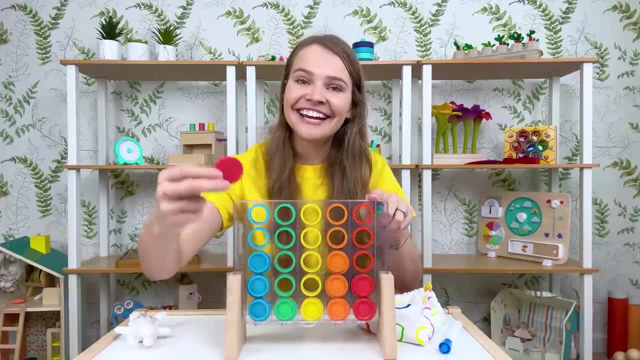 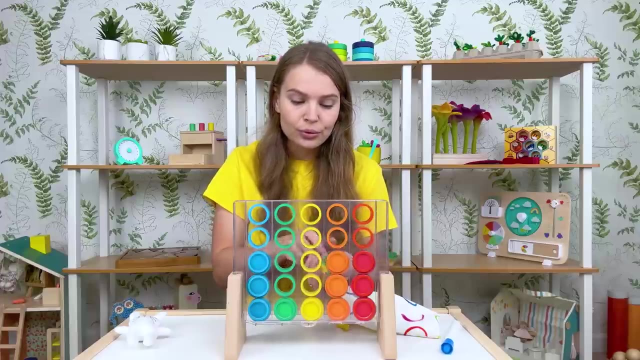 In here in the orange. I'll put it in for you. Here you go. How about a red circle? Where should we go Right here? Great, Thank you for helping me. Let's see what other colors I've got in my bag. Ooh, How about a yellow circle? Where should we put it? 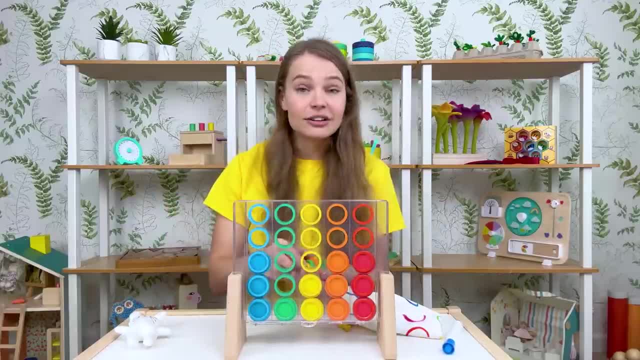 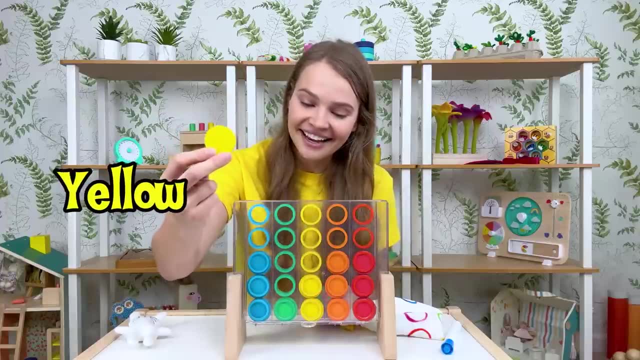 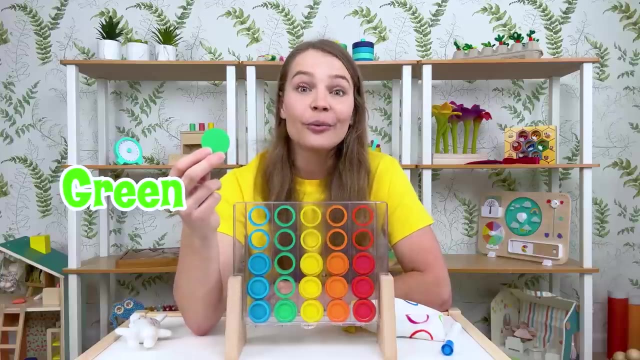 In here. I'll put it in. You're a great friend to play with And I like taking turns to put our circles in. Thank you for playing with me. How about this yellow one In here? Yeah, Good thinking. Okay, How about this green one? It's your turn. Where do you want to put it in In here, I'll. 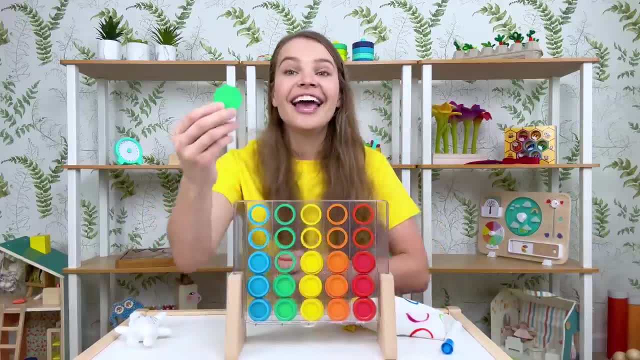 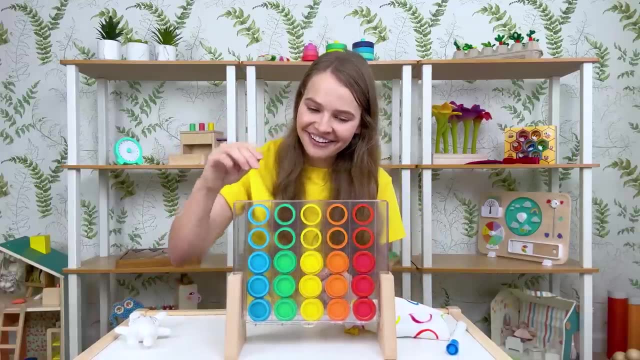 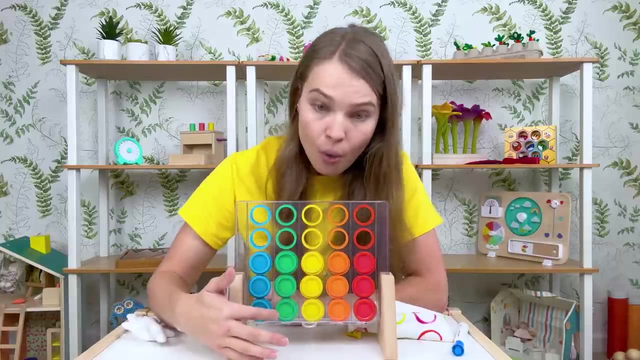 put it in for you. Here you go. I got, oh, another green one. Where should we put it In the green? I'll put it in for you. Wow, Now we've got one, two, three blue circles. One, two. 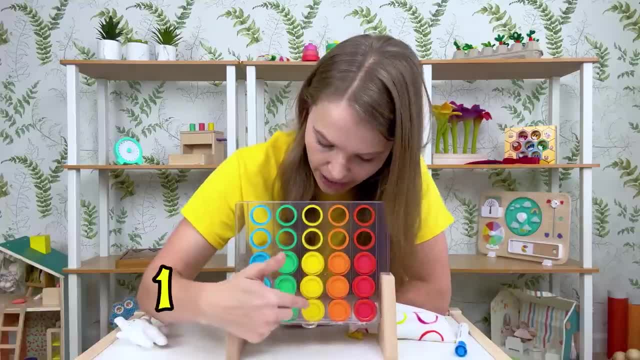 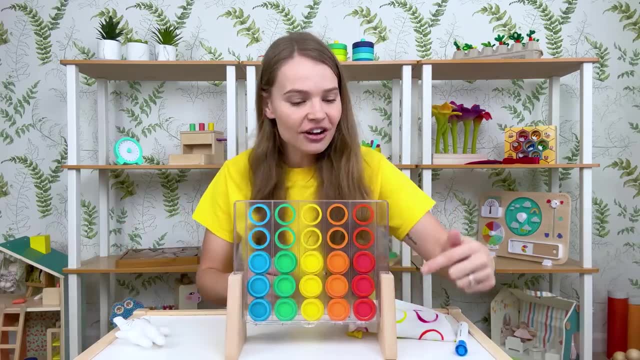 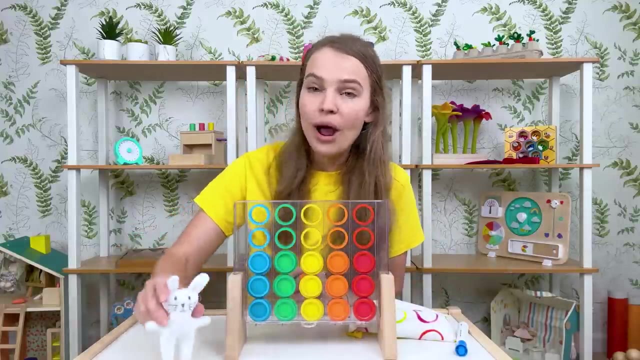 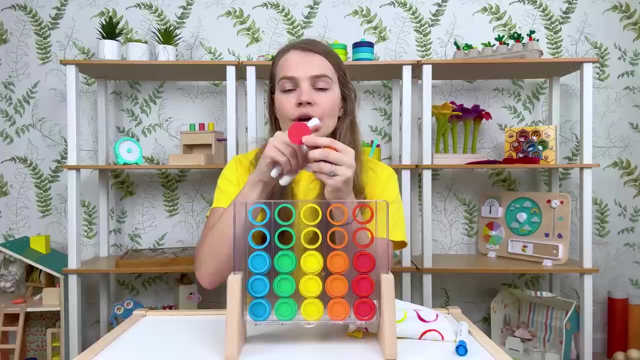 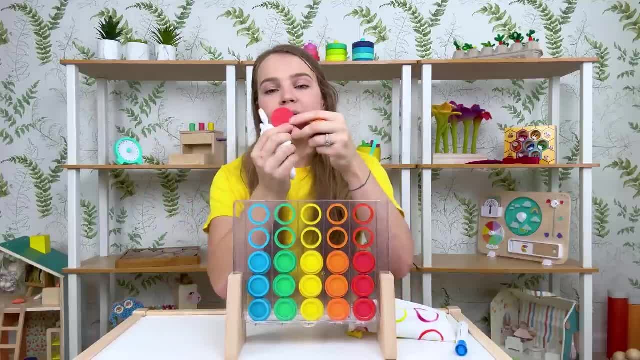 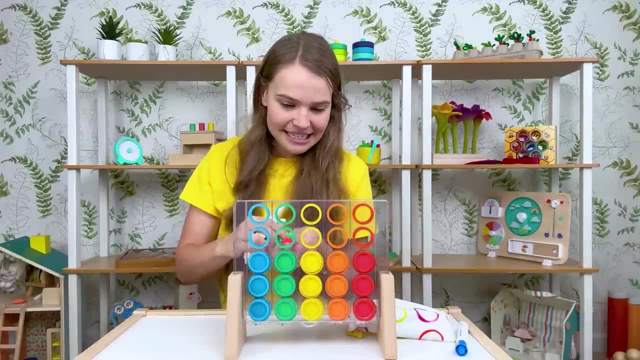 and around. That's right, And it's all the same way, Kind of like wheels of a car: Drive, drive. All right, Let's put the rest of our circles in. I've got a green one, Bunny, do you want to put? 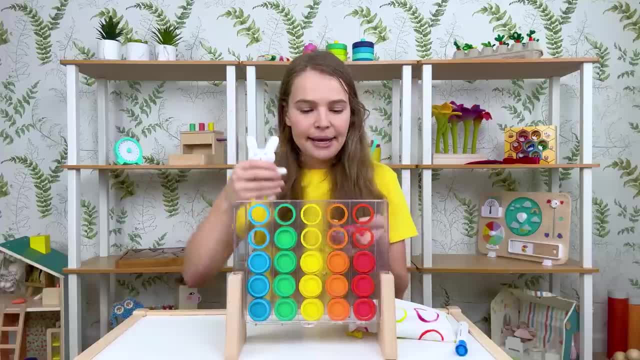 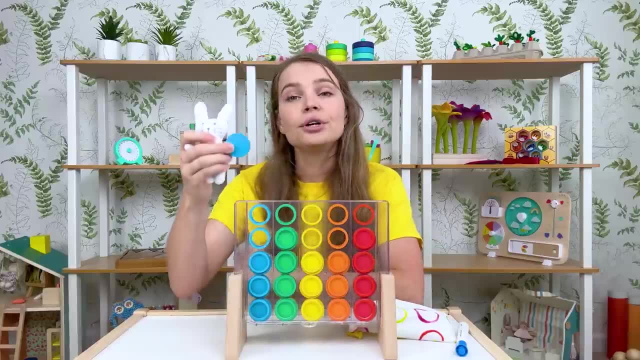 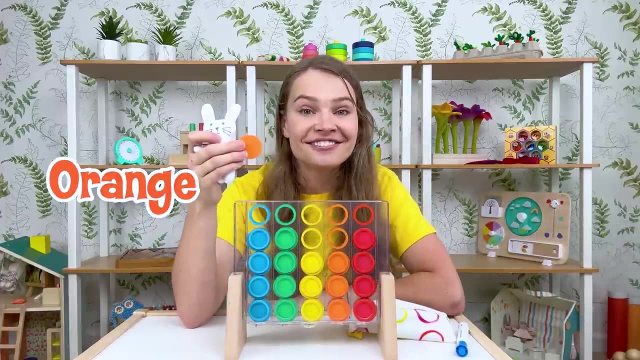 it in. Oh, I'd love to Hop, hop, hop in. How about this red one, Bunny? Hop, hop, hop in. Bunny, you're good at finding your colors. What about blue one? Where should the blue one go In? the blue, All right. How about this orange? 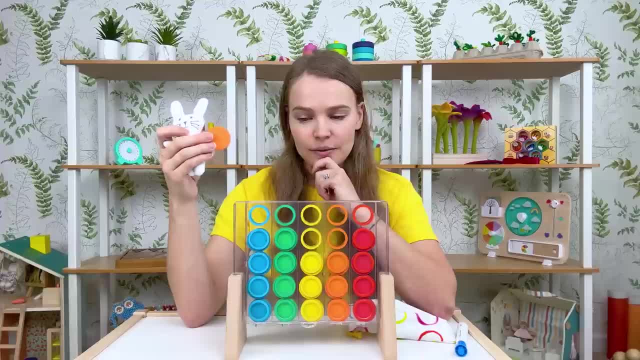 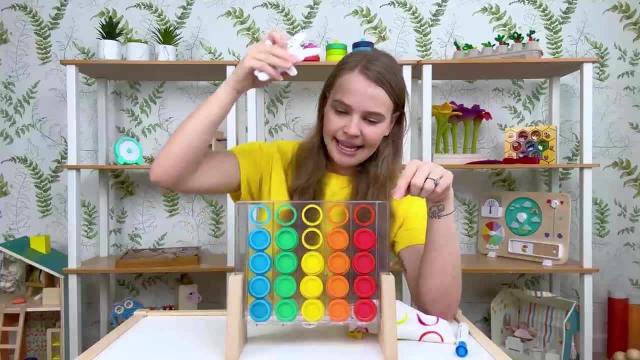 one. Will you help the bunny put it in? Let's see Where should we put it. There's yellow, but that's not orange. Here's orange. Here we go In. Let's get more circles out, All right. 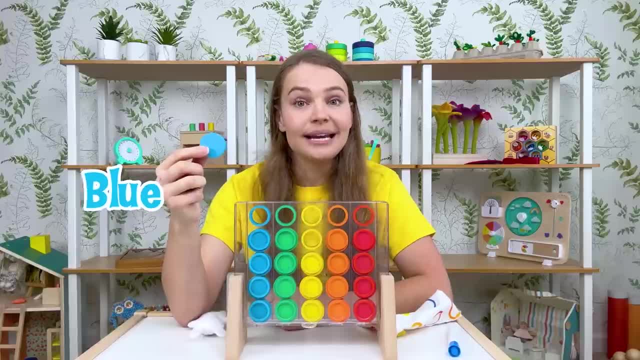 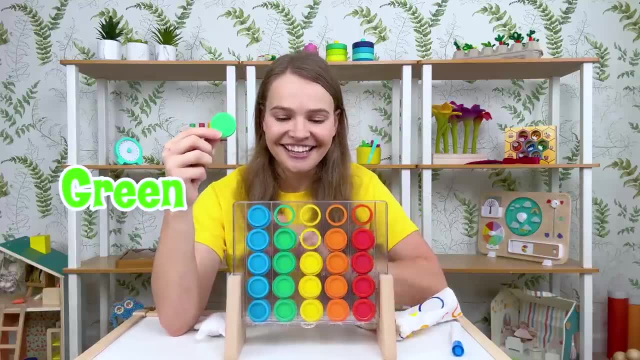 Here's a blue one, And it's your turn. Where would you like to put it in In the blue? Here we go. I've got a green one. Where should we put it In the green? Here we go. I've got a yellow one. 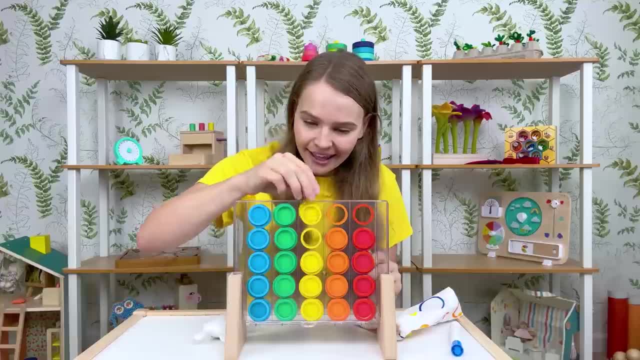 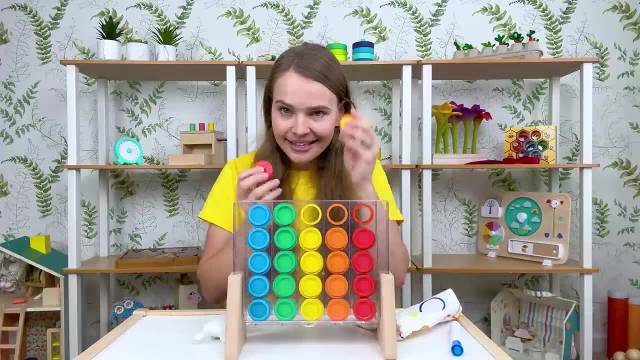 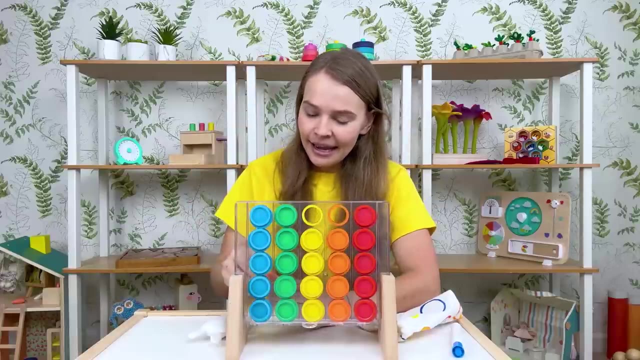 Where should we put the yellow In the yellow In? you go circle Oopsies. Oh, I dropped that one. Come back, orange circle. We're still playing silly circle. How about this red one In here? What about this orange circle? 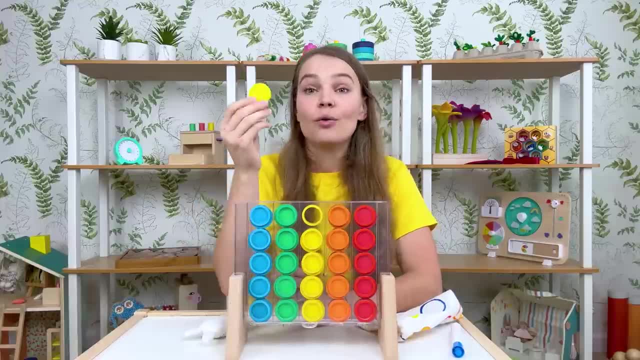 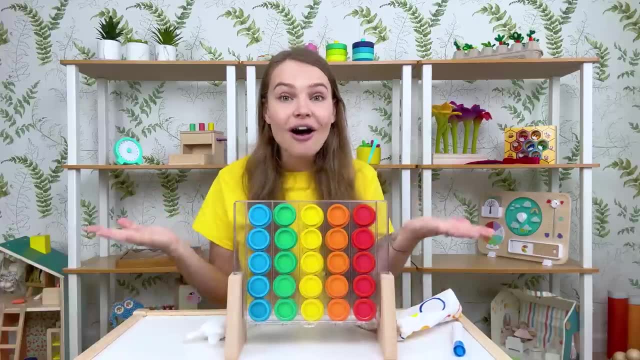 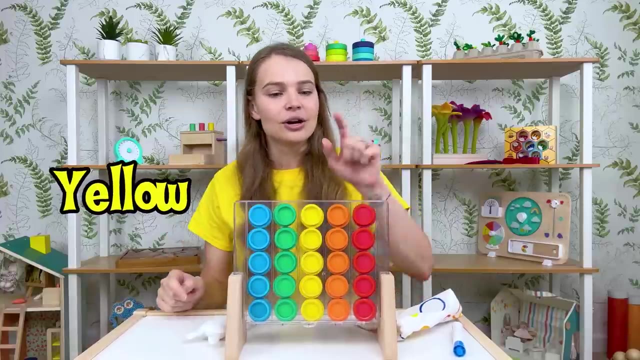 In the orange. Here we go. What about this yellow circle Right here? Wow, look at our game. It's all filled up with all of the colors. There are blue circles, green circles, yellow circles, orange circles and red circles. 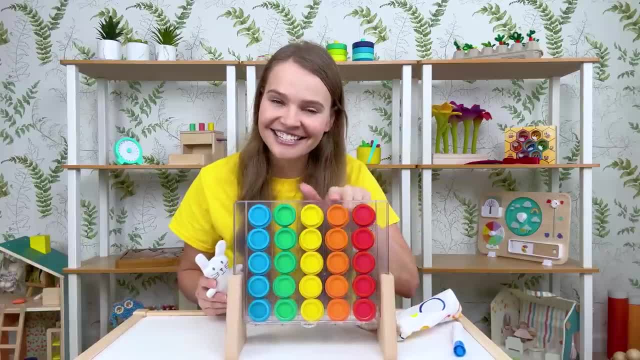 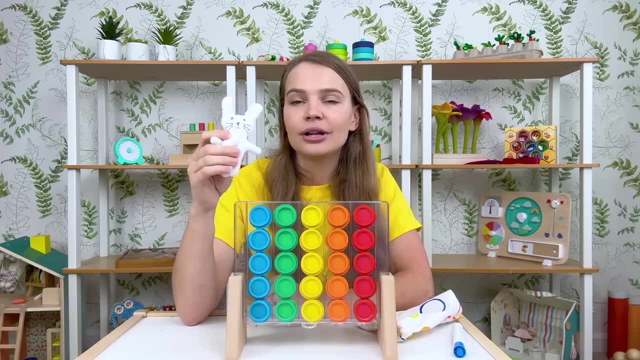 You're really good at your colors and you know your shapes, Like this circle. Wow, says the bunny, Hop, hop, hop, hop hop. I love all these. I love all these colors And I'm really glad to know what a circle is. 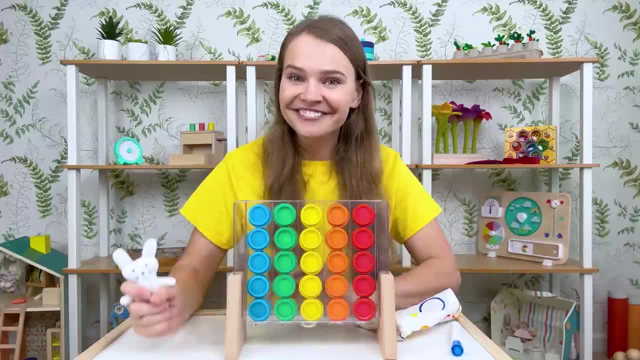 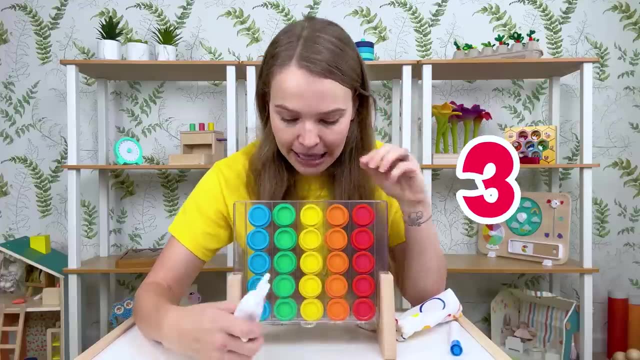 Now let's push this button over and they'll all fall down. You ready, It might be loud, Okay, ready, I'll count to three. One, two, three, Slide it over. bunny Whoop, Oh wow, and they all fell down. 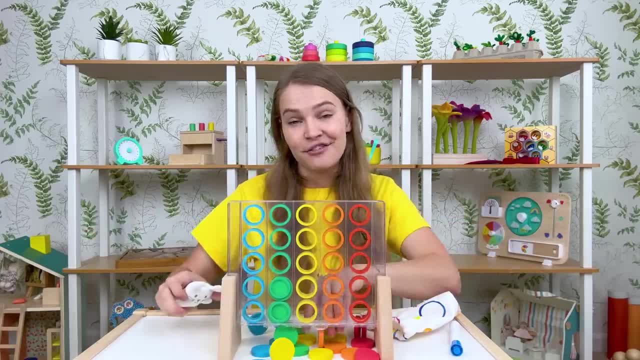 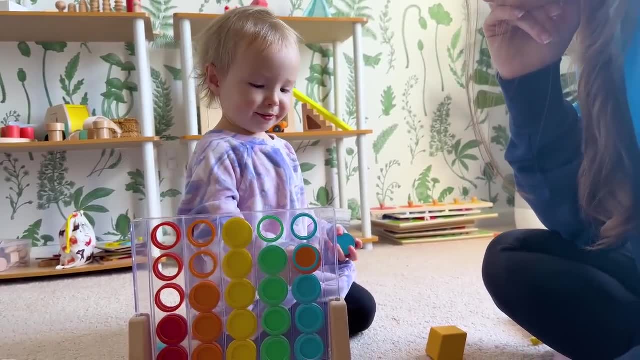 They all fell down. Silly game. This is a fun game with circles. What's your favorite shape? Heart, Heart, You like circles. No, I like circles. What Did you get an orange one in there? All right, you can press the button. 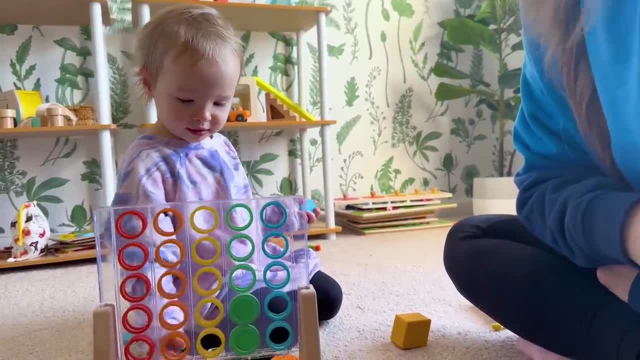 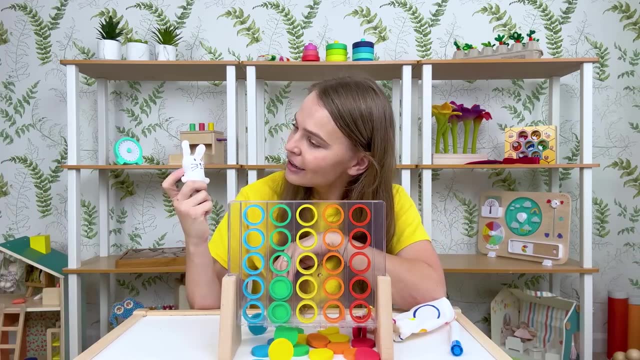 Whee, And they all come crashing down. Now, bunny, now that you know what a circle is and we put so many in, do you wanna draw a circle together? Oh, I'd love to draw some circles together. All right, let's do it. 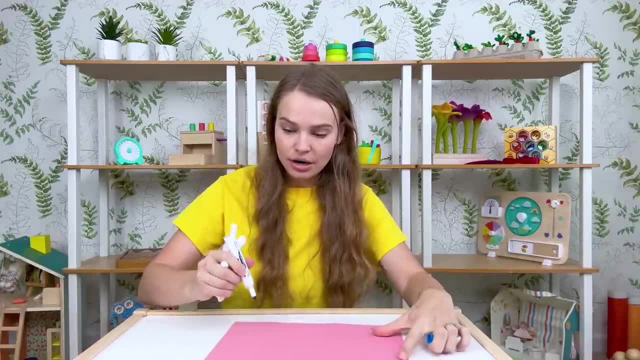 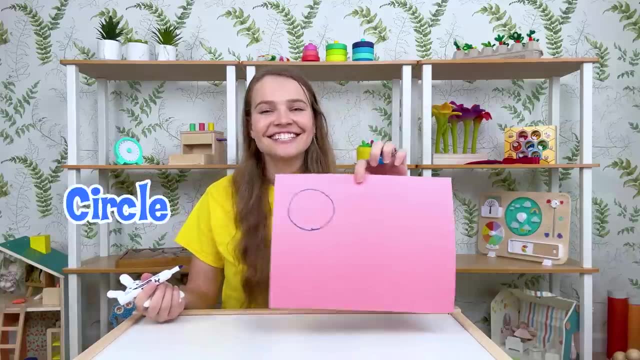 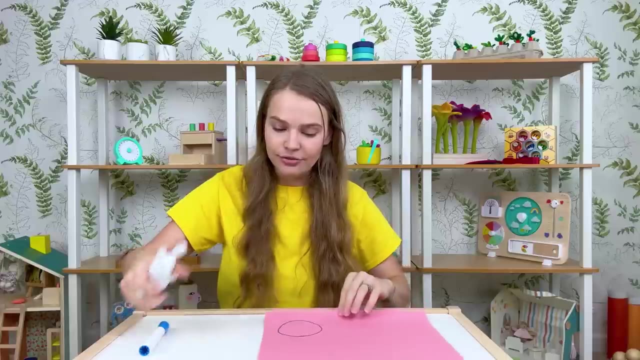 Let's draw a circle together with bunny. To draw a circle, you go, oh wow, Round and come back to the end. Circle around and back, Circle. here you go, bunny, Now you've got your first shape and you can hop in it. 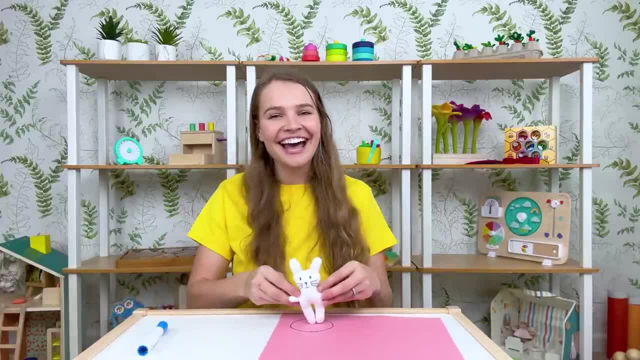 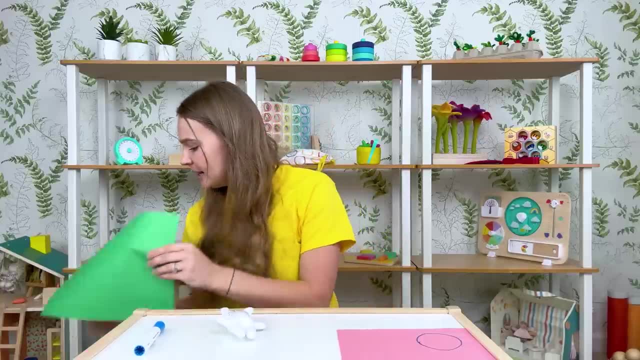 Hop in the circle, Hop, hop, hop, hop. You can also cut out fun shapes. if you ask your grownup for help, You can get a piece of paper and scissors, but make sure your grownup touches and uses the scissors. 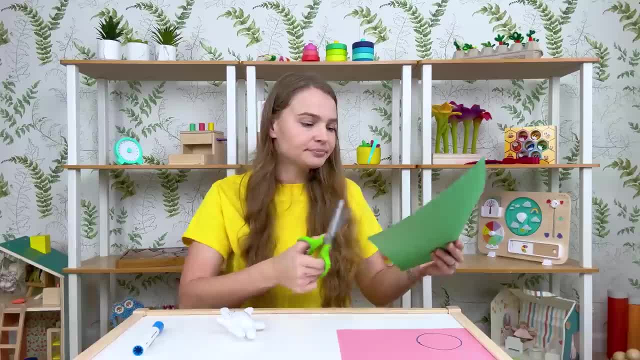 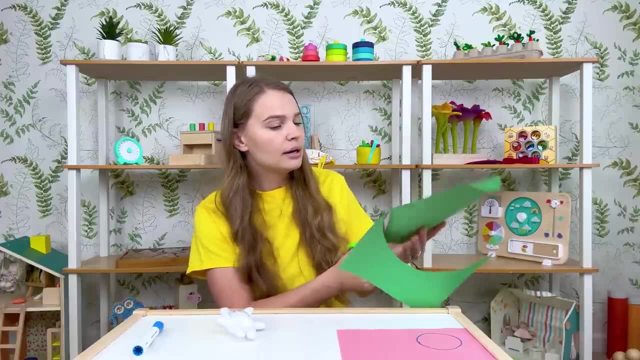 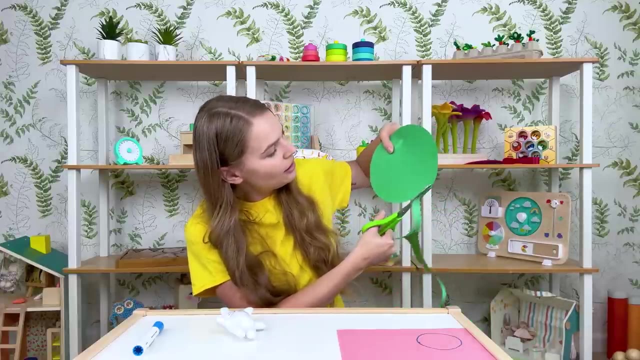 because they are sharp. We don't wanna touch sharp things, They're only for grownups. But you cut it around. You would ask your grownup to cut around, Cut around. Here we go, Cut around And we've got a circle. 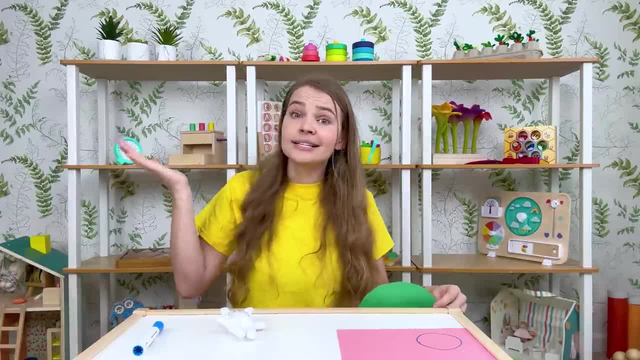 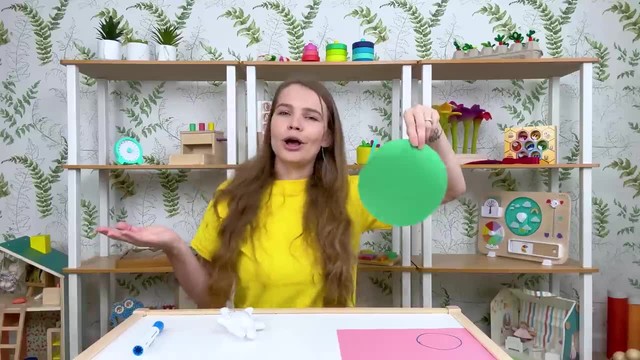 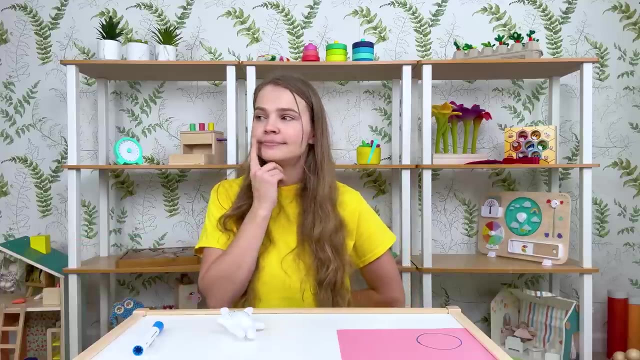 Oh, where is circle? Where is circle? Here? I am, here, I am, Here I am. How are you today, sir? Very well, I thank you. Run away, run away, Silly circle. where did it go? 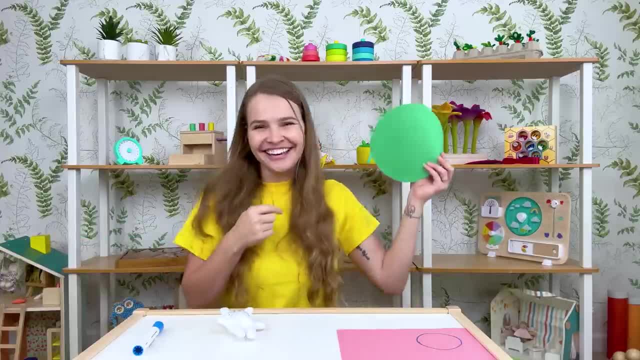 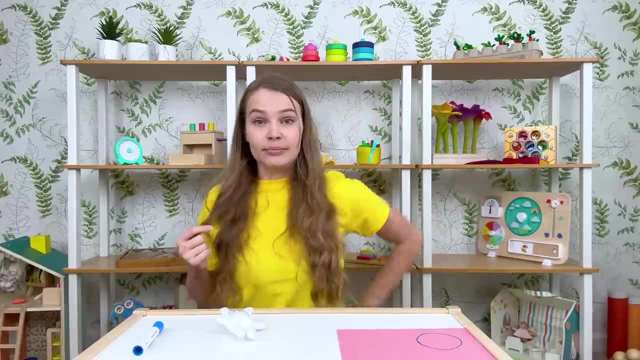 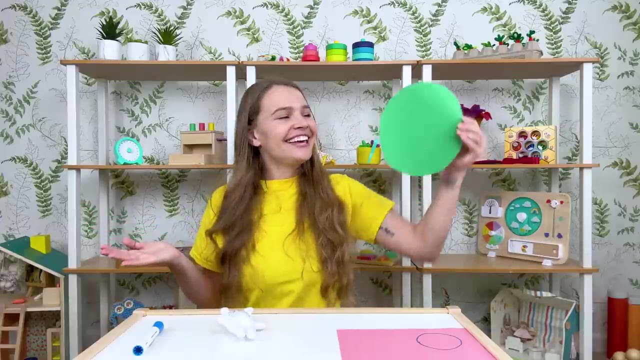 Hmm, behind my back, Here it is. Oh, where did it go? Here it is: Oh, where is circle? Where is circle? Here I am, here I am. How are you today, Sir? very well, I thank you. 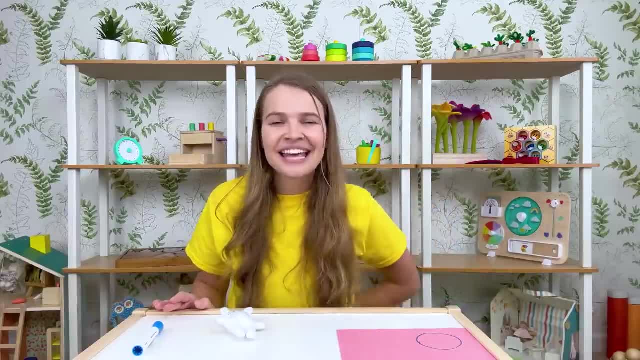 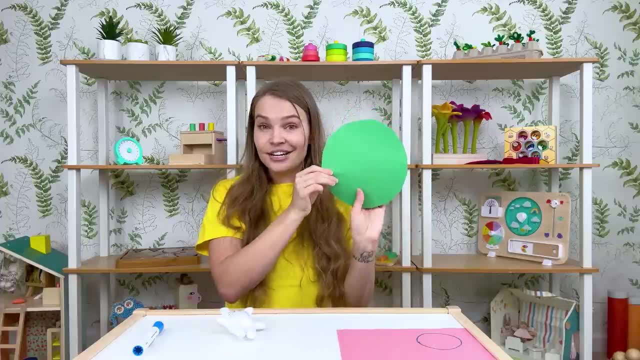 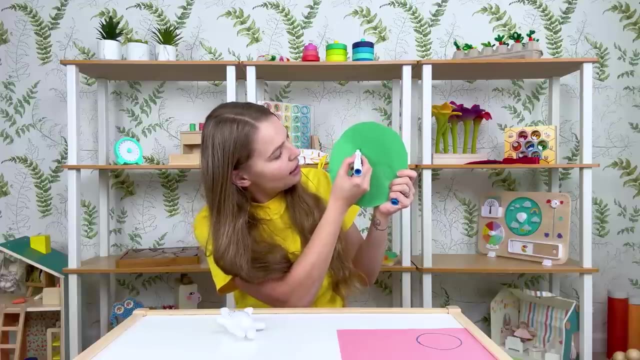 Run away, run away, Silly circle. You can find circles anywhere. If you look around and you see something round, it looks like a circle And we can draw a little happy face on this circle. to make it a happy face, Here's a one eye. 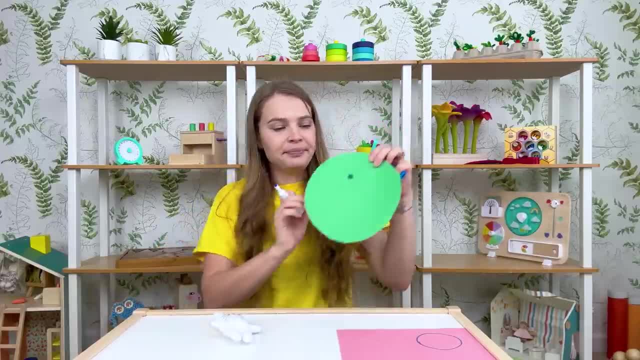 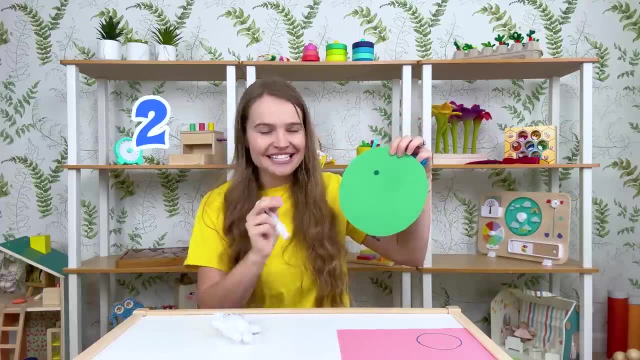 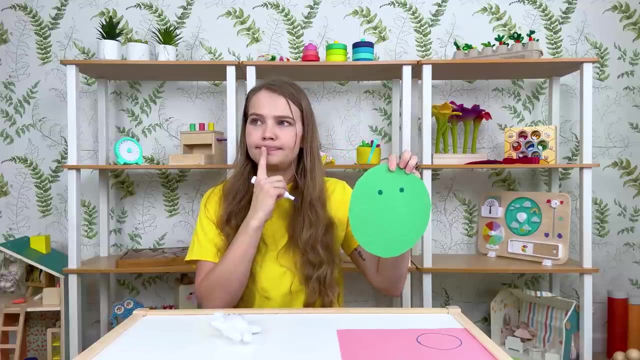 Let me set this down and draw one eye. Wait a minute, how many eyes do we have? One, Two, Two eyes. Let me draw another one, then Two. Let's see what else do we have on our face? Hmm, 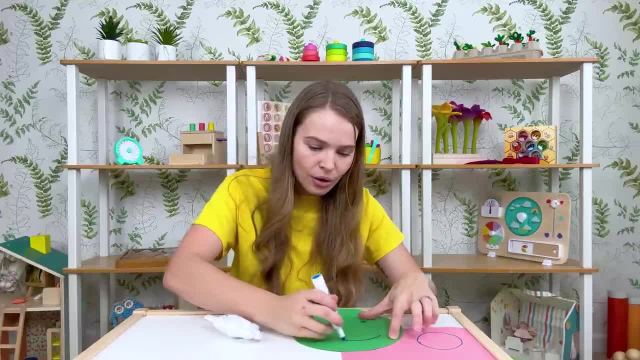 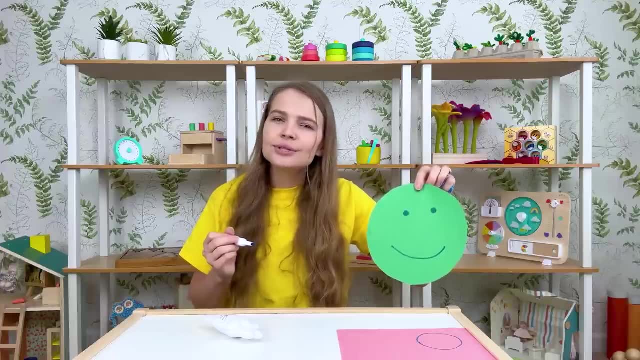 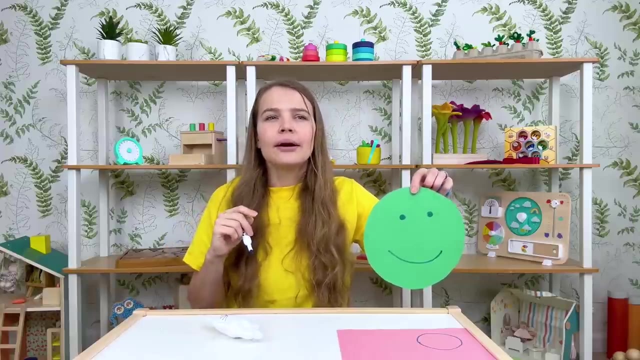 Mouth. Let's draw a mouth, One mouth. And what about something we smell with? What do we use to smell Ear? No, that's how we hear things with our ear. How do we smell things With our Nose? 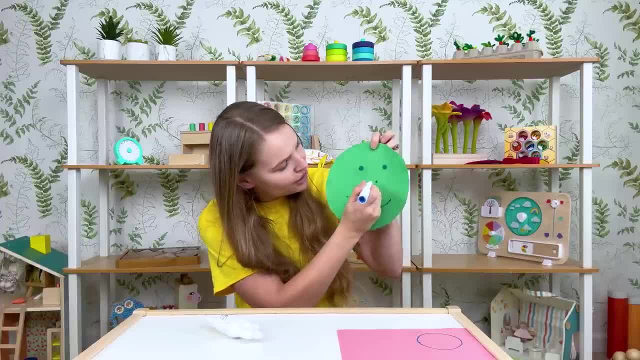 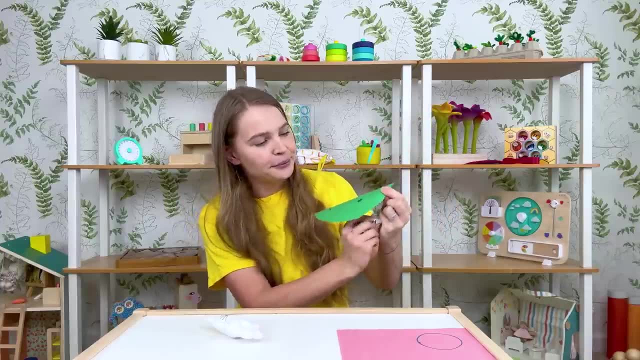 Let's draw a little nose. We'll do that. Beep boop, A little nose. Circle says: hello, Hi circle, happy face, Nice to meet you. And the bunny says: oh, I love circles. now They go around and around. 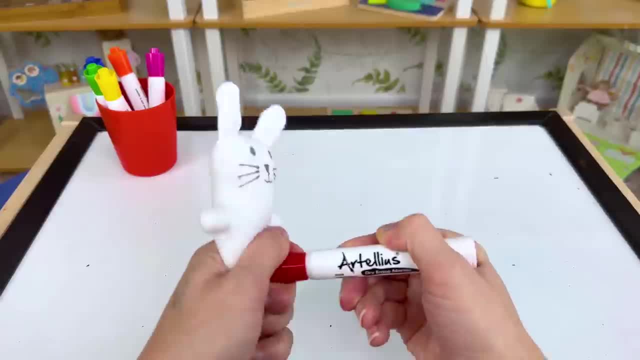 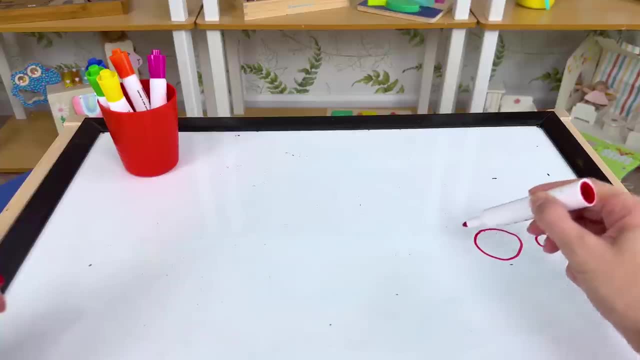 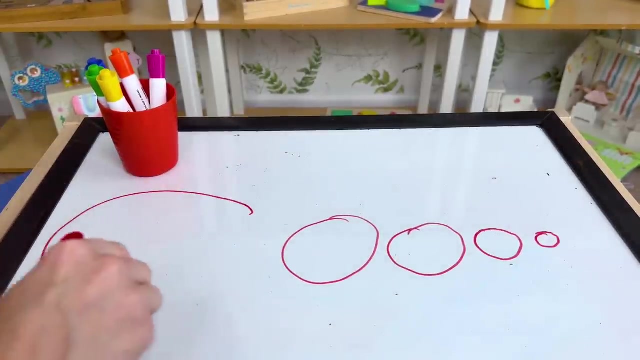 That's right, bunny. Now let's draw some circles for bunny. Let's do a little circle, a little bit bigger, a little bit bigger, A little bit bigger, Whoop And a really big circle. Oh, I love these circles. 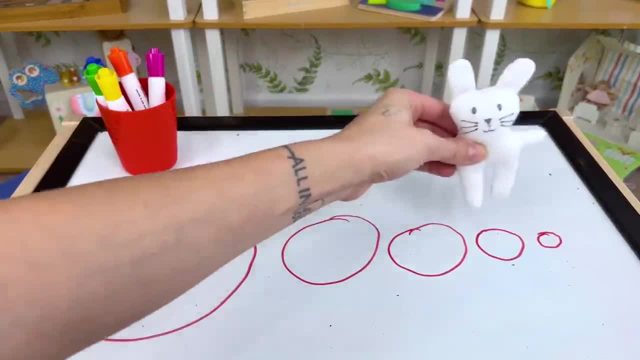 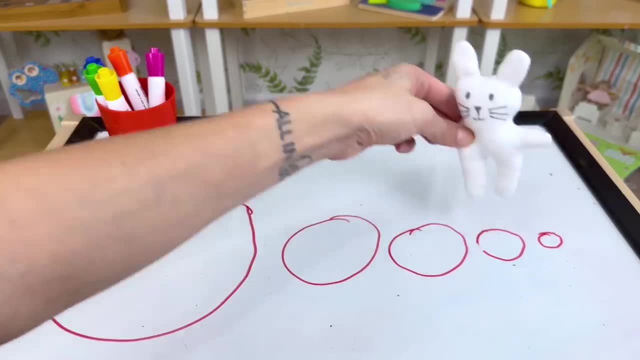 Hop in the big circle. Hop in another circle. Hop, hop, hop, Hop, hop, hop. Hopping through the circles. Hopping through the circles, Hop, hop, hop. I like my circles. Wow, bunny, we're so happy you like your circles. 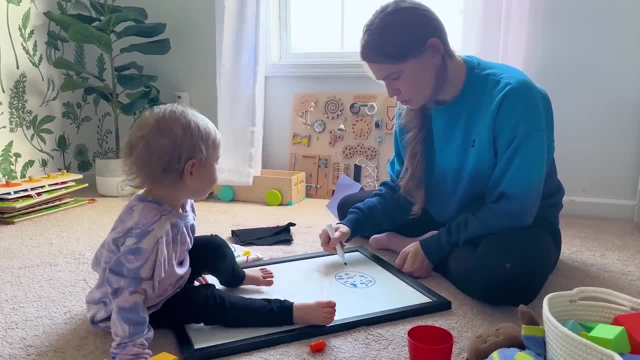 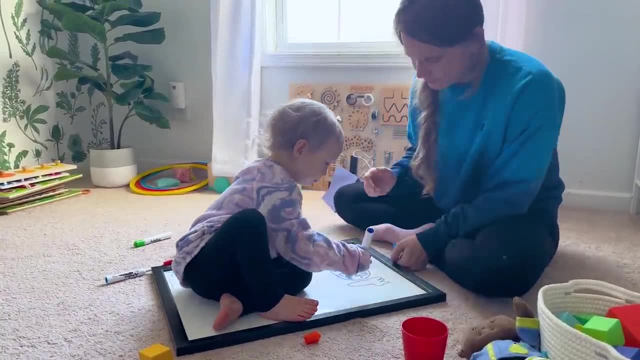 Bye, bunny. And here's some blackberries too. And here's your spoon. Eat up And a fork. Here's a fork. Enjoy Poop And grab a fork. Poop, poop, Yum, yum, yum. 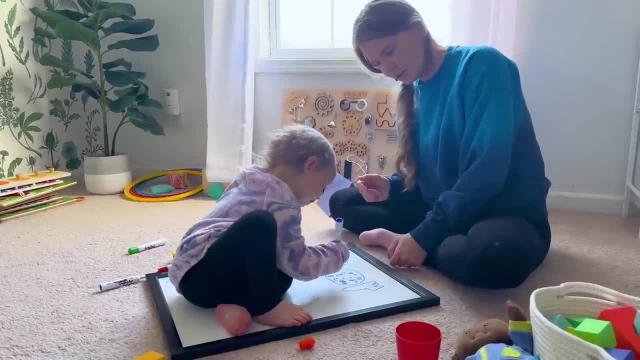 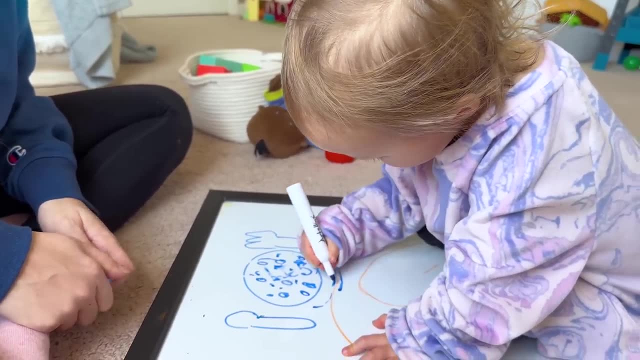 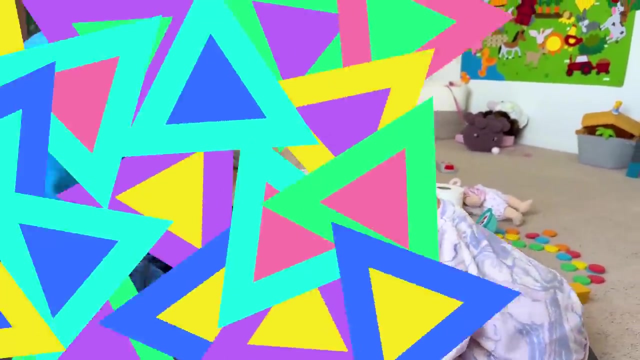 And then look It's in there. Oh yeah, What about some birds and some seeds? But I have a bee and I want to make two birds. Triangles are really great shapes too, And they have fun. They have three corners and three sides. 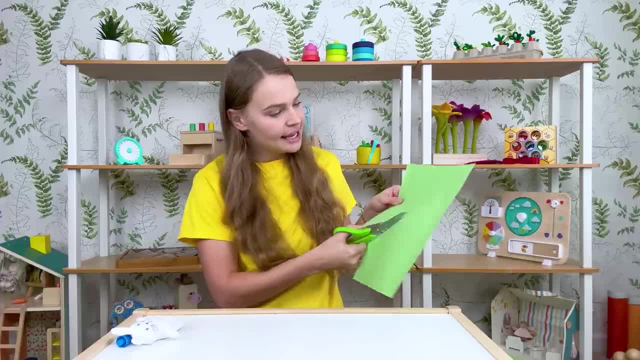 And you can ask your grownup for help to cut a triangle for you. Oops, this one's a little wonky donkey. It's not a corner. What's going on? Let me cut it again. Sometimes I make mistakes, huh. Sometimes I don't do things right, but then I can go ahead and fix it. Here is a triangle. This triangle has one, two, three, four, five, six, seven, eight, nine, 10,, 11,, 12, 13,. 12, 13,. 14,, 15,, 16,, 17,, 18,, 19,, 20,, 21,, 22,, 23,, 24,, 25,, 26,, 27,, 28,, 29,, 30,, 31,, 32,, 33,. 32,, 33,, 34,, 34,, 35,, 36,, 37,, 38,, 38,, 39,, 40,, 41,, 42,, 41,, 42,, 42,, 42,, 43,, 42, 43,. 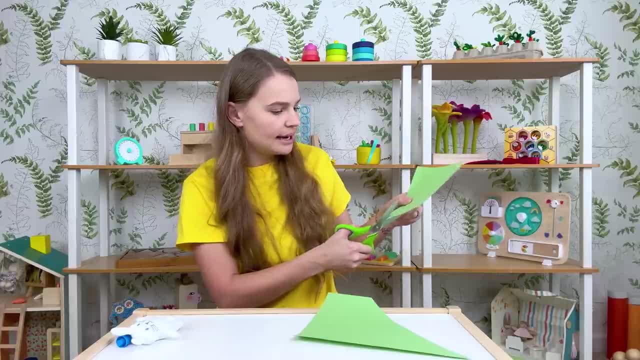 44,, 45,, 46,, 47,, 48,, 49,, 50.. Here is another one. It's not a triangle. What's going on? Let me cut it again. Sometimes I make mistakes, huh. Sometimes I don't do things right, but then I can go ahead and fix it. 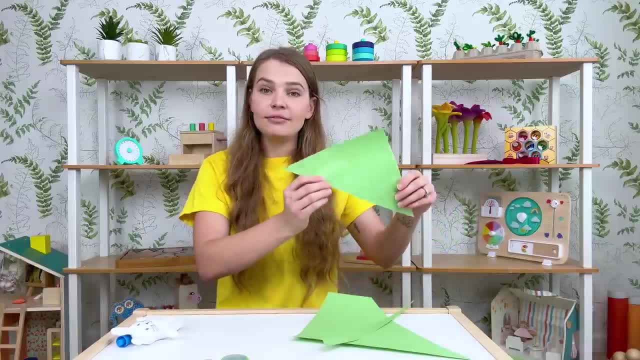 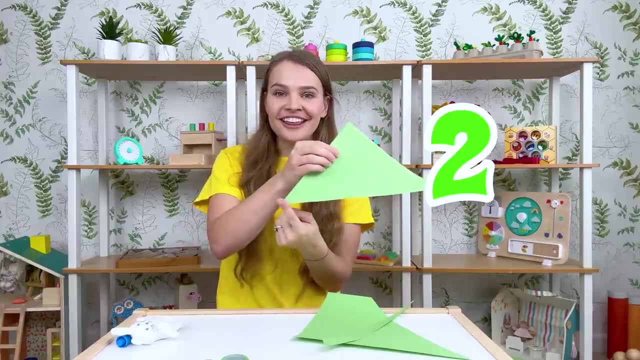 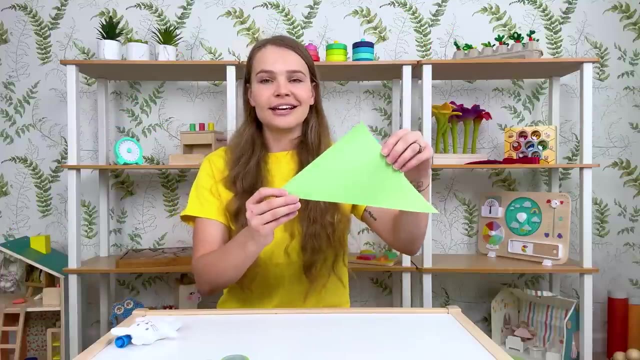 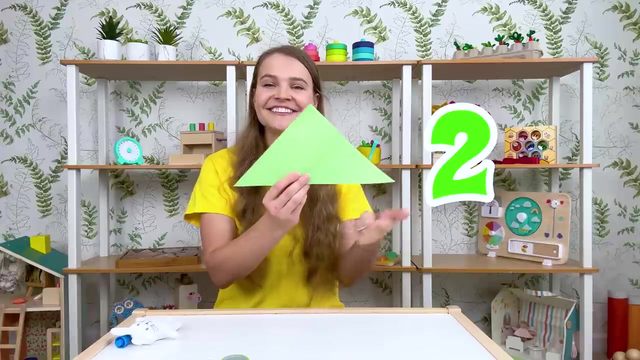 Here is a triangle. This triangle has one, two, three corners, and one, two, three sides. This triangle says: triangle triangle, look at me, my sides, one, two, three. you can do the corners too. triangle triangle, look at me. 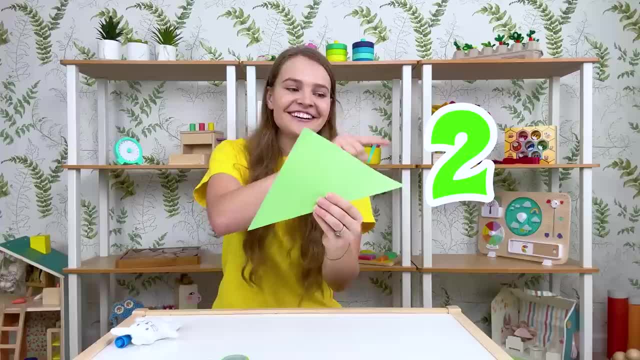 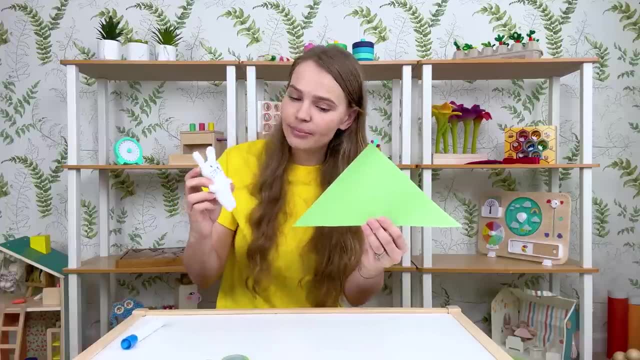 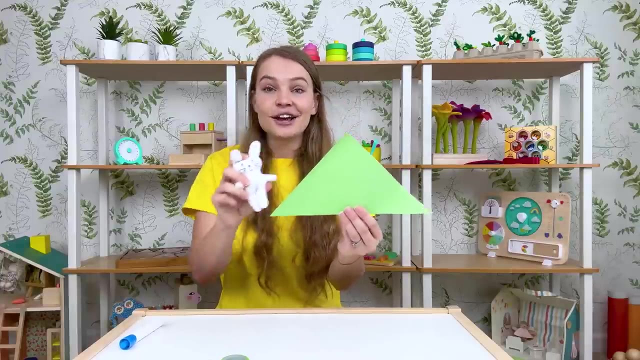 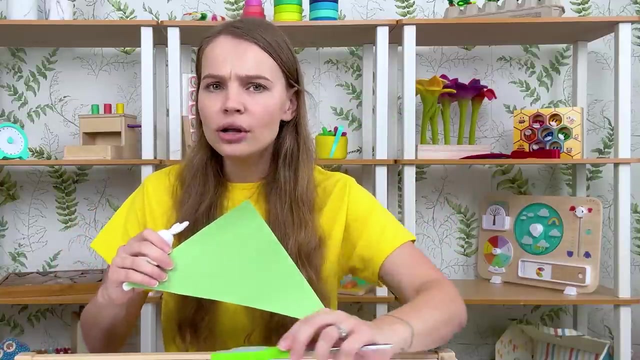 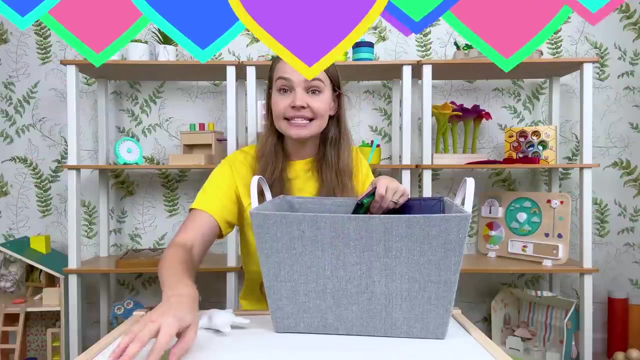 count my corners: one, two, three. a triangle has three corners. oh wow, I can hop on those corners. you sure can bunny. here's one, here is two, here is three. three corners for a triangle. I've got this triangle and I have some magnetic tiles, but they're all together. let me get them out. whoa hey, let's see if we 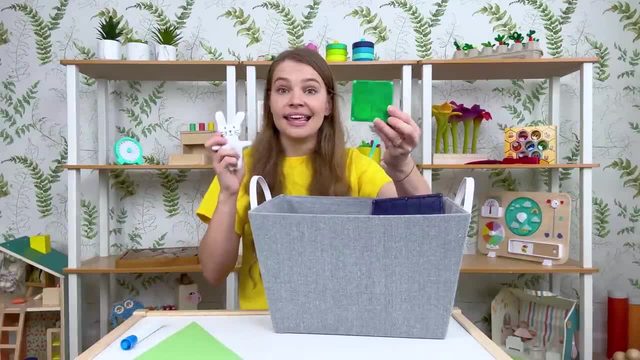 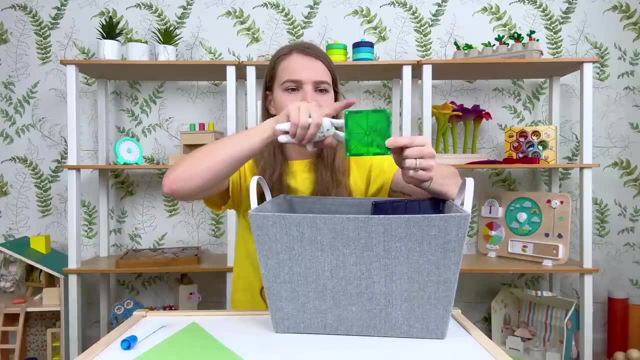 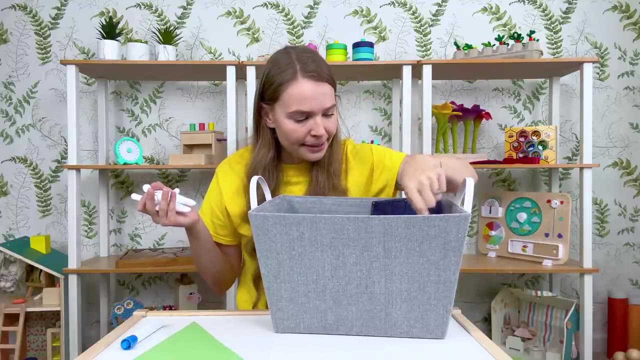 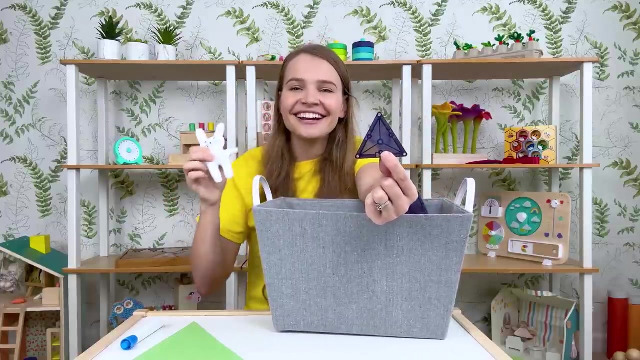 can help bunny find triangles. hmm, this has four corners- one, two, three, four- and four sides: one, two, three, four. that's a square. we're looking for triangles. we'll put that back. how about this one? is this a triangle? let's see one, two, three, three corners. that's a triangle. we'll put it. 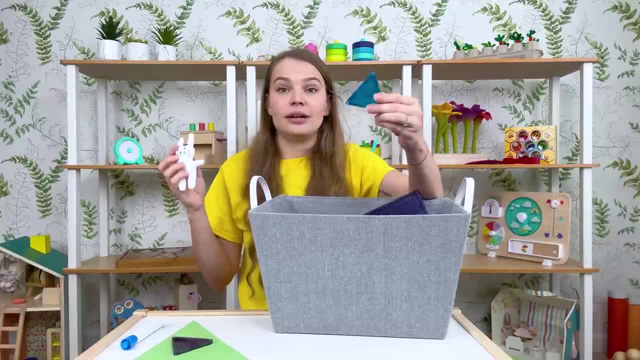 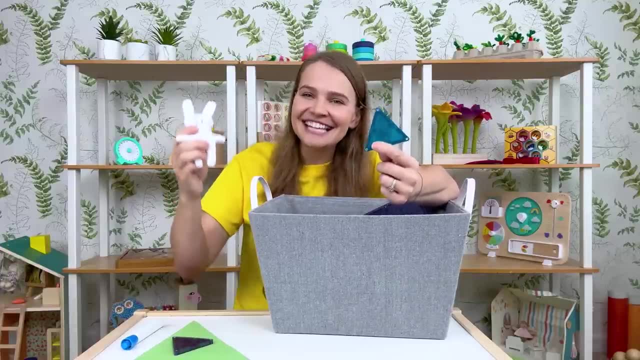 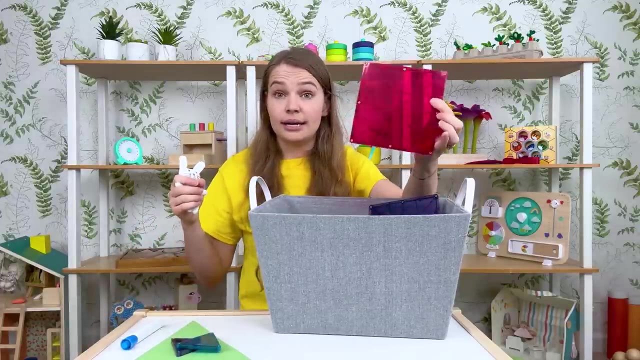 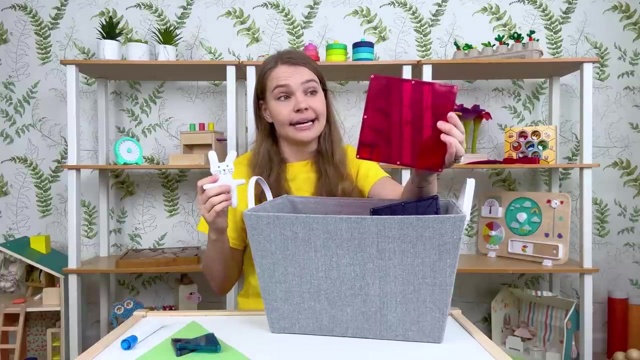 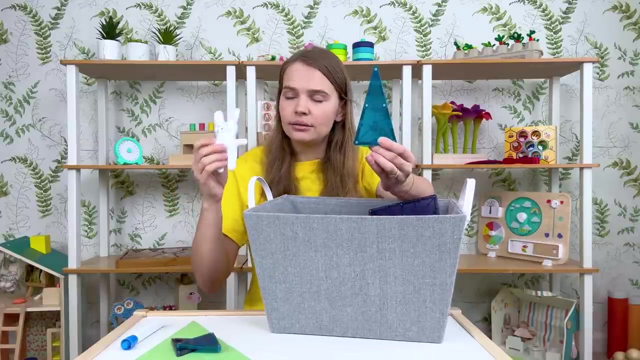 right here, let's see how about this one? is this a triangle? let's see one corner, two corners, three corners: that's a triangle. you know, bunny, this one is this a triangle? let's see one, two, three, four corners. I think that's a square. hmm, that's not a triangle. point it back. how about this one? let's. 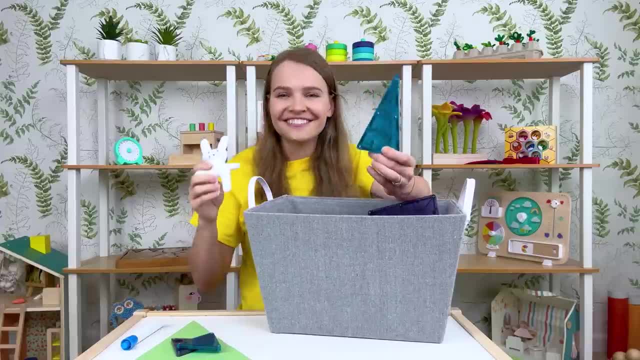 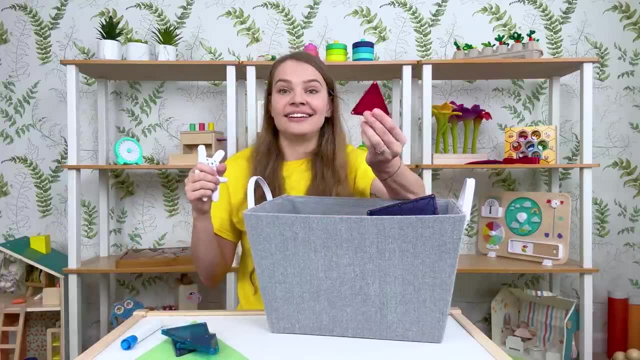 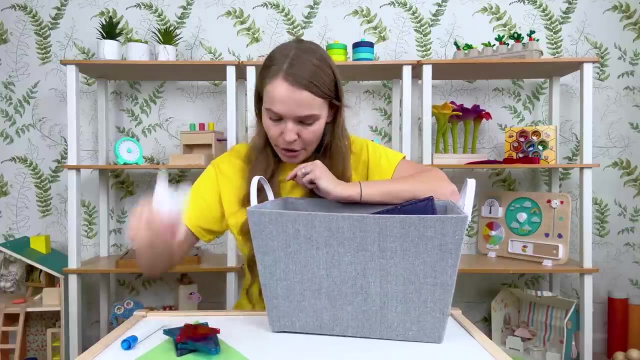 count the corners one, two, three, three corners. it's a triangle. here you go, buddy. how about this one? let's count the corners one, two, three. it's a triangle, it's a red triangle, thank you. there you go, bunny. let's see if we can find you. 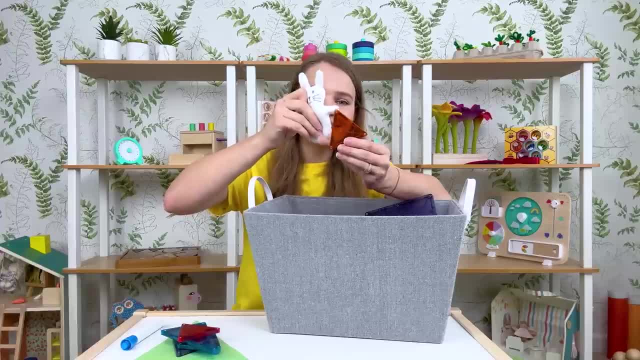 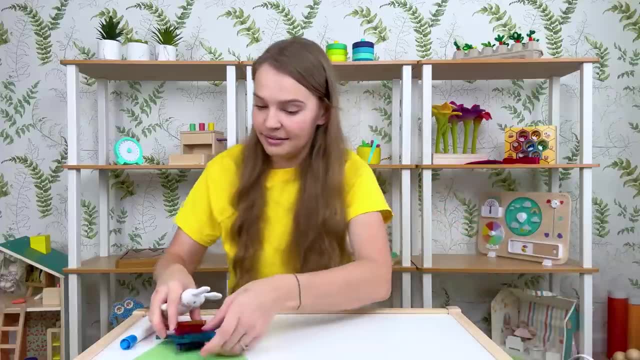 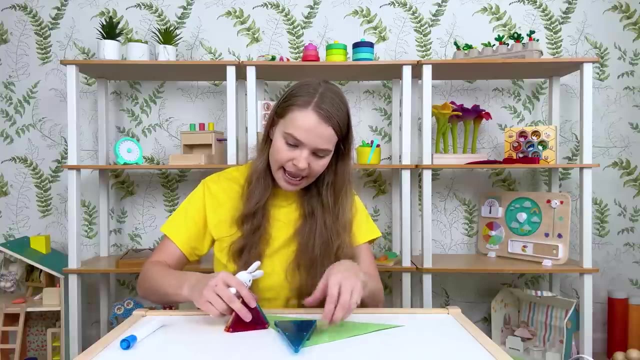 another one. how about this line? oh what, dude three, we've had a triangle for money. go by Paris. bunny, you did a great job looking for triangles. let's hope we can put these ones together for you. but I'm all in. this is a little pyramid, and 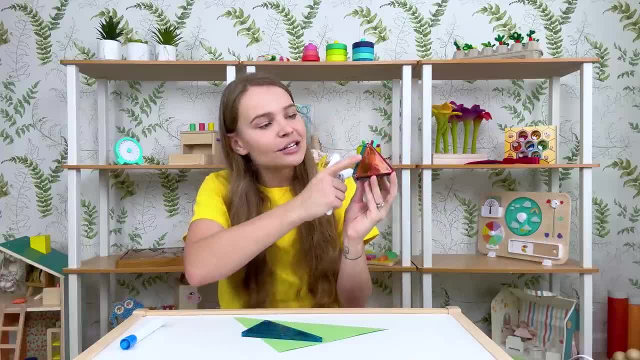 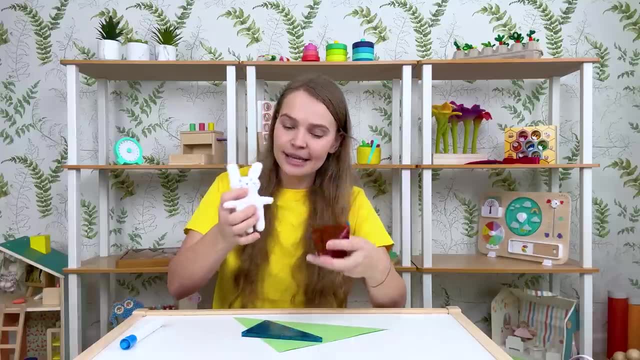 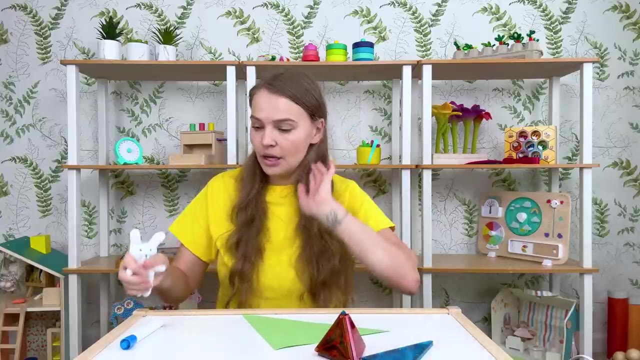 A pyramid is shaped like triangles. There's a triangle on this side, triangle on this side, triangle on this side, and all around there's triangles. Oh wow, says the bunny. Thank you for helping me learn about triangles, Of course. 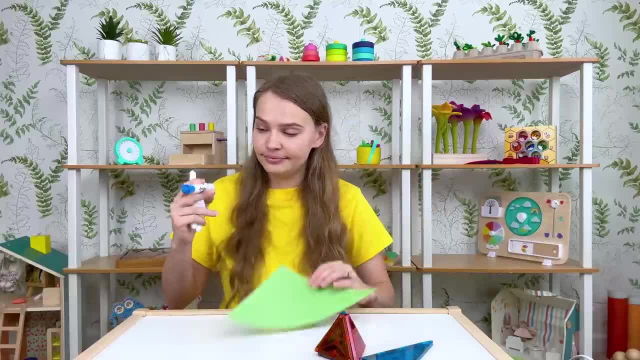 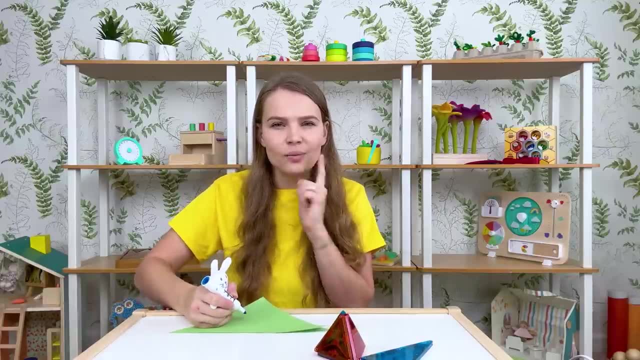 We can draw a happy face on this triangle and make it a happy triangle. You want to? Oh, I'd love to. Here we go, bunny, We'll draw. how many eyes was it? One, two, two eyes, two eyes. 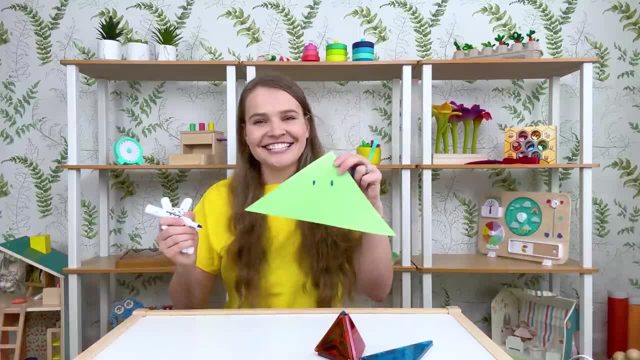 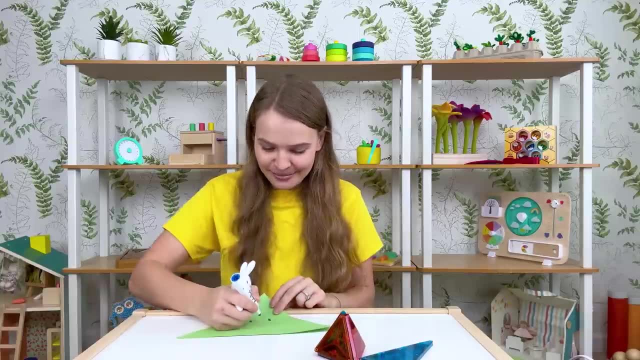 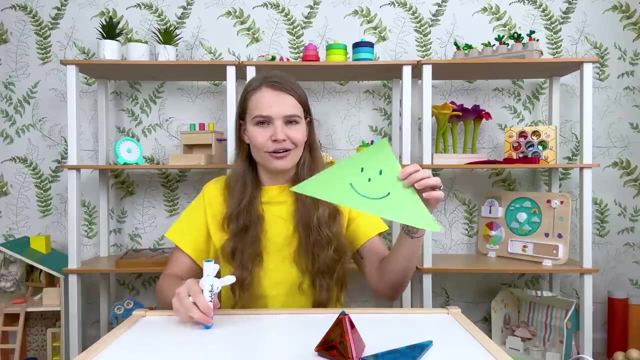 Good thinking. One eye, two eyes. And how about what was that in the middle? Nose, nose goes in the middle And mouth Hello, says the triangle. I'm a happy, happy triangle Oopsies. let me close this marker. 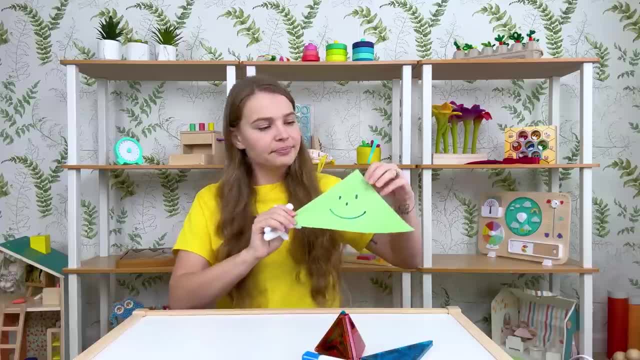 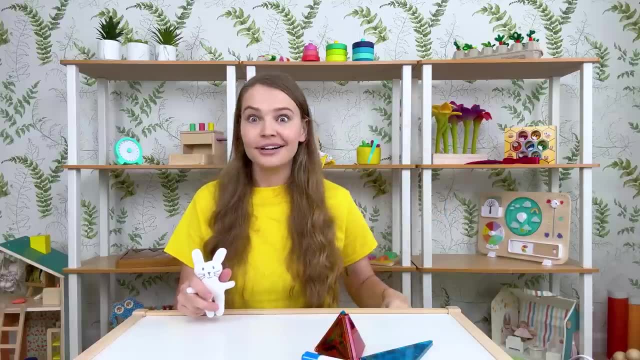 Marker, here you go. Gotta put the lids on so they don't dry out Marker's it. Marker, I meant to say triangle. Triangle says peek-a-boo. where did it go? Peek-a-boo triangle, peek-a-boo triangle. 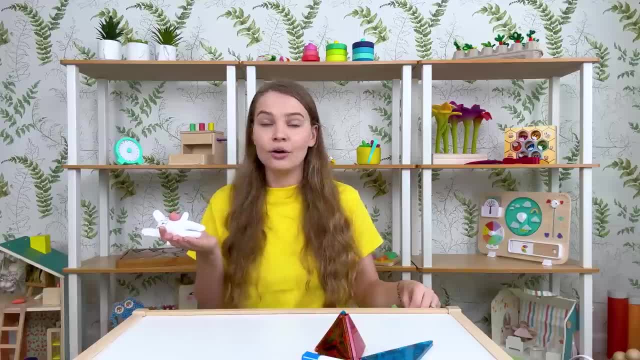 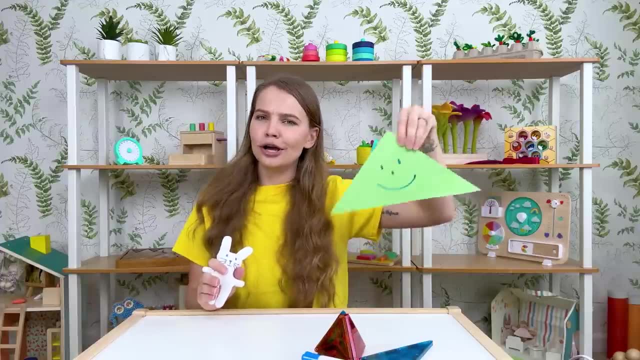 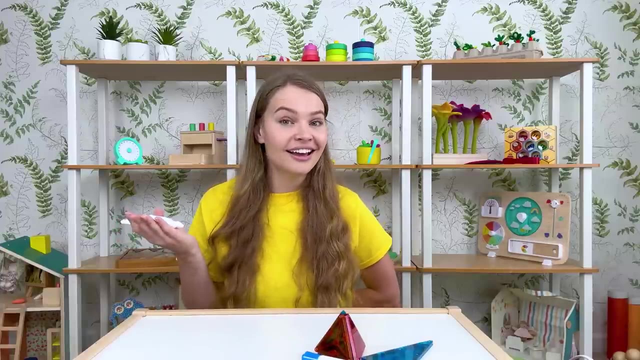 Where is triangle? Where is triangle? Here I am, here I am. How are you today, sir? Very well, I thank you. Run away, run away. Where did the triangle go? Behind my back, Behind my back, Oh hi, triangle. 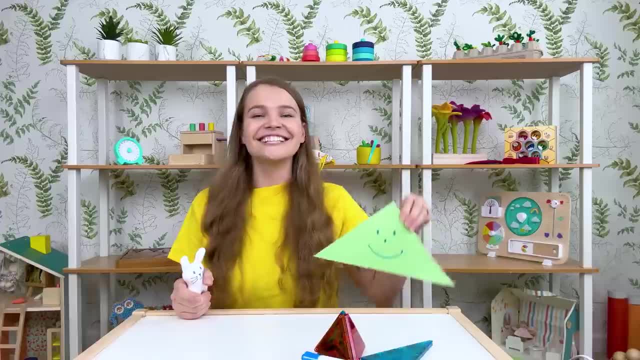 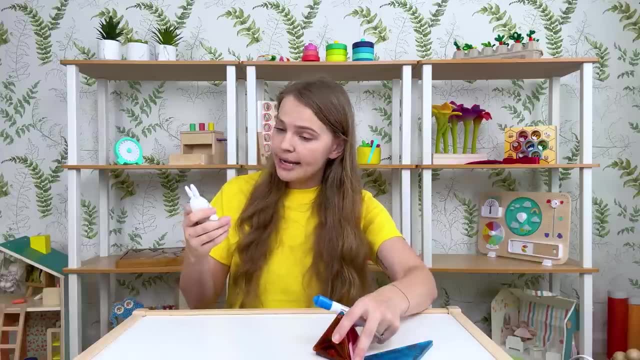 Triangle, says: peek-a-boo, peek-a-boo, silly triangle. Thank you for helping me learn about triangles. Bunny, do you wanna draw it on your piece of paper with your circle? That way you can have all your shapes together? Oh, I'd love to, says bunny. 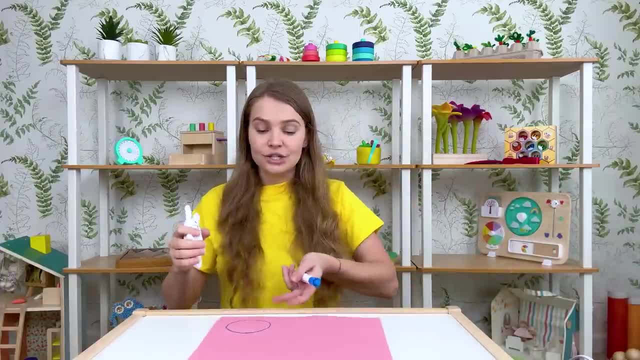 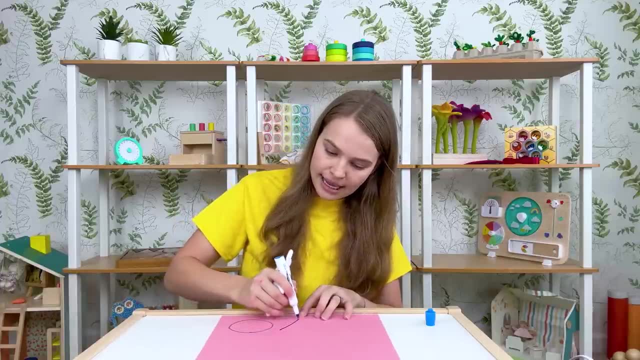 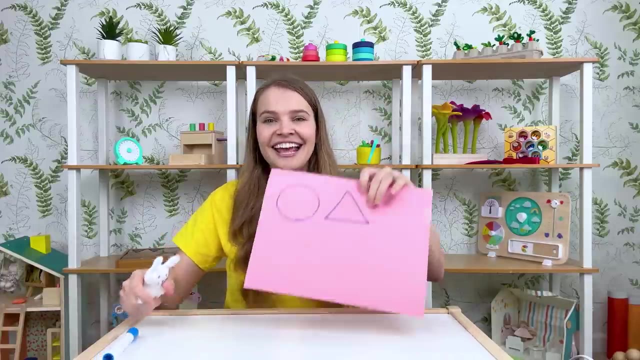 Here we go. I'll get you a piece of paper To draw a triangle. let's see, it has three sides, three corners. So we'll do one line, two line, three lines, and I'll put my lid back on. 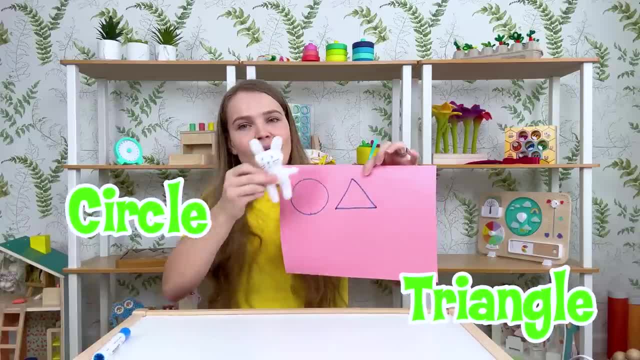 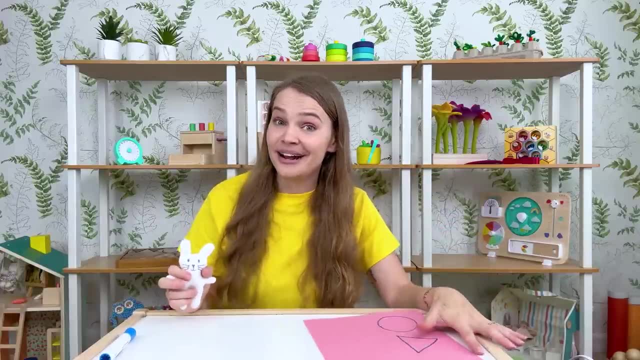 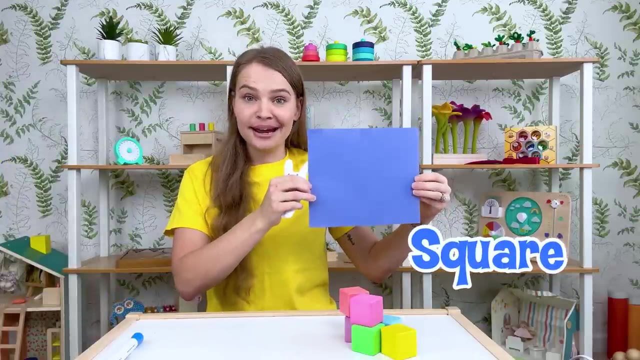 Now we've got a circle and a triangle. Bunny can go. hop in the circle, hop in the triangle. Let's learn about more shapes. How about a square? Let's learn about a square. This is a square. This is a blue square. 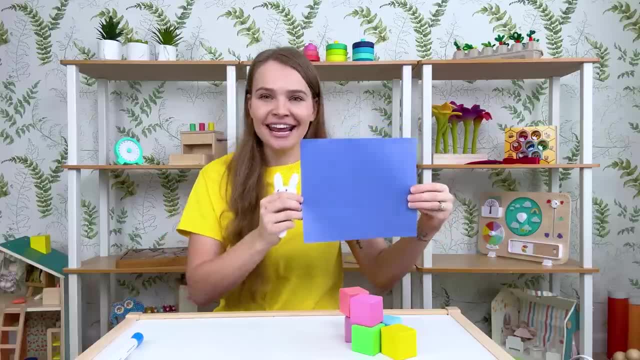 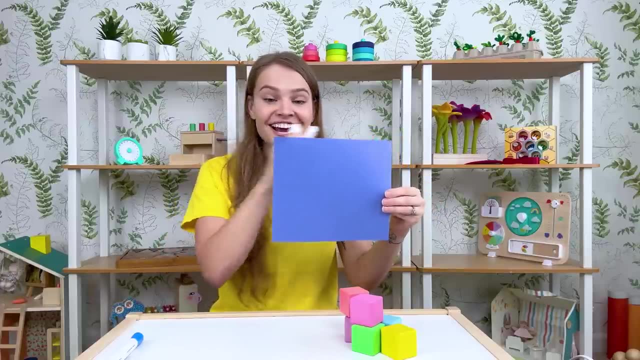 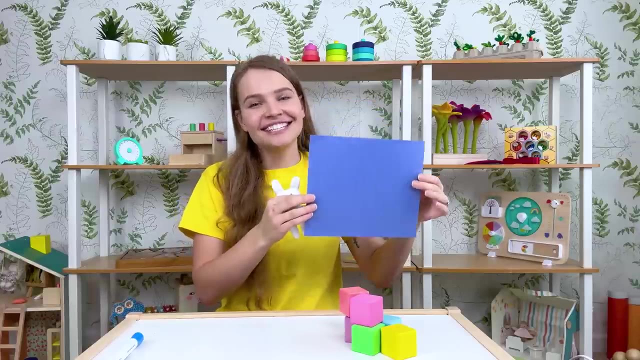 The square says square, square, Square, square, Square is my name, with four sides that are all the same. This side is the same as this side, same as this side and it's the same as this side. Four sides that are the same and four corners. 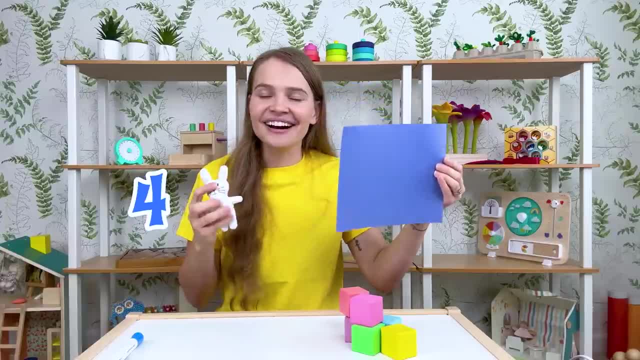 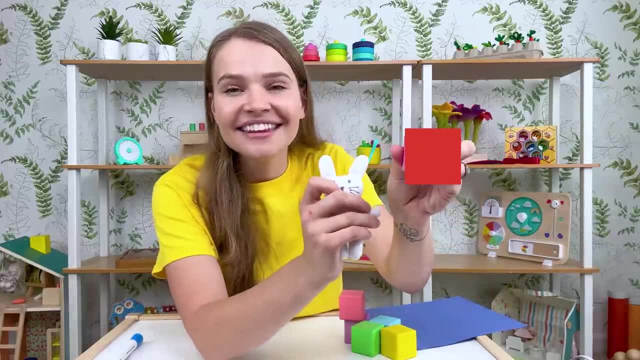 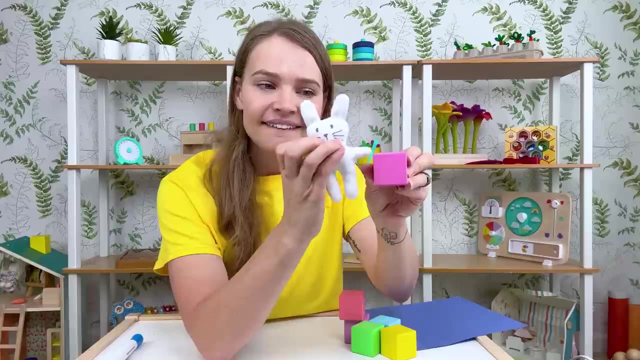 One, two, three, four Square. you can find a square on your blocks. You see the square. Let's count the sides: One, two, three, four and four corners. One, two, three, four, four corners. 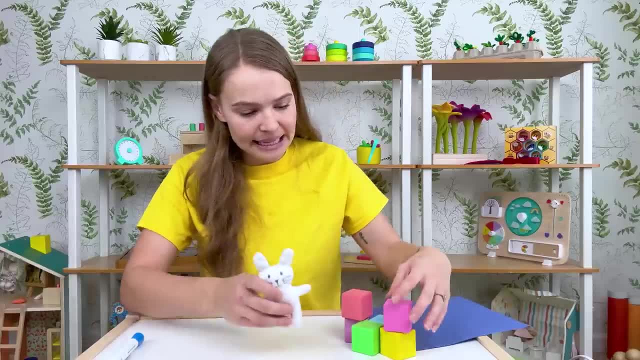 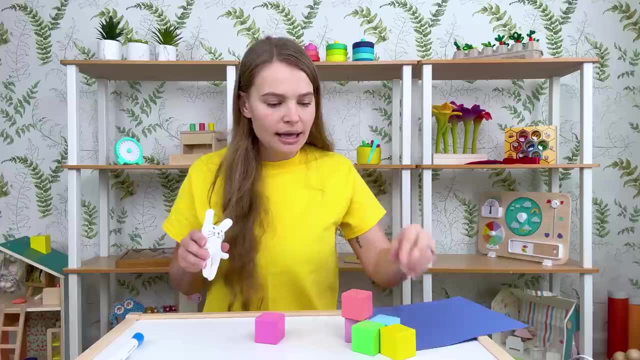 Let's stack our blocks that have squares on them. Let's see, Bunny, maybe you can help me. The pink one Next let's do. how about a yellow one? It's your turn. Do you want to put it on? 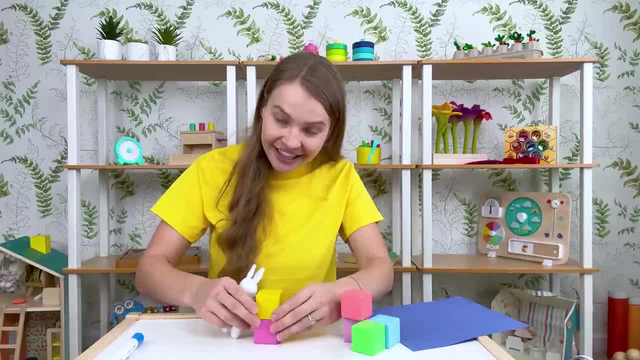 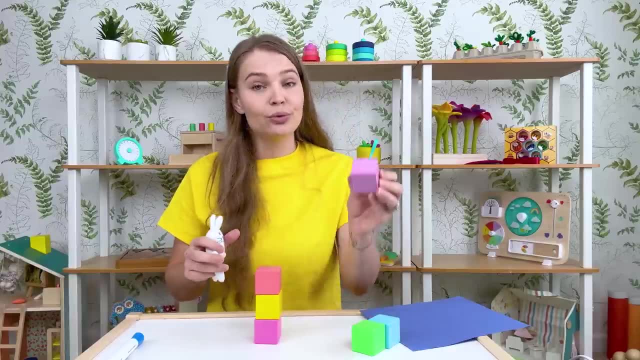 We'll help you. Here we go, Put it on, Stop stacking. How about this one? Let's put it on. And, ooh, a purple one. You go, Bunny, You want to do it, Stacking it on. 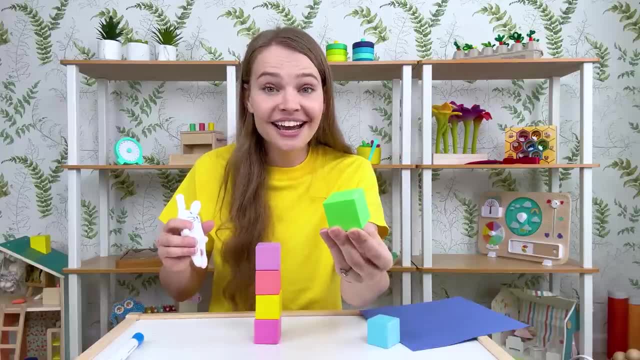 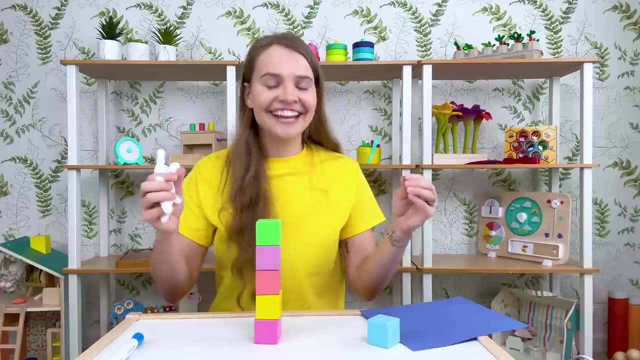 How about a green one? It's your turn. I'll help you put it on. Ready, Carefully, carefully, slowly, slowly put it on. And how about a blue one? Put it on. Oh wow, Look at our tower. 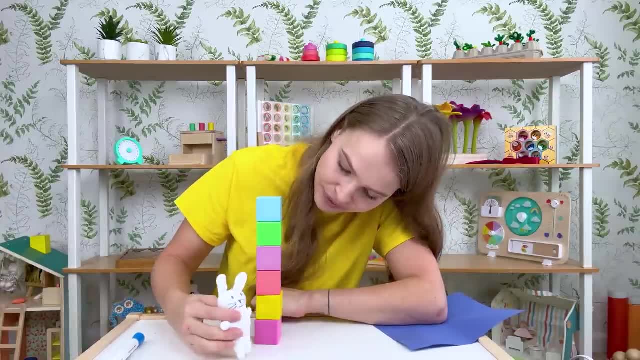 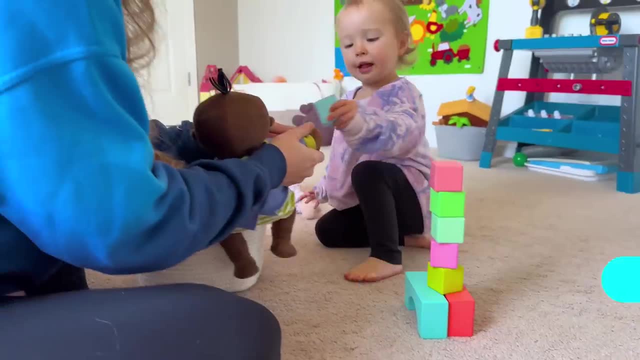 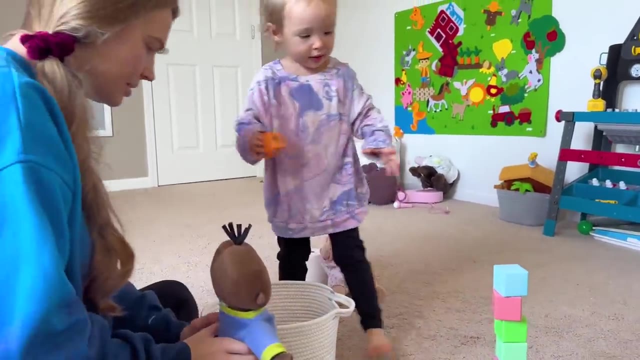 Sliding with it on, It's got many different squares And we learned that square has four corners and four sides. Oh, Bezio, Thank you, baby, You're very welcome. Thank you, Okay, show me, show me. 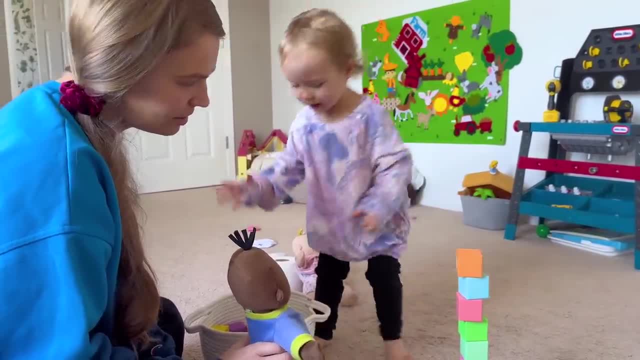 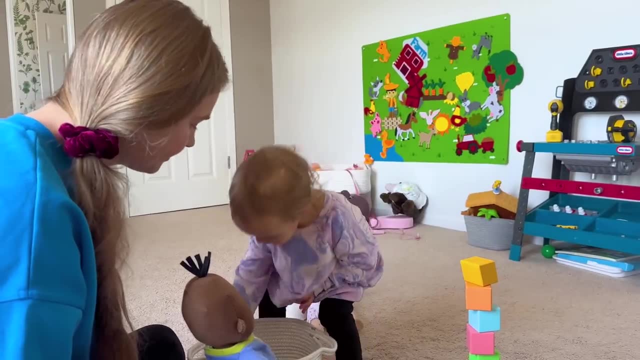 The boop And then the boop. I like that Boop. What kind of colors you got over there, girl, I'm sorry. Okay, I like that. Put them on a block. Oh, Let's draw a little face on this square. 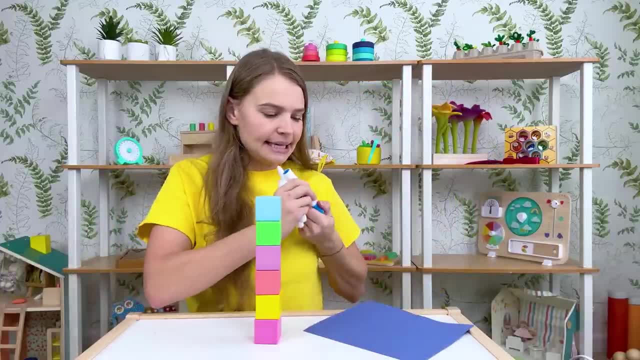 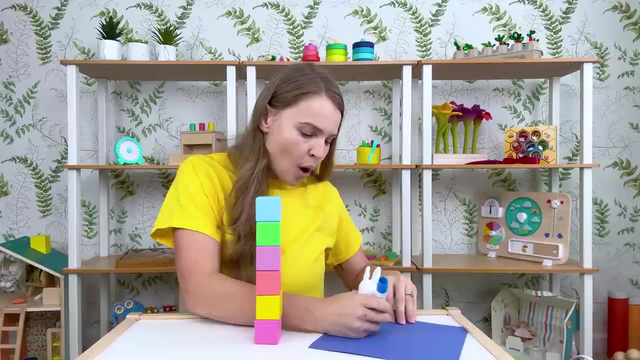 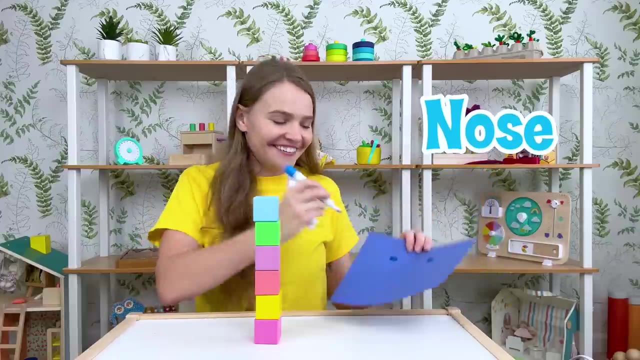 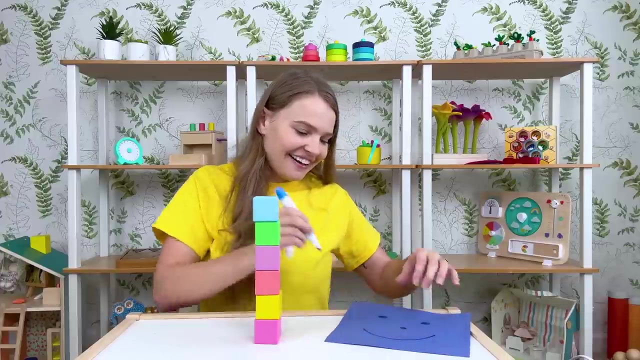 and we'll join our little shapes family. Let's see What is it that we draw to make a happy face, Two eyes, One Two And A nose And mouth, Mouth. Close the lid. Hi, happy square. 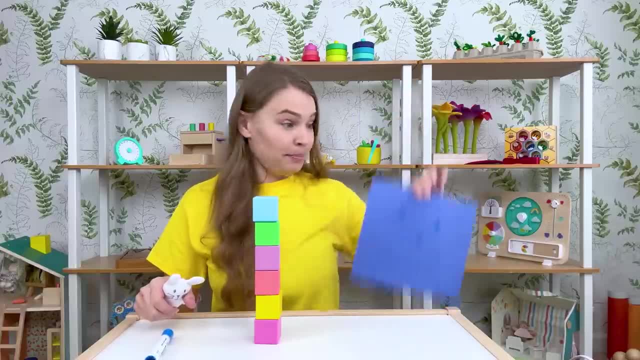 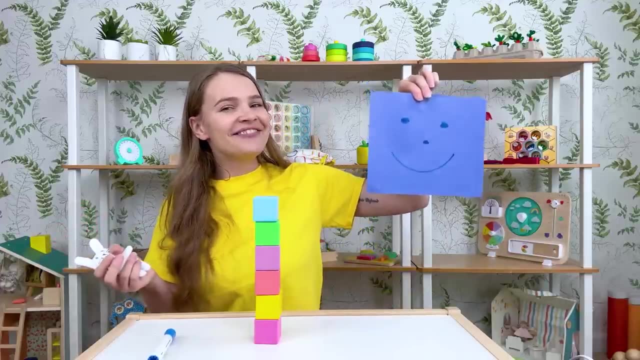 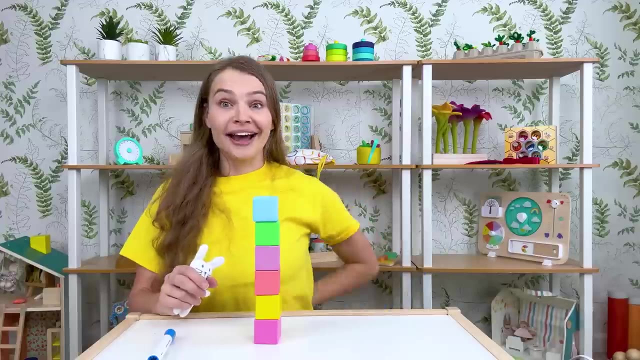 Oh, where did it go? Peek-a-boo, Peek-a-boo, Where is square? Where is square? Here I am, Here I am. How are you today, sir? Very well, I thank you. Run away, Run away. 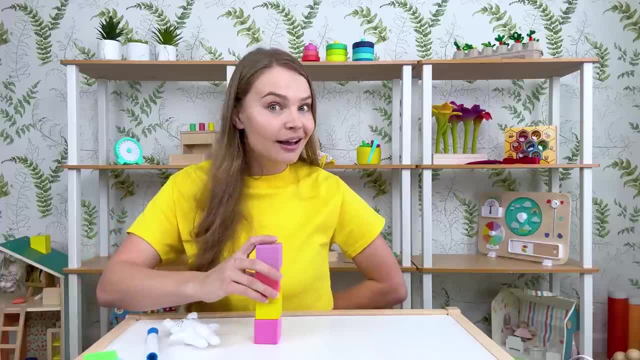 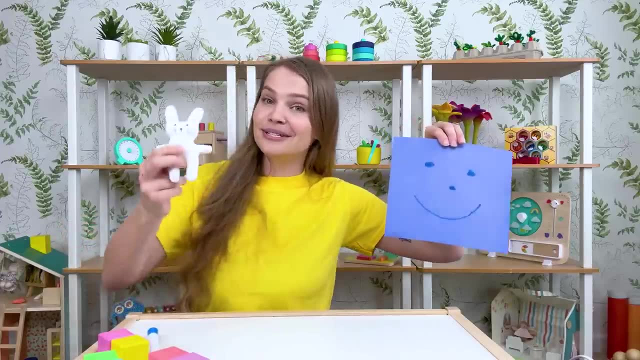 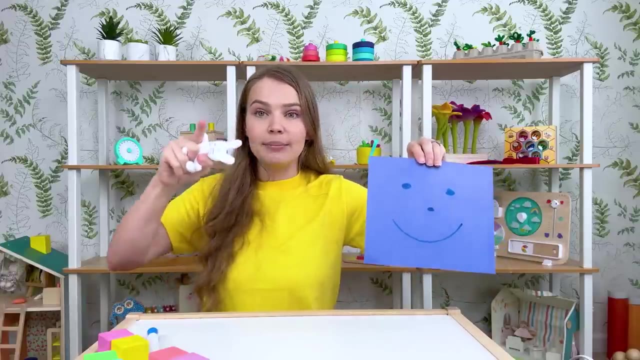 Where did that silly square go? Behind my back? Peek-a-boo square, Silly square. Oh wow, It was so nice to learn about squares. Bunny, do you want to draw a square? You have to draw four lines And make them all into a square. 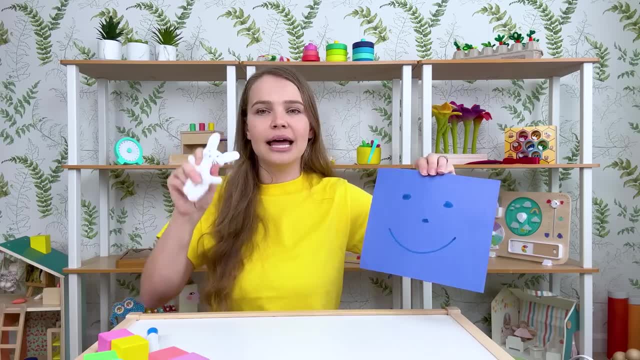 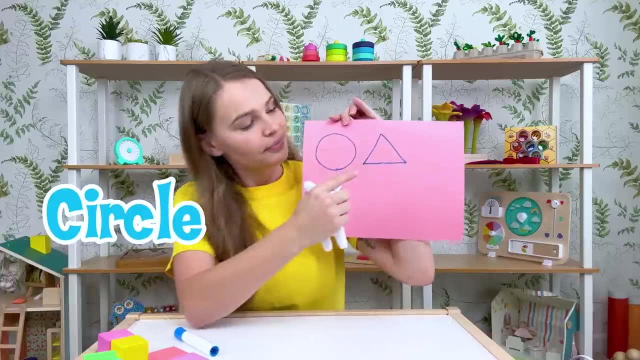 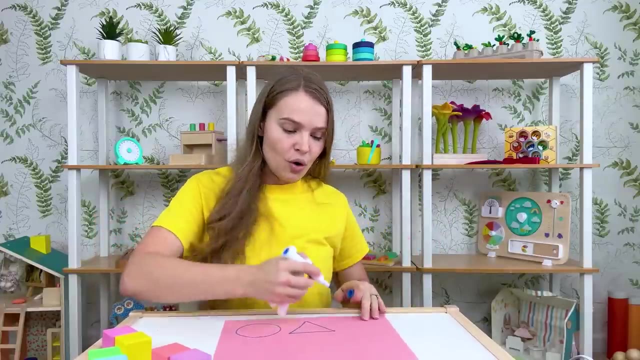 We can add it on your shapes paper. You want to. Oh, I would love to. Let's do it. We've got our paper with our shapes. So far we have circle Triangle and let's draw a square. let's see, we'll do one line down, one line over another line down. 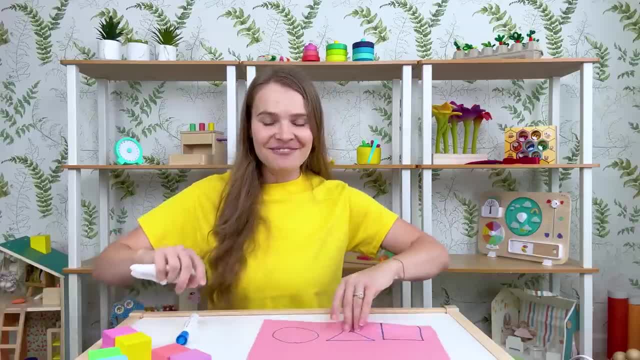 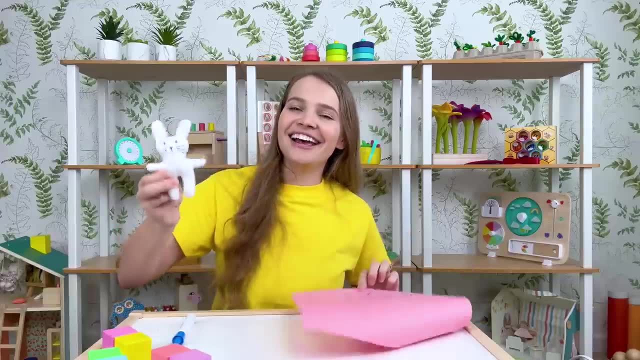 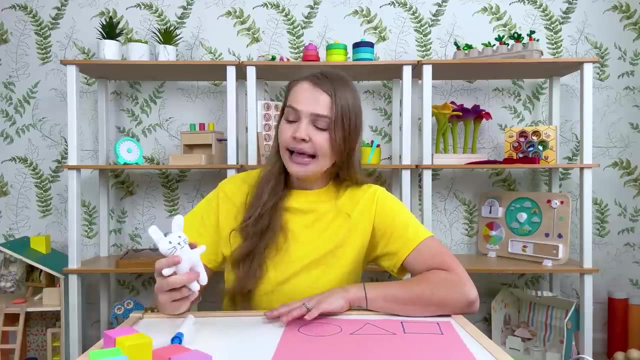 and connect them all. now, finally, you've got a circle, a triangle and a square. bunny says: i love learning about shapes with you. thank you so much for teaching me. you're really good at your shapes and your colors. let's learn about more shapes. how about, oh, a rectangle? let's do it. 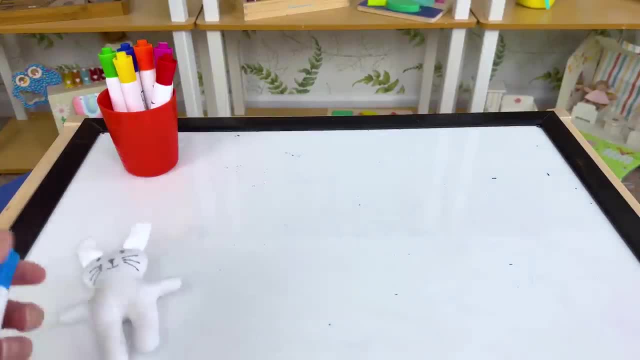 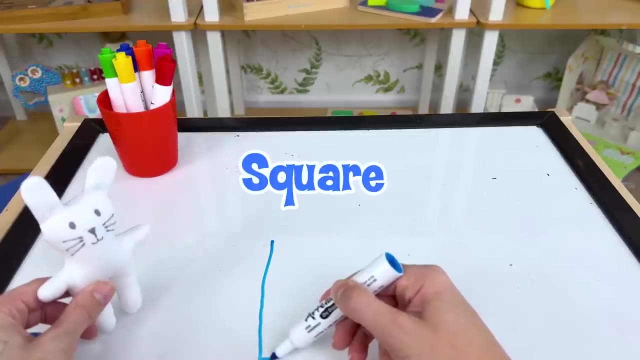 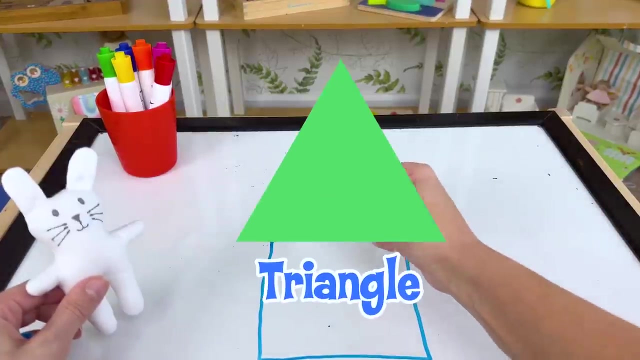 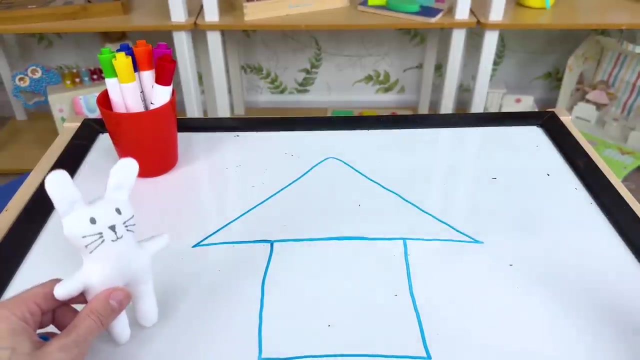 let's help bunny draw some shapes. here we go, bunny. how about a square? has four sides? one, two, three, four a square? what about a triangle up top? a triangle has three corners and three sides. well, that kind of looks like a house. what if we put a circle in here? 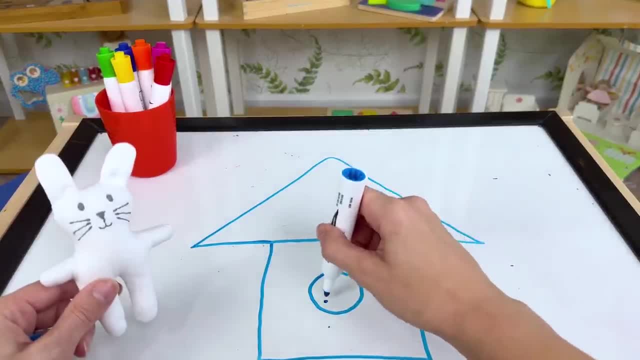 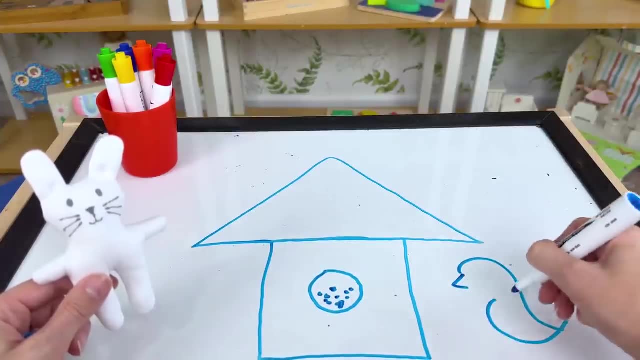 that looks like a birdhouse. huh, let's put some seeds inside, seeds inside for the bird. let's draw a little birdie here. tweet, tweet, tweet, tweet, tweet says the birdie, tweet, tweet, tweet. two eyes smiling birdie says tweet, tweet, tweet, tweet, tweet. thank you, thank you, i love. 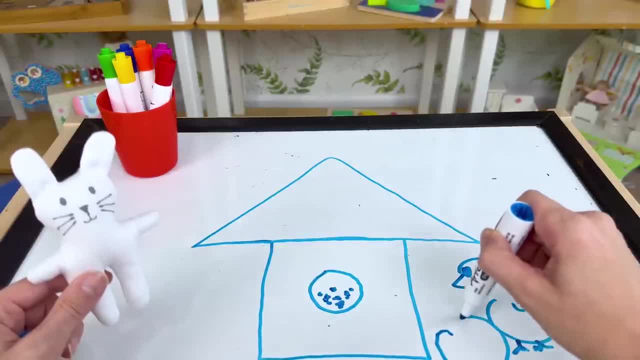 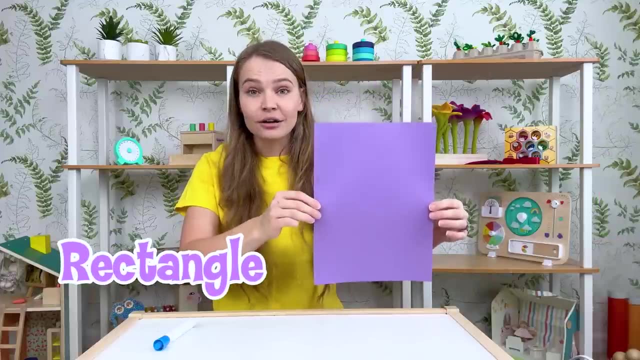 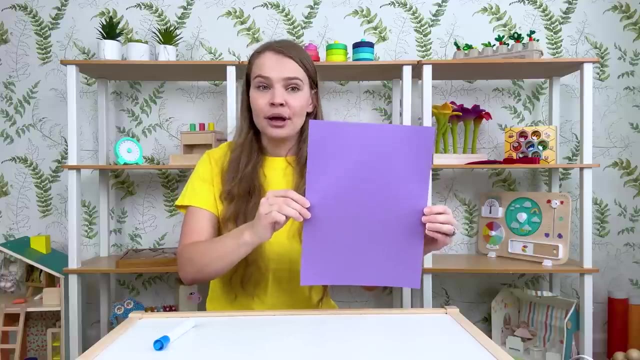 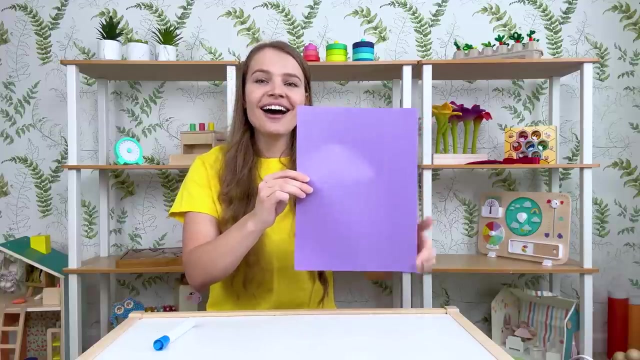 to eat these seeds. here's some water for you too, birdie, so you don't get thirsty. enjoy. this is a rectangle. this is a purple rectangle. this one says: purple rectangle is my name. my four sides are not the same. two are short and two are long. count my sides, come right along one. 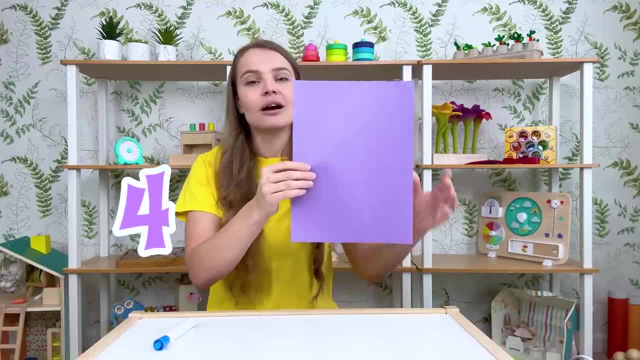 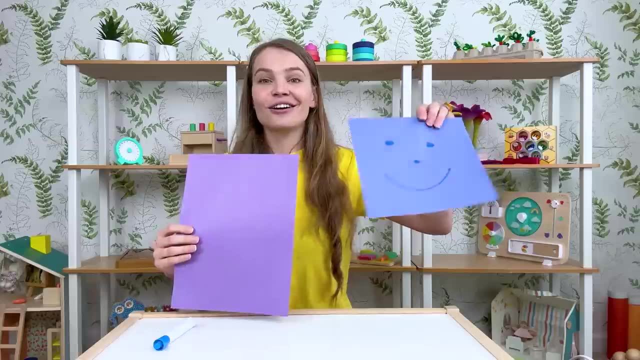 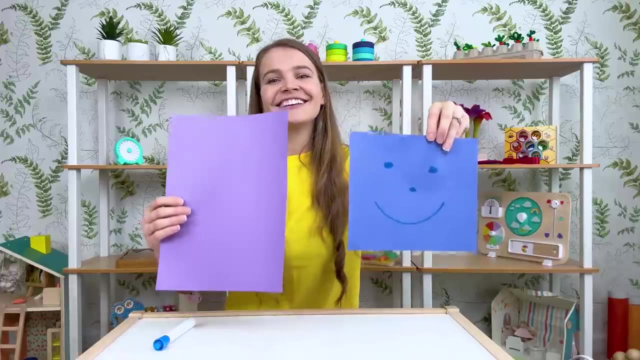 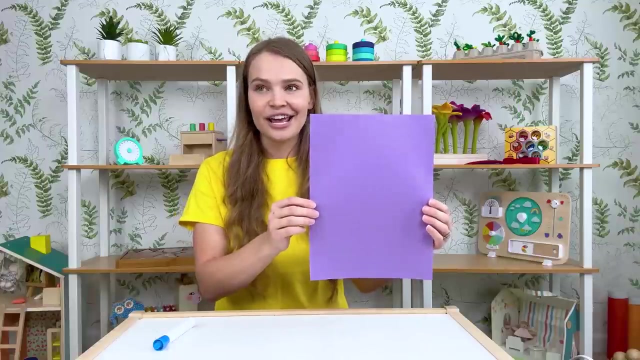 two, three, four. a rectangle is really similar to a square, but it's longer. let's see, here's our square, here's a rectangle. they both have four sides, but the rectangle is longer. this is a square, this is a rectangle. you might find the rectangle shape on a door or a book, or a book piece on a book. Ross, look, i'm- not sure. i'm very good, you come help mearmella. 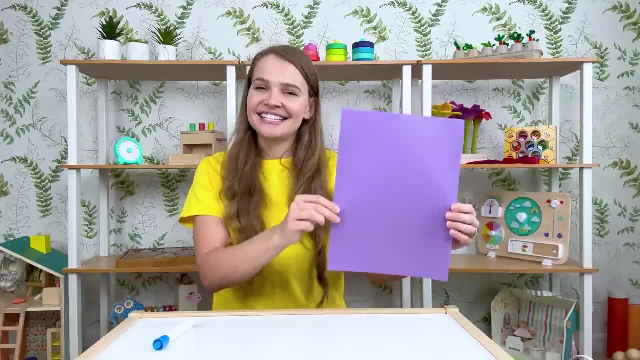 is making a flower bunch, but you can't find a flower about two feet away, apart from the master deathعد or a piece of paper. This is a rectangle. Let's draw another happy face on it and it can join our little shapes family. 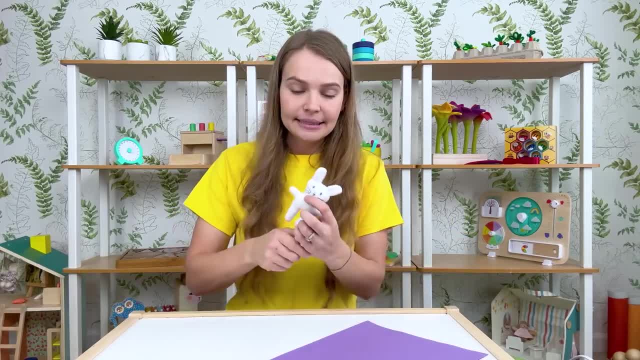 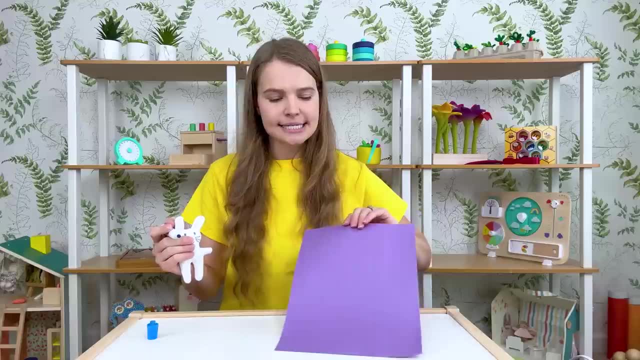 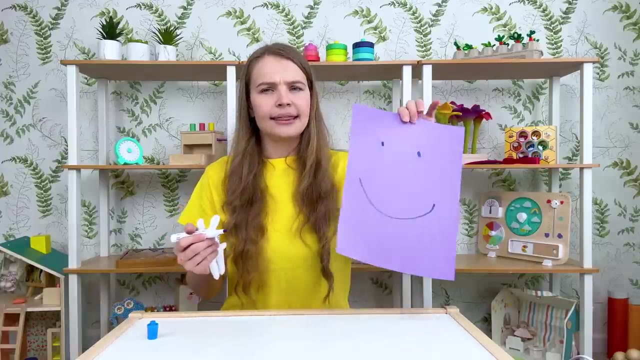 Bunny, where are you? Peek-a-boo, here are you. Let's see, Bunny. What do we draw to make a happy face? Is it one eye, Two eyes, One two and a mouth? I think we're missing something. 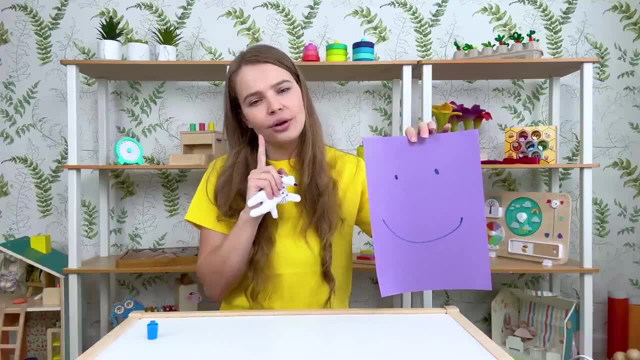 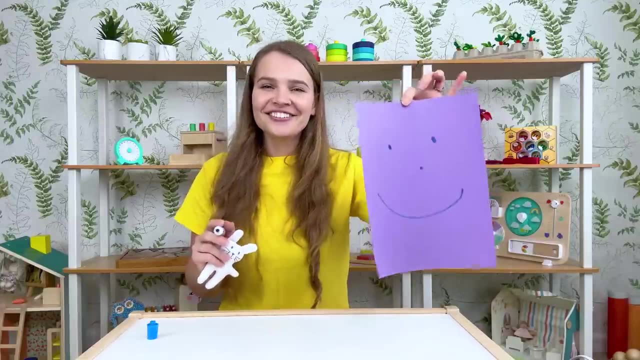 We've got the eyes, we've got the mouth. A nose, Nose is what we need. Here you go, peep-a-boo. Hello, rectangle, Where did it go? Did it go under the table, Peek-a-boo? 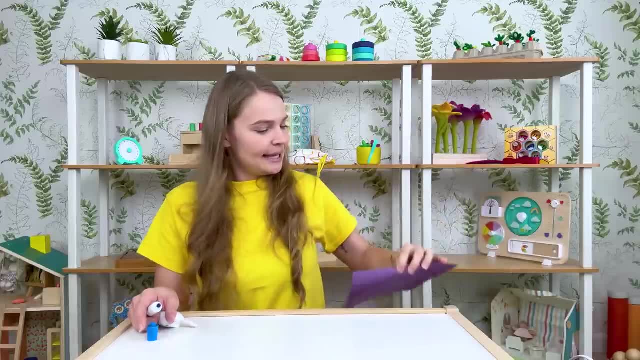 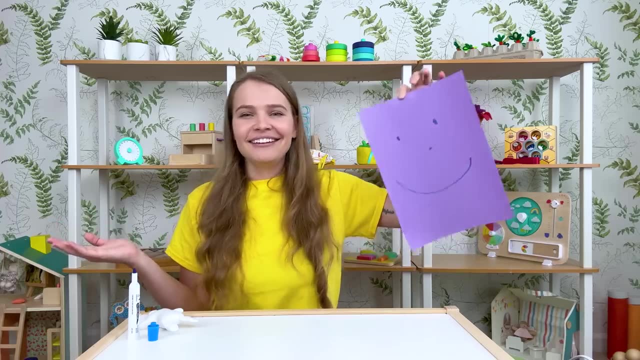 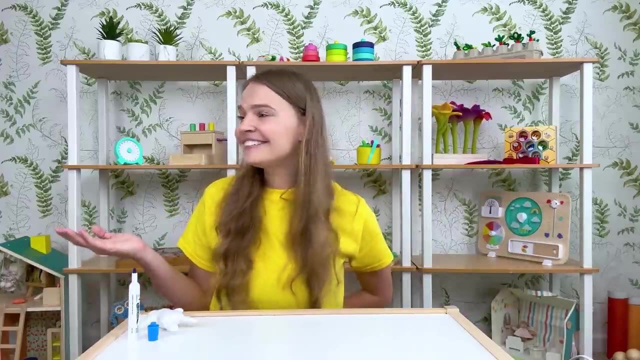 Rectangle, you silly rectangle. Where is the rectangle? Where is the rectangle? Here I am, here I am. How are you today? How are you today, sir? Very well, I thank you. Run away, run away. Oh Bunny, do you want to draw a rectangle? 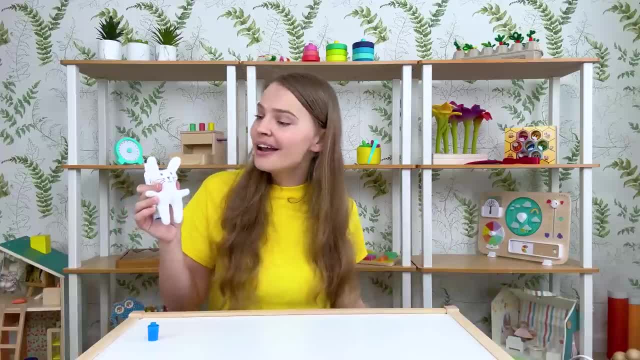 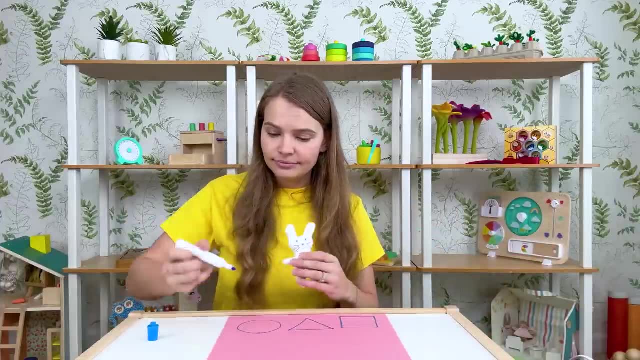 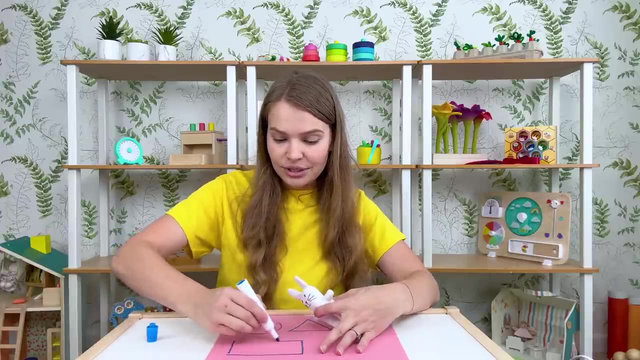 Oh, I'd love to draw it. Let's draw it on your piece of paper with all your other shapes. Let's see Now, rectangle. it's got four sides and four corners, like the square, But two sides are long and two sides are long. 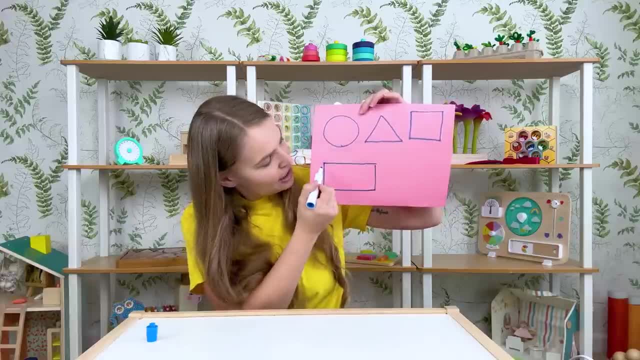 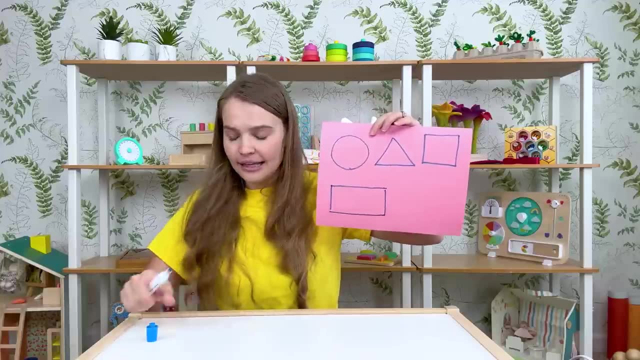 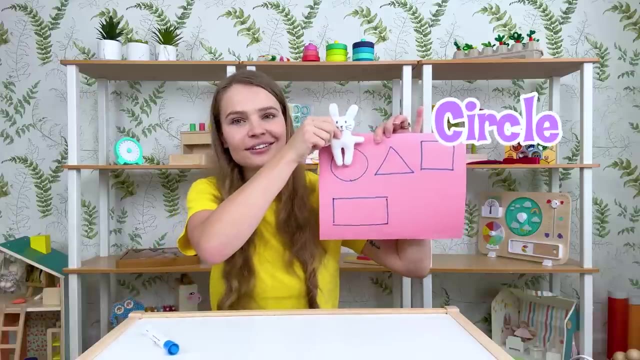 Two sides are short. Now we've got a rectangle. There's two sides that are short and two sides that are long. Here you go, Bunny. Let me close my marker And you can hop in your shapes. Bunny, hop in circle. 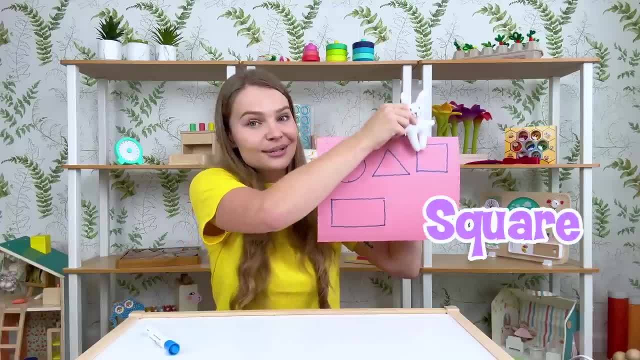 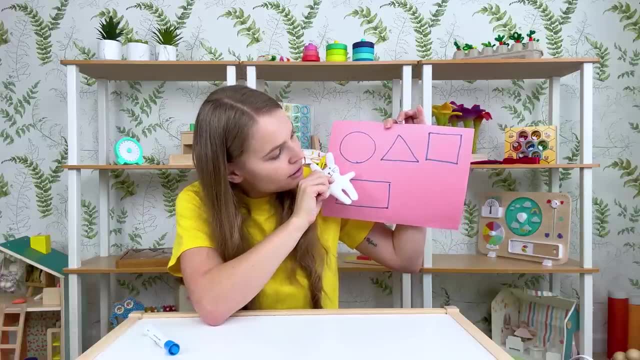 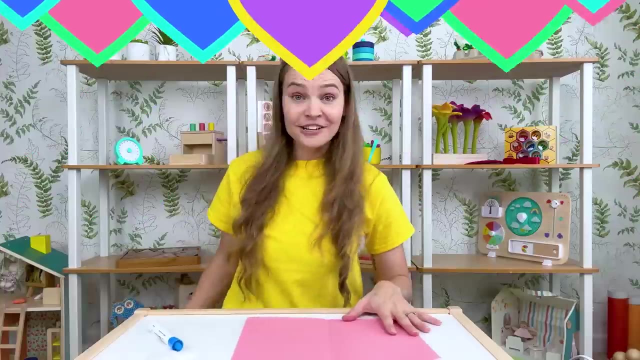 Bunny hop in triangle, Bunny hop in square, Bunny hop in rectangle. We've got a little space for another shape. Hmm, maybe let's do a heart, Let's draw a heart together. First let's cut out a heart, And you can ask your grownup for help with the scissors. 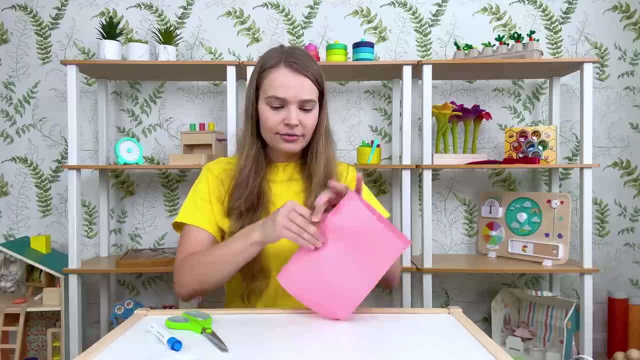 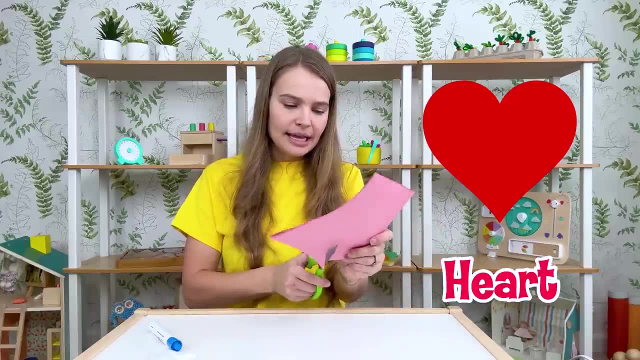 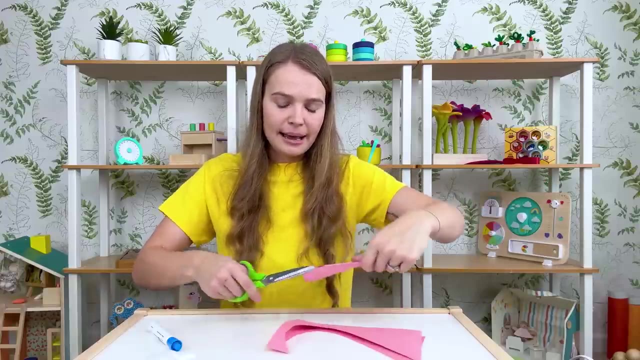 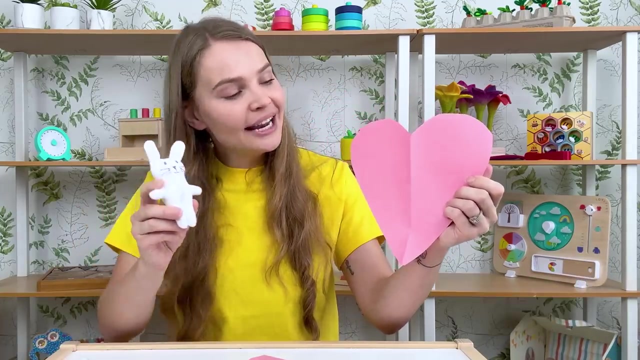 I'll fold my piece of paper in half And a heart kind of has that corner at the bottom And it's got two half circles up top, So let's round it at the top And here's a heart. Oh wow, says Bunny. 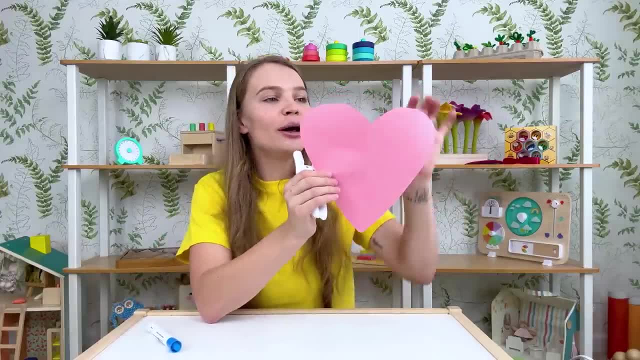 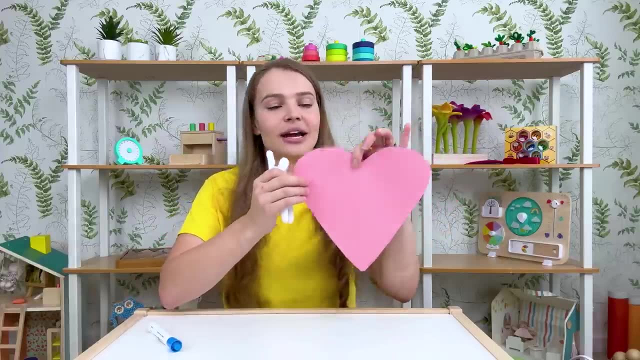 This is a heart. It's got the one corner at the bottom and two rounded kind of humps up top And we draw a heart when we love someone And we can write I love you Mom Or I love you Dad. 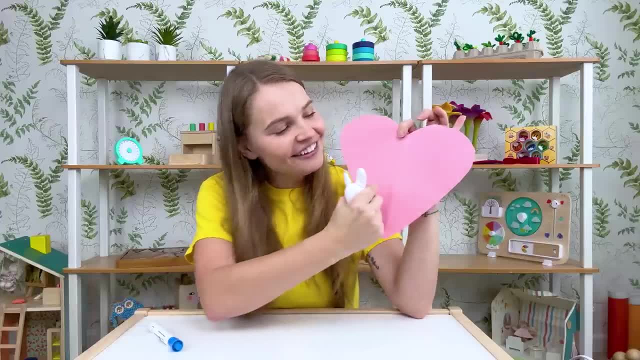 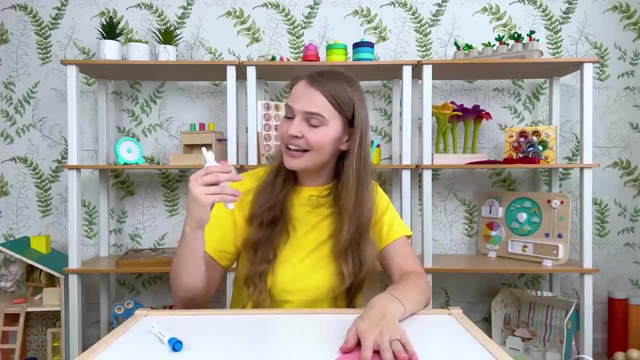 Or I love you Grandma, Or I love you Grandpa, And we can draw little hearts together. And we can draw little hearts together. And we can draw little hearts together. Let's draw one right now. Do you want to draw your heart? 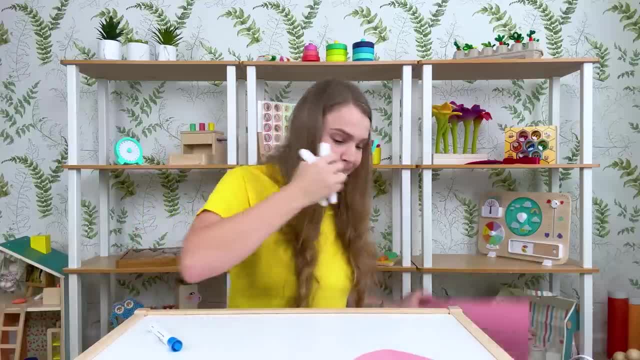 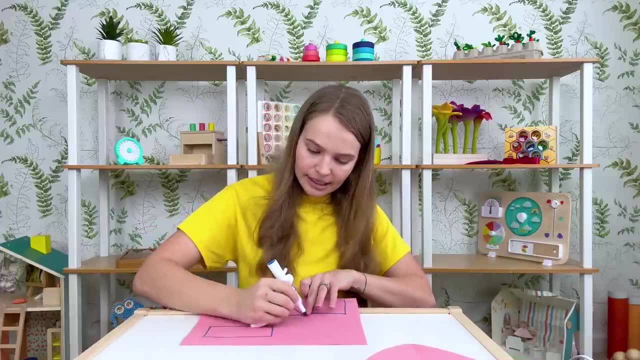 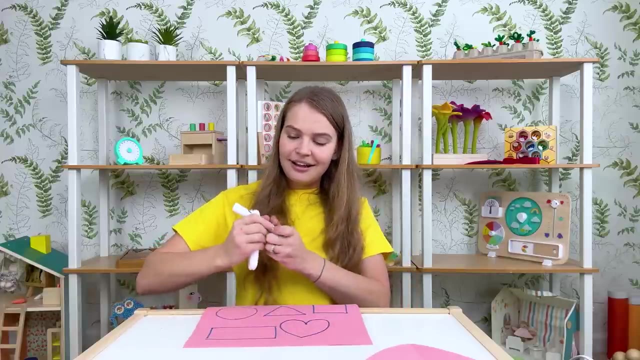 I'd love to draw my heart. Okay, Bunny, let's get your piece of paper. Let's see, Maybe we can draw a heart right here, And it goes round and down, And round and down. All right, Bunny, Now you can hop in your shapes. 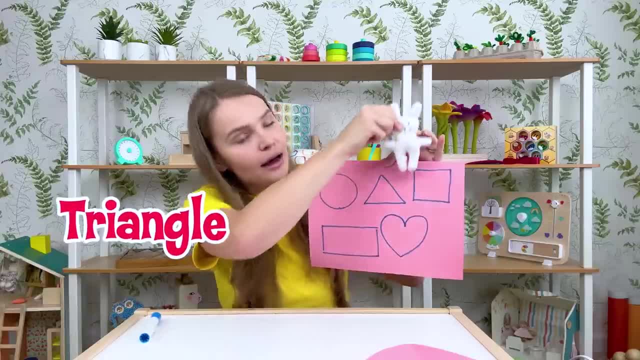 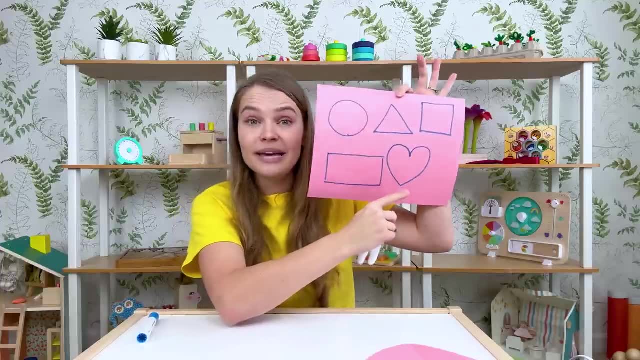 You can hop in a circle, Hop in a triangle, Hop in a square, Hop in a rectangle, Hop in the heart, And I saved a little space for one more shape, a star shape. Do you want to help me make a star? 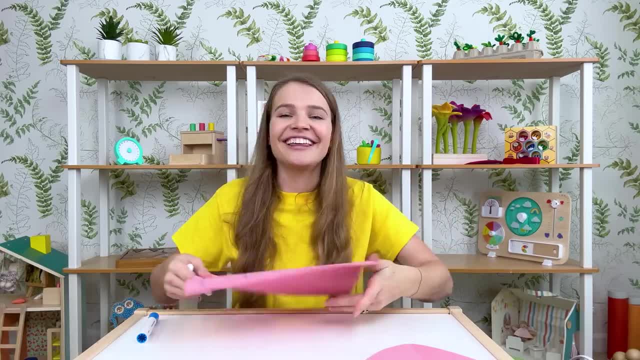 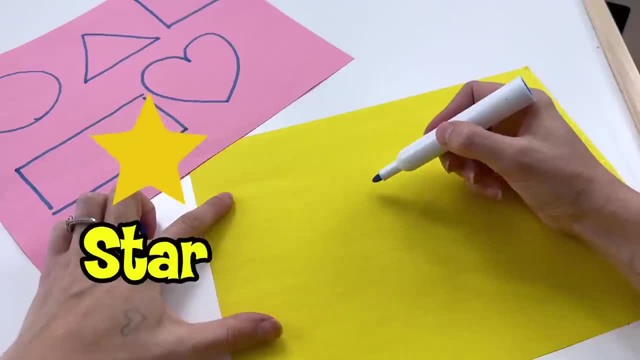 It's got five points. It's a lot of points, but I think we can do it. Let's do it together. A star has five points and they all each kind of look like a triangle. Do a triangle up here, but we won't connect the bottom. 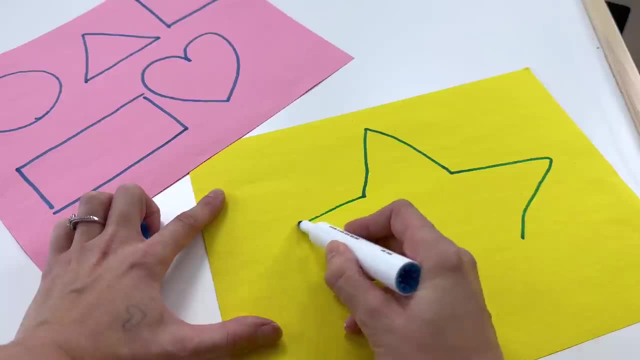 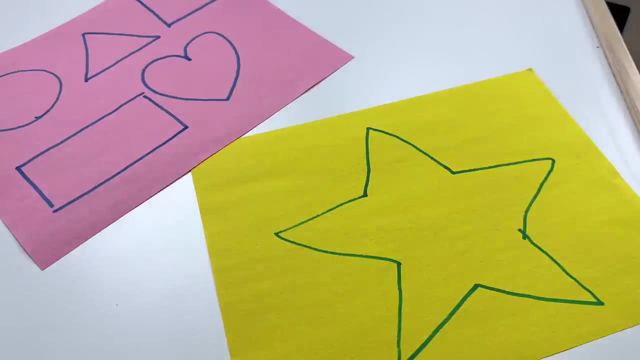 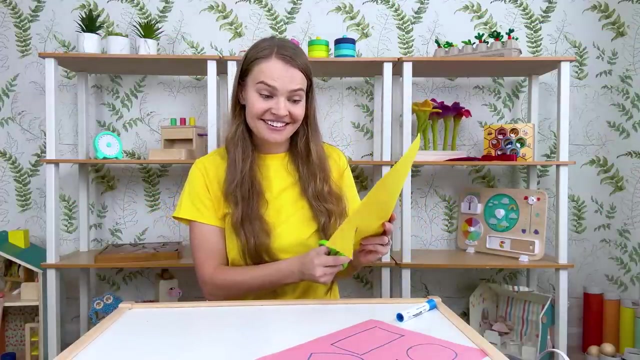 Another triangle, Another triangle, Another triangle, One more triangle and we've got a star. Let's cut it out. All right, let's cut out our star together, and then we can add a little happy face on it, And then we'll help Bunny draw the star in the paper. 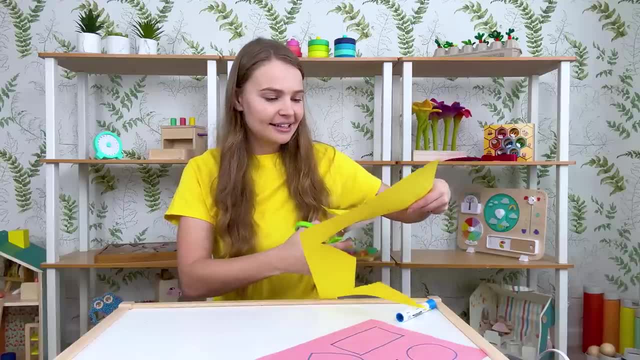 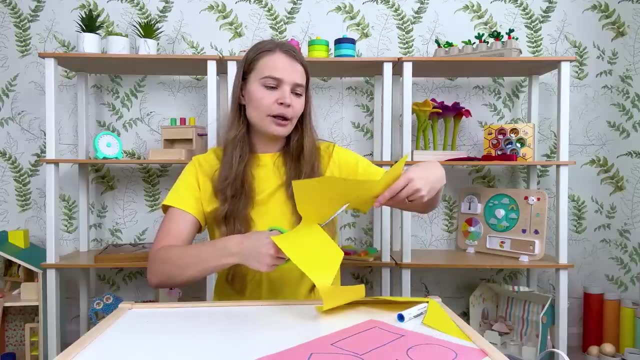 And Bunny will have all of the shapes to hop on. We did a great job learning our shapes. Great job learning our shapes today, huh, and helping Bunny. You're a good helper and you're a good friend. All right, we've got a star. 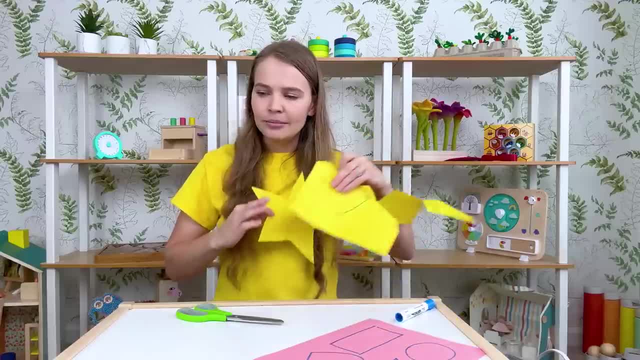 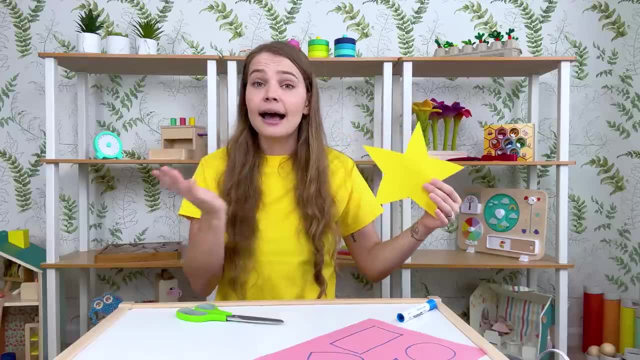 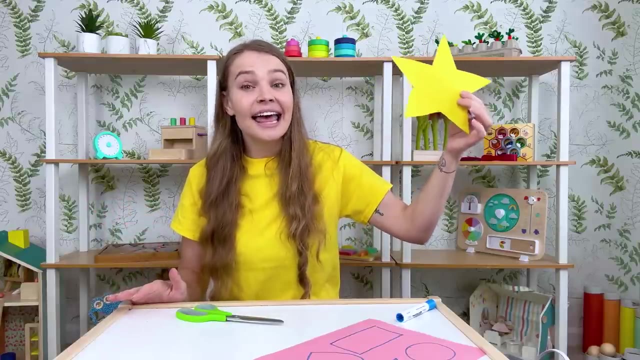 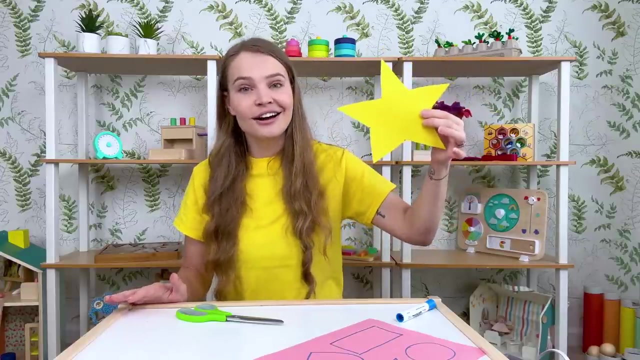 Now, do you know a song about a star, Maybe? Twinkle and Twinkle and Twinkle, twinkle, Twinkle little star. how I wonder what you are, Up above the world, so high Like a diamond in the sky. twinkle, twinkle, little star. how I wonder what you are. 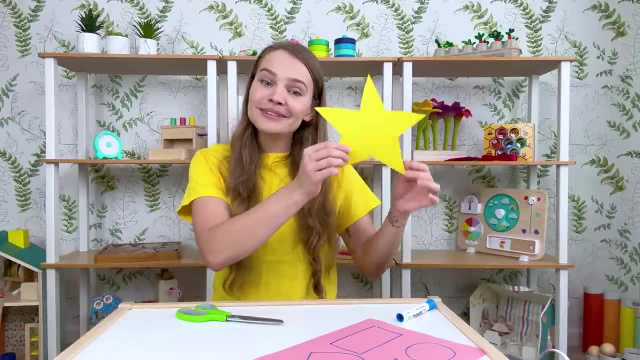 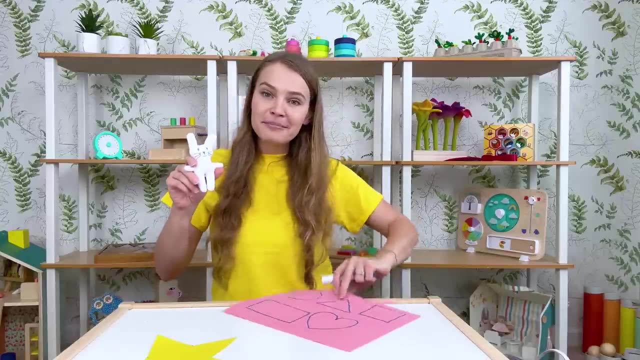 Yay, This is a beautiful star. You did a great job helping me draw it, Bunny. where are you? Hop, hop, hop, hop, hop. Let's draw the star at the bottom of your paper here, And you have all your shapes. 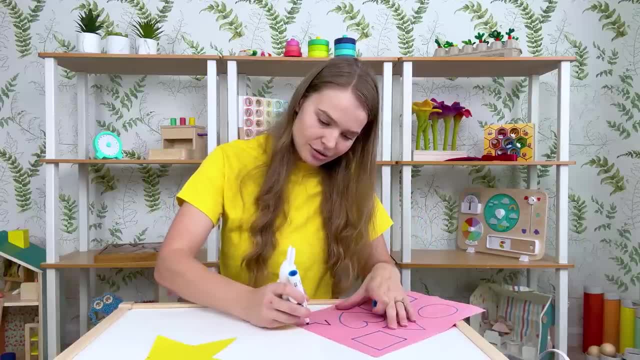 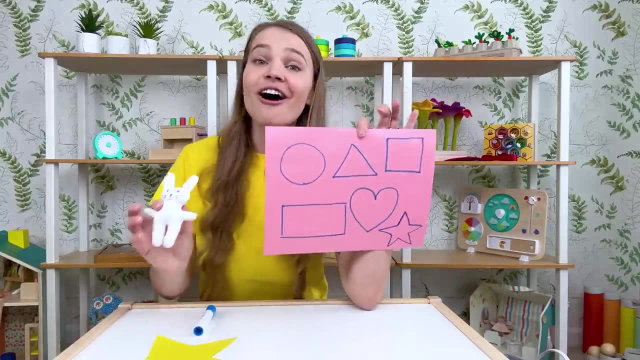 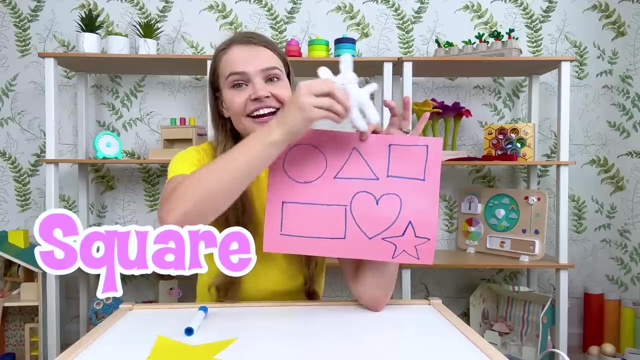 Let's see, We'll draw the triangle. Yes, you have five points. Wow, Look at all of the shapes that we learned today. We've got a circle, triangle, a square, a rectangle, a heart and a star. 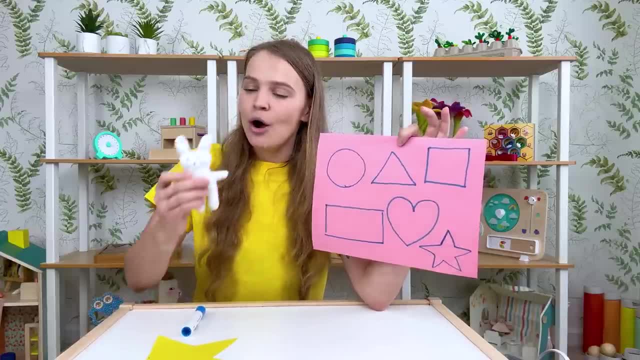 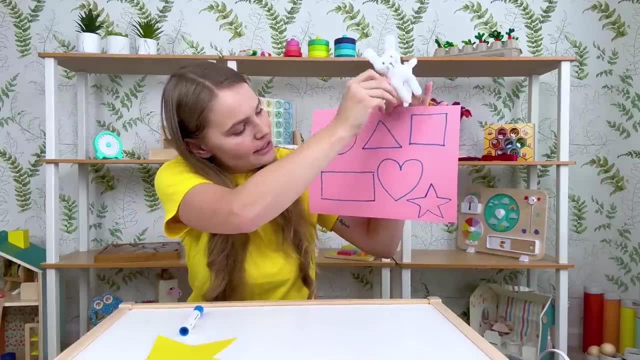 Wow-wee, That's a lot of shapes. Oh, I'd love to hop through them. Let's hop. Hop in the circle, hop in the triangle, hop in the square, hop in the rectangle, hop in the heart, hop in the star. 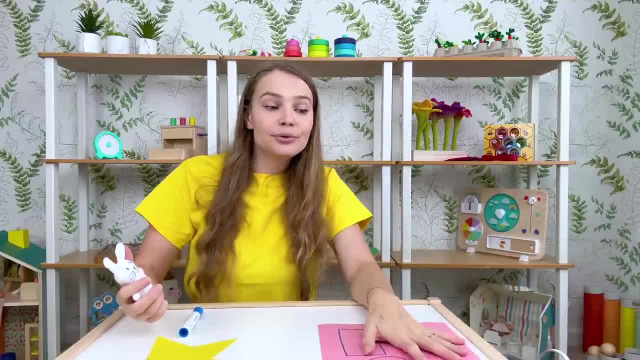 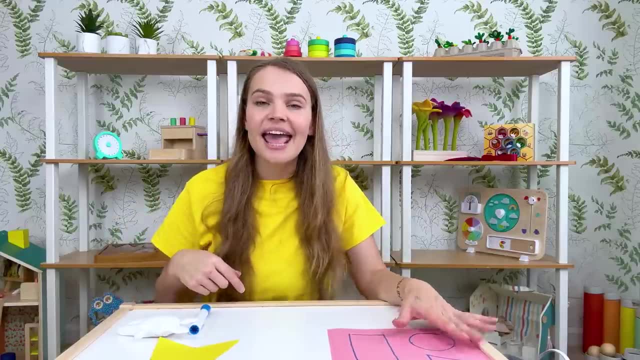 Something that's really fun to do is if you have some blue tape, some blue painter's tape, at home, and then you can ask your grown-up for help. you can tape the shapes on the floor and then go hopping in them or practice walking slowly, slowly, slowly. 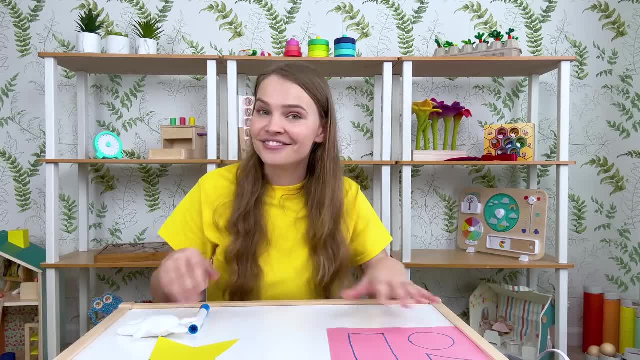 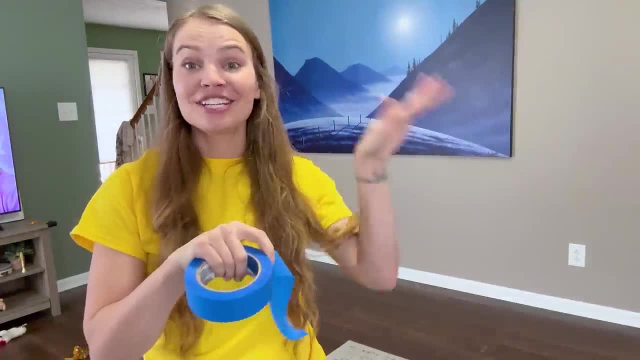 Oh, jumping them. It's really, really fun. Let's do it together. Here's a fun activity you can do at home Now. you need some painter's tape and you can make shapes on the floor and then go jump in them or hop in them. 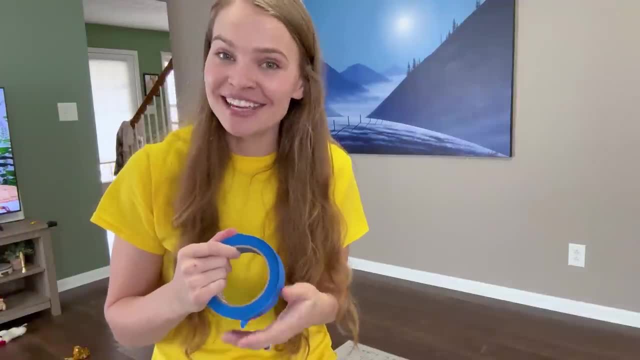 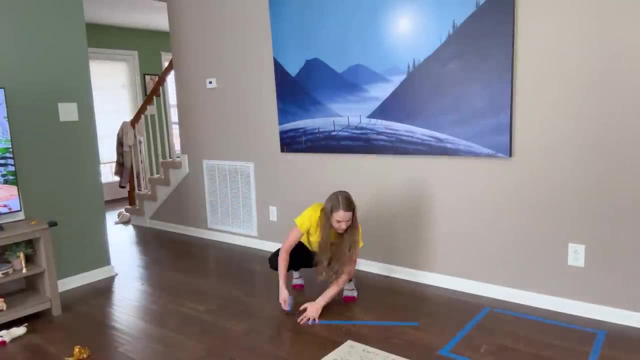 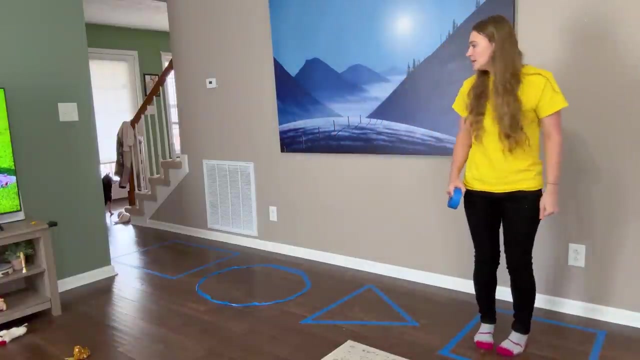 or practice walking slowly and carefully. So let's make some shapes, All right. Now let's hop in the circle and walk to the triangle, Walking, walking, walking. And let's run to the square: Run, run, run, run, run, run, run. 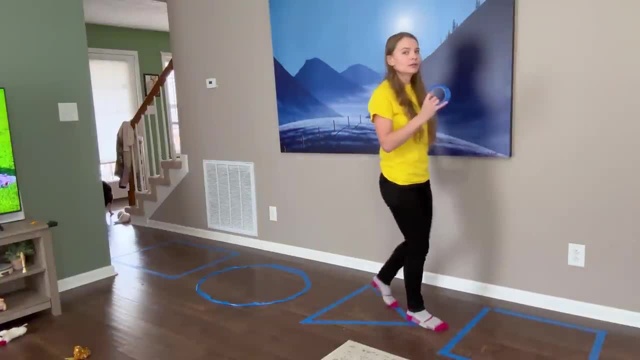 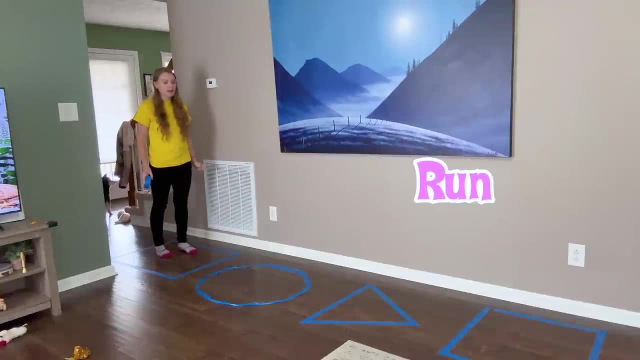 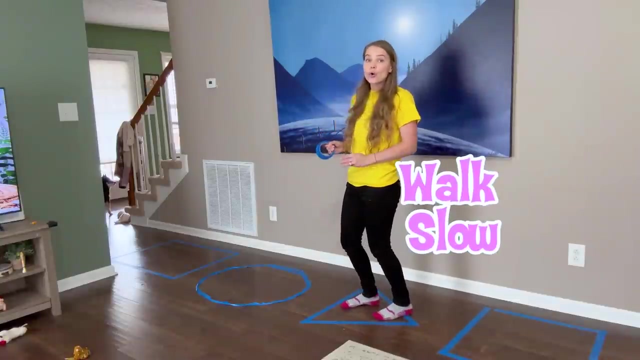 Let's walk backwards to the rectangle, Backwards, backwards, backwards, backwards, backwards, backwards, backwards. Now let's run fast to the triangle, Run fast, run fast, fast, fast, fast. Let's walk slow to the rectangle. 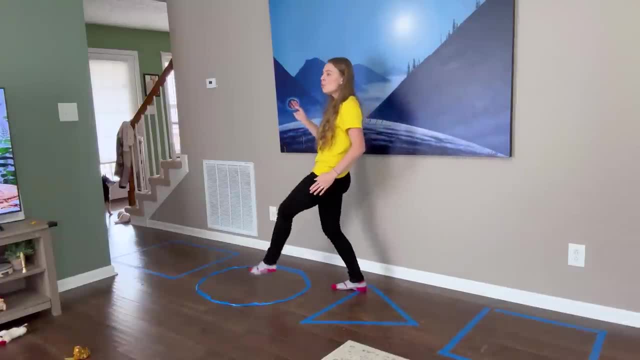 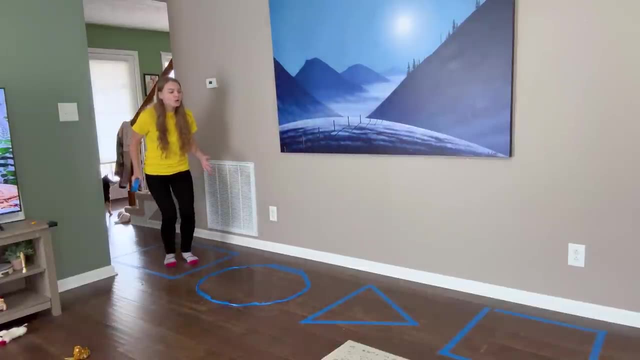 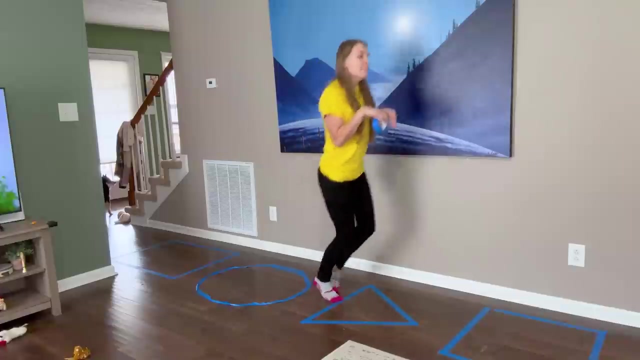 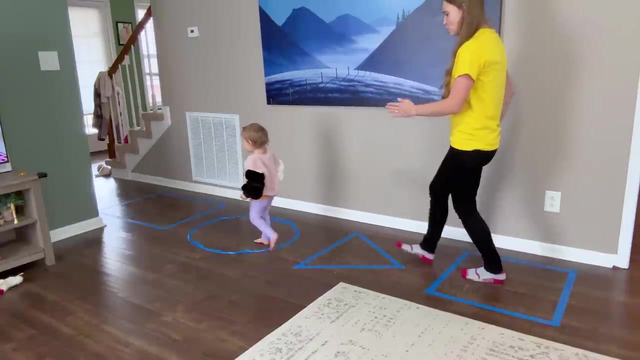 Slowly walking to the rectangle. Let's hop over to the square. Do you see the square Over there? Hop, hop, hop, hop, hop. Great job, hopping. You want to walk slowly to the rectangle? Yeah, Good job. 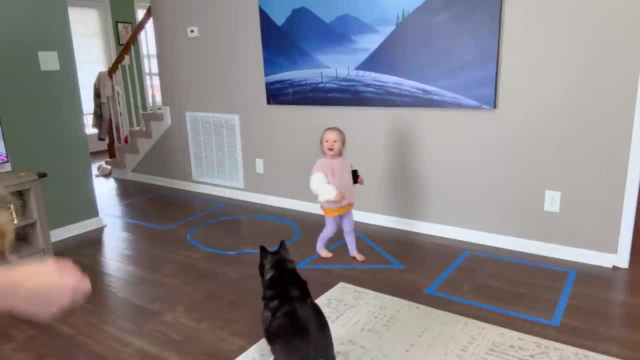 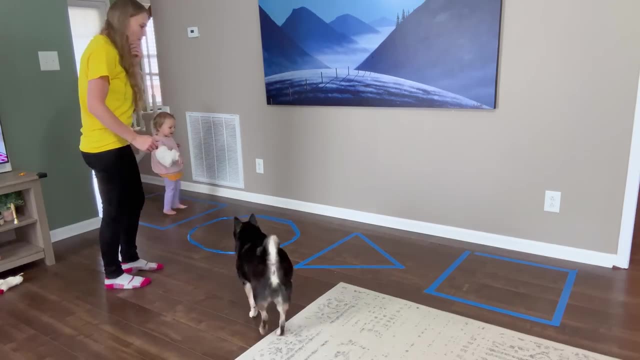 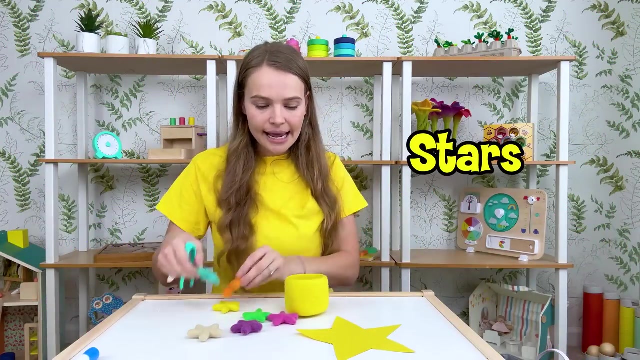 Okay, how about hop to the triangle Here? Yeah, Okay, where is the square In the rectangle? Ah, rectangle. Okay, how about I'll go in the square? Where should Paisley go? Right here, I've got some stars that I need to put into this yellow little bucket. 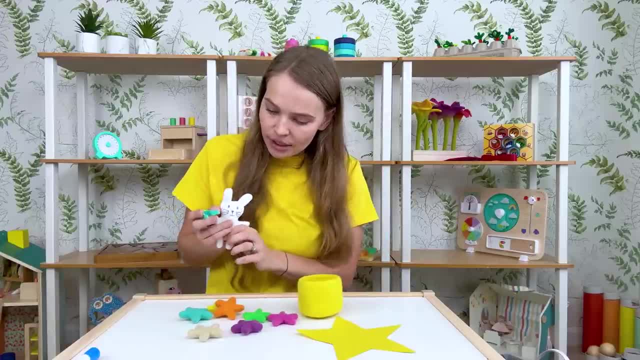 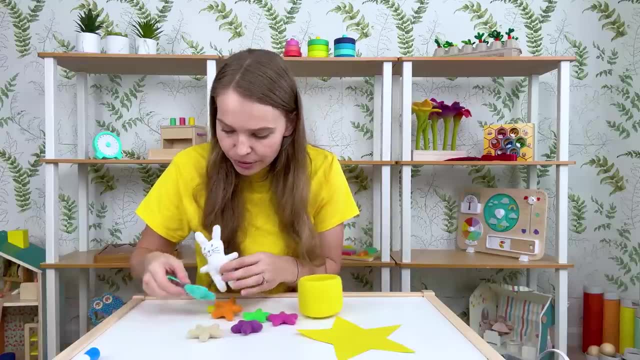 Will you help me put them in Here? bunny Let's, I've got these little tongs. They'll help me pick them up. Let's see First how about this blue one, Blue star, Put it in Now. let's grab the orange one. 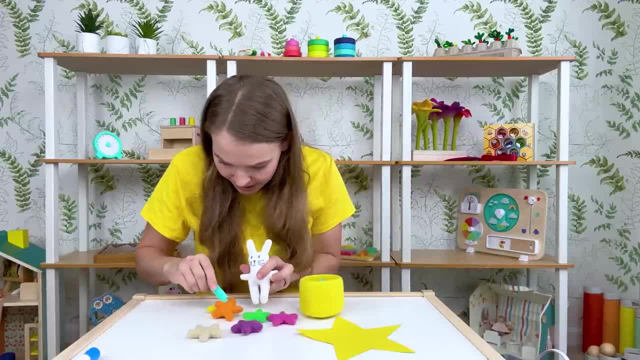 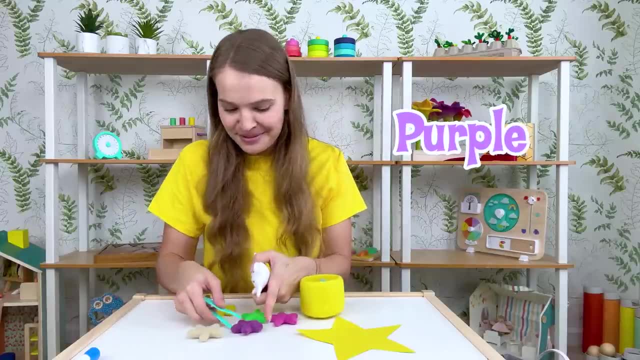 Do you see the orange one Right here? Pick it up, Put it in. How about a purple one? Here's a purple one. Thank you, Pick it up. Oops, Oopsie, daisy, I dropped it, That's all right. 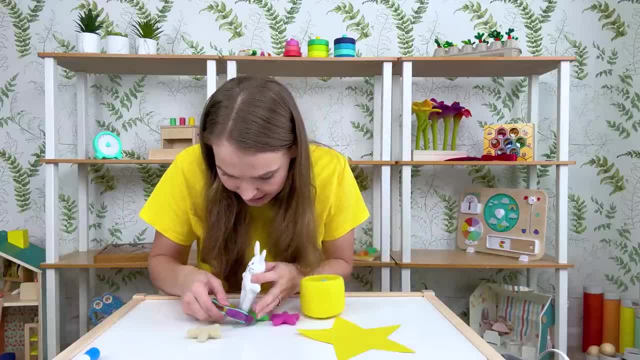 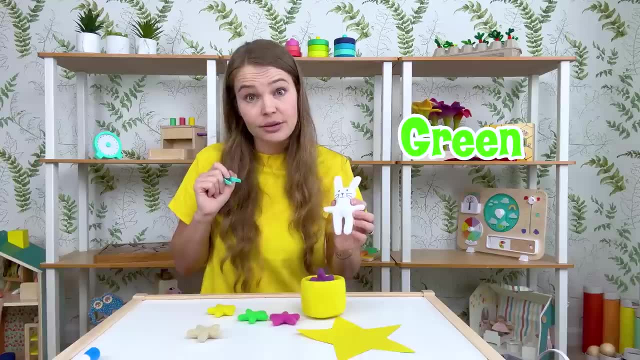 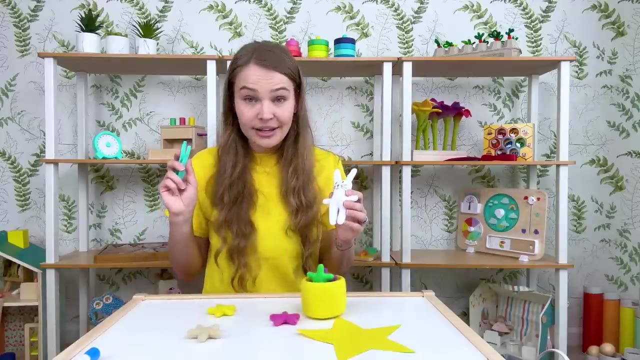 We'll pick it back up. I'll try again. Pick it up, Put it in, Let's see, I'm looking for a green star now. Do you see a green one Right here? Thank you, Green star in. How about a yellow one? 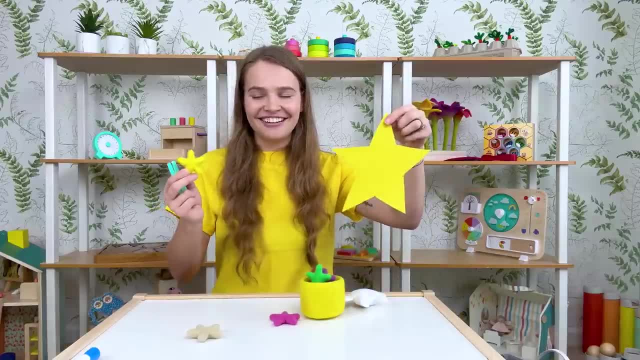 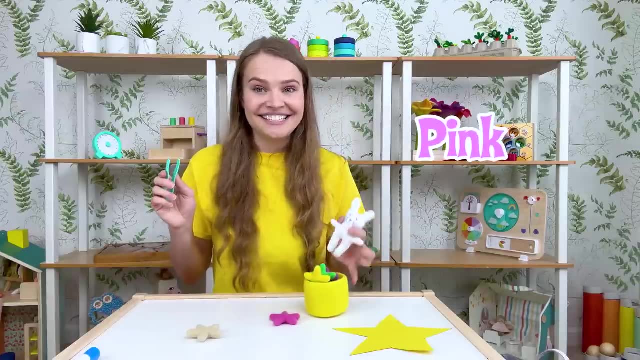 Well, there's kind of two yellow ones. huh, There's a big one and a little one. Let's grab the little one and we'll put it in Little yellow star in. How about a pink one? Do you see a pink one? 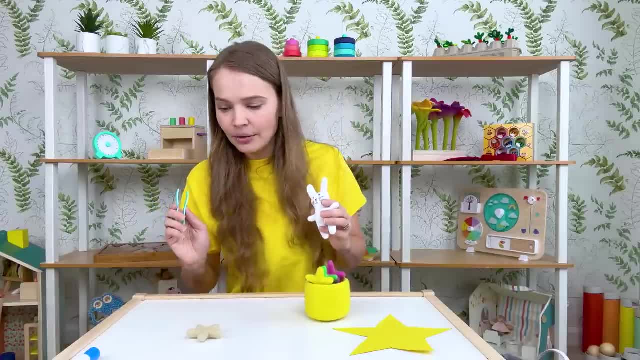 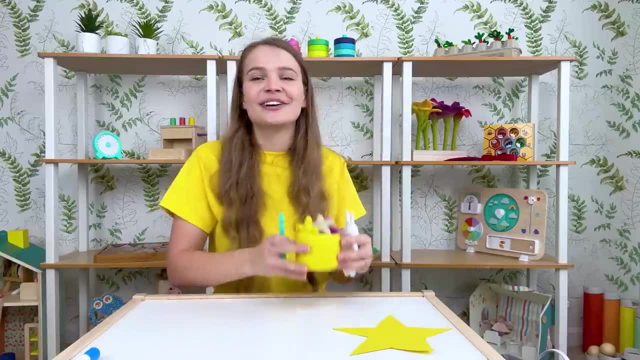 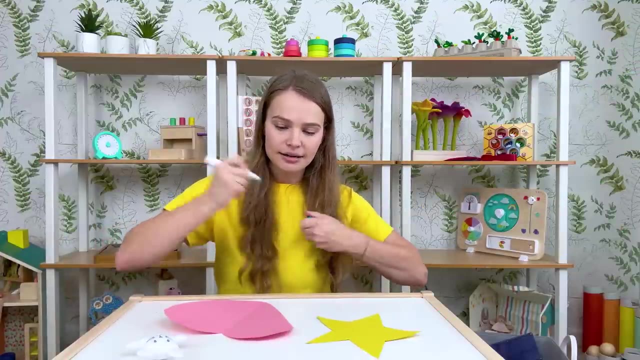 Pink one in, And how about? well, this one's kind of a white beige color. Let's put this one in. All right, Thanks for helping me put all the stars in. Thank you. Let's draw our happy faces on our star in the heart. 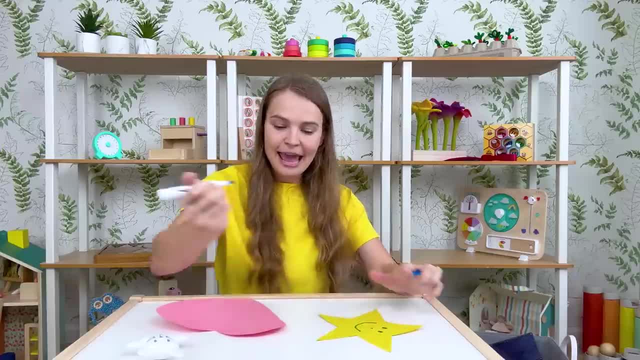 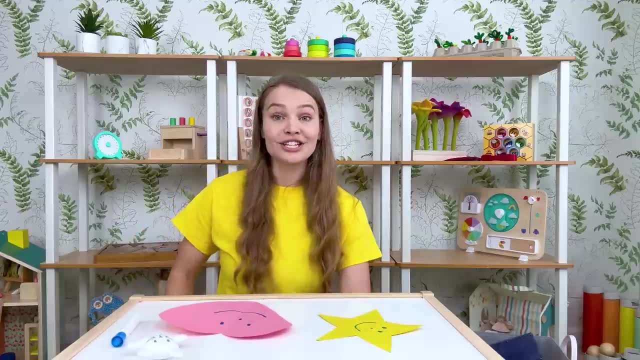 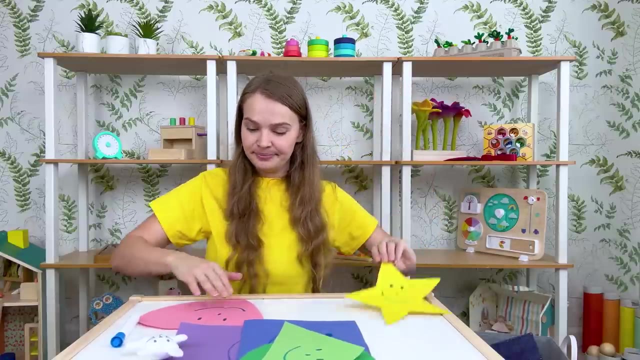 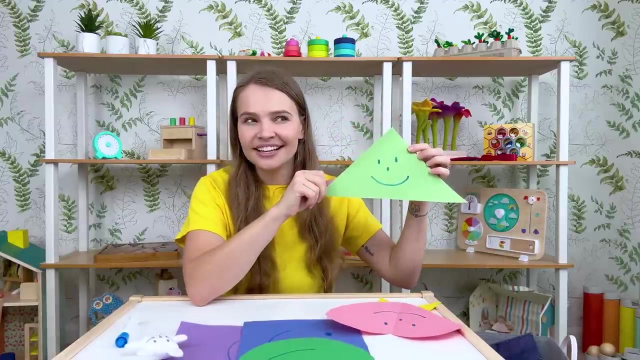 And so we'll have all of the happy shapes together: Eye, eye, nose, mouth. Let's look at all of the shapes. we've got Whoa. We've got star heart, and what was this shape? Triangle, Thank you. 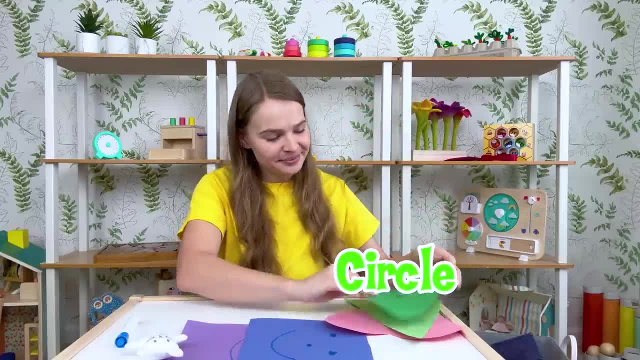 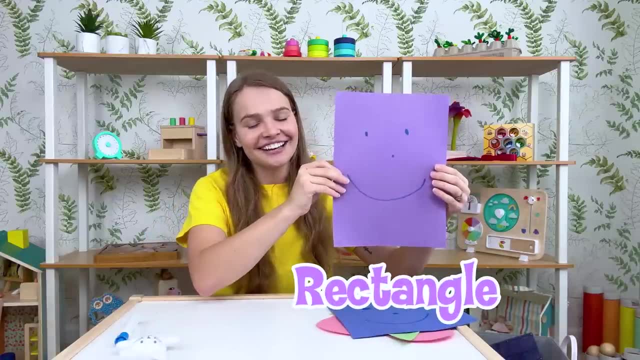 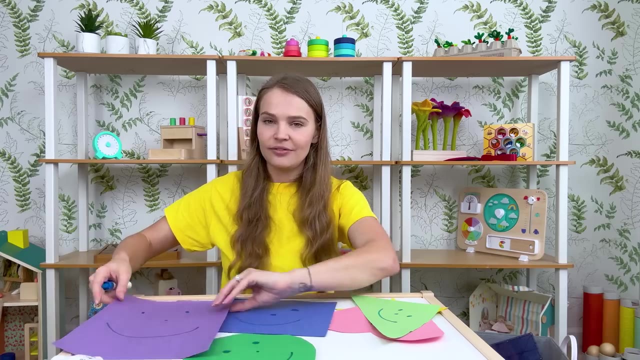 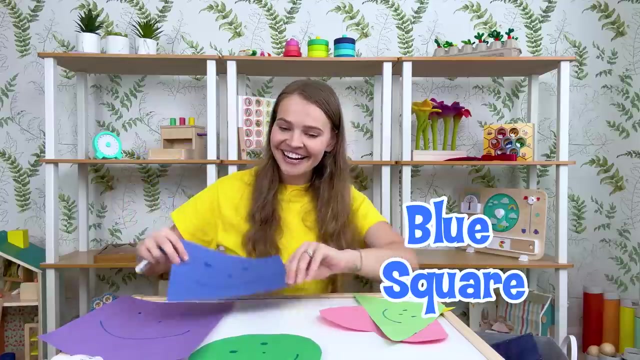 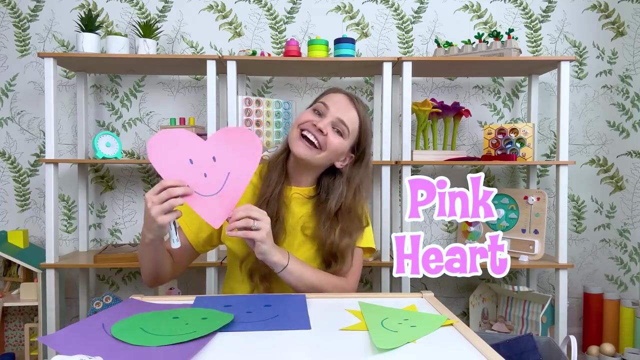 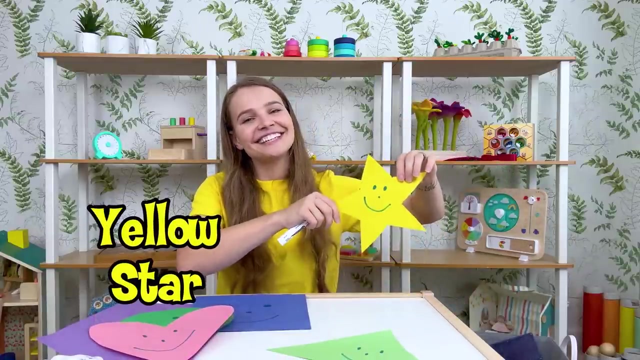 What about this one Circle, circle, square and a rectangle? Wow, You sure know a lot of shapes. Oh, what about all the colors on these? Let's see, We've got purple rectangle, blue square, a green circle, a pink heart, a green triangle and a yellow star. 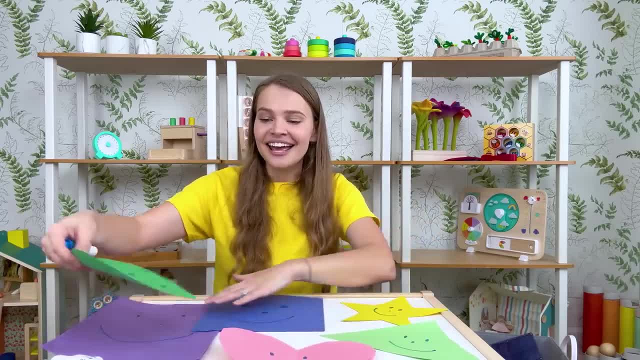 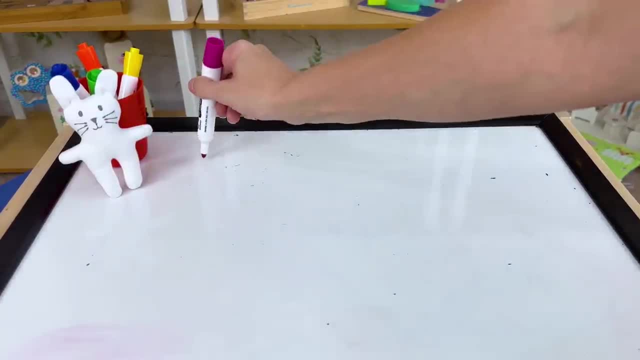 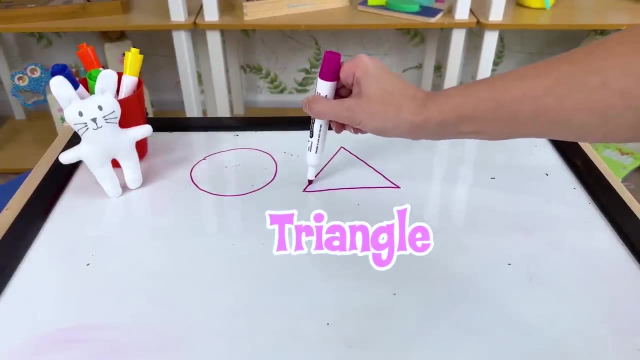 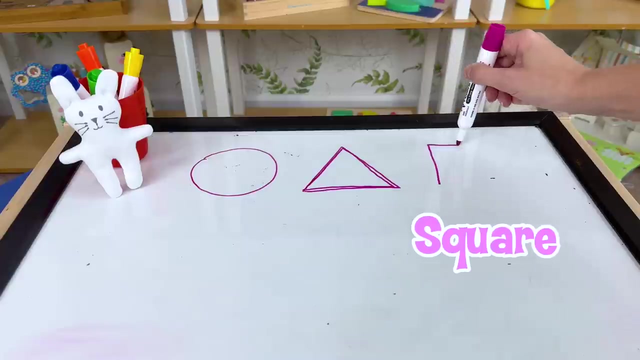 Wow, So many shapes. You're really smart. Thank you so much for helping me. Let's draw all the shapes that we learned for Bunny. Here is a circle. A triangle has three sides: One, two, three. A square has four sides. 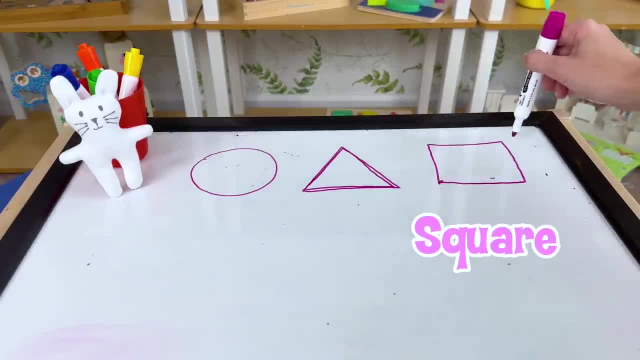 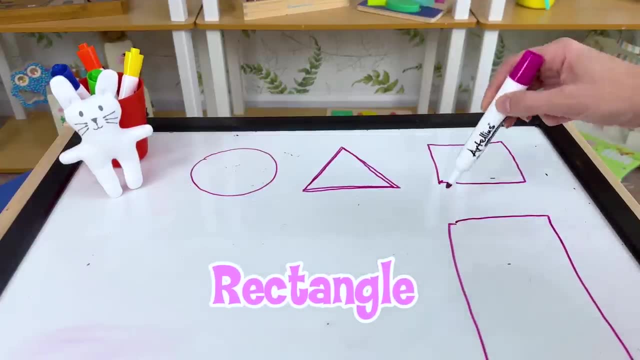 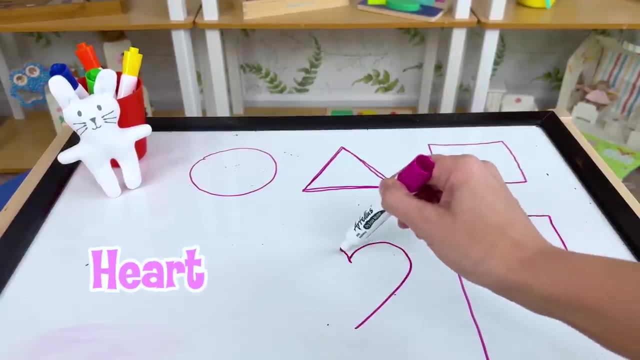 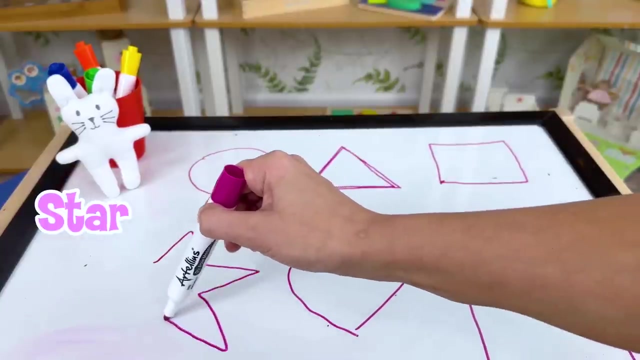 Two, three, four, And they're all the same. A rectangle is similar to a square, but it's long. It's got two short sides and two long sides. We also learned about a heart and a star. Here is a star. 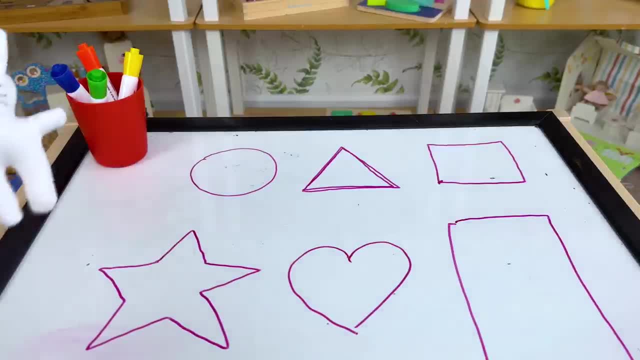 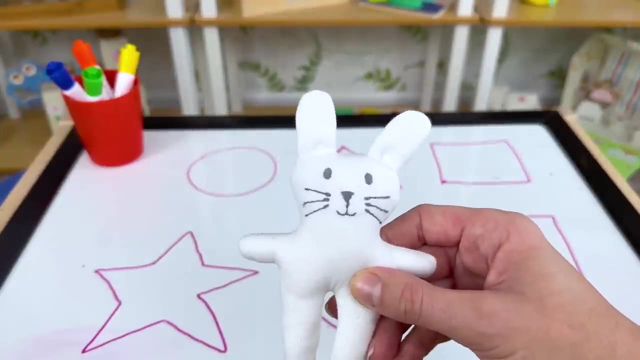 Let's help Bunny find the shapes, Okay, Okay, Will you help me? I'm looking for a heart. Do you see a heart? Hmm, Right here, Bunny. Yay, I'm in the heart Now. do you see a star? 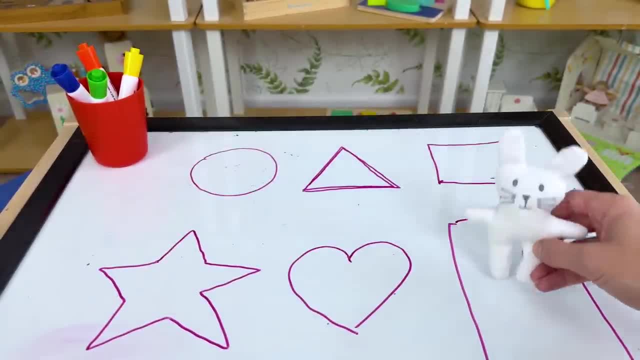 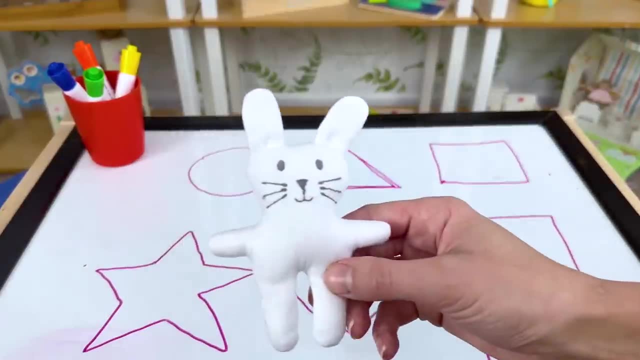 Hmm, Where is the star? This is a rectangle. Right here, Bunny. Hop, hop, hop, I'm in the star. Now do you see a circle? Hmm, Right here, Here you go, Bunny. Thank you. 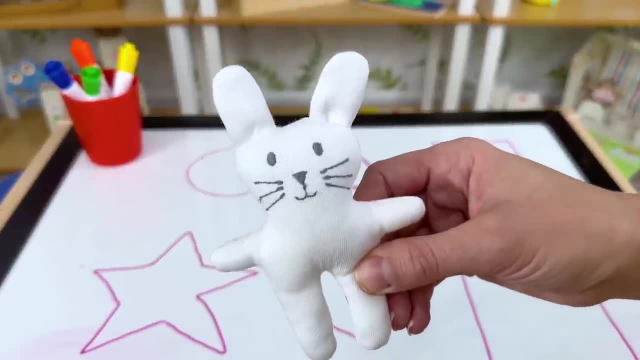 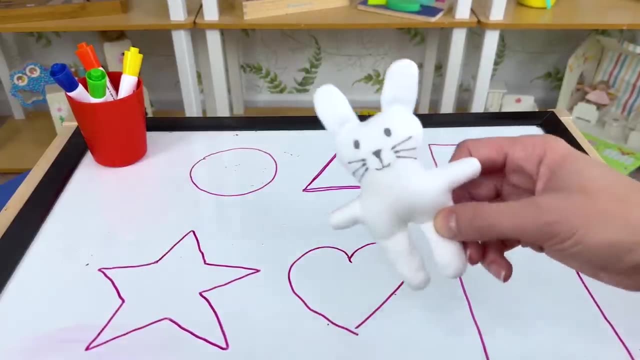 Thank you. Do you see a rectangle? Hmm, Right here, Bunny. Here we go. Thank you, Thank you. Do you see a triangle? Hmm, Right here, Bunny. Thank you, Thank you, Thank you. Now. do you see a square? 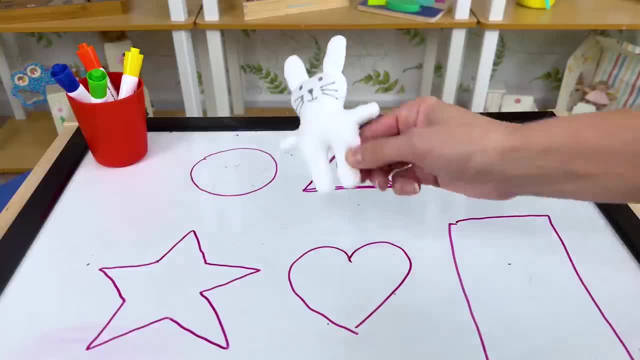 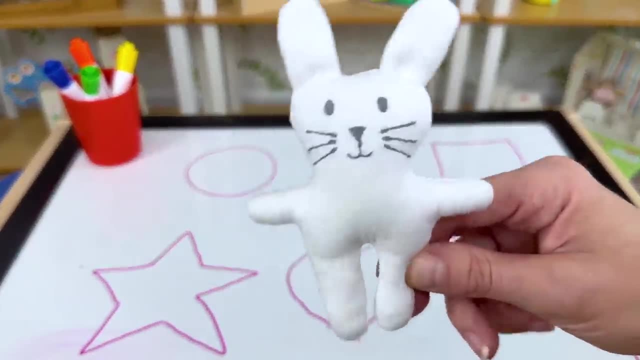 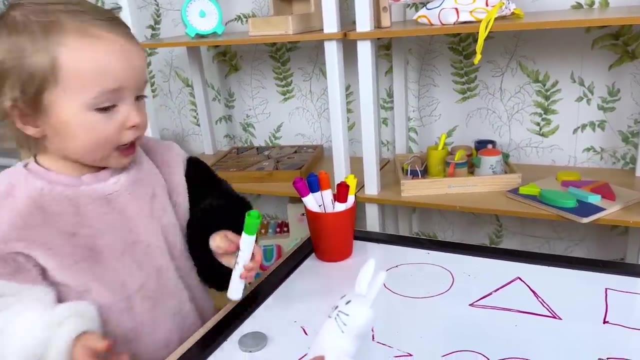 Hmm, Right here. Wow, Thank you for helping me find all of the shapes. Thank you, Thank you, Thank you. What shape are you going to draw on? Let me see. What shape are you going to draw? Can you help? 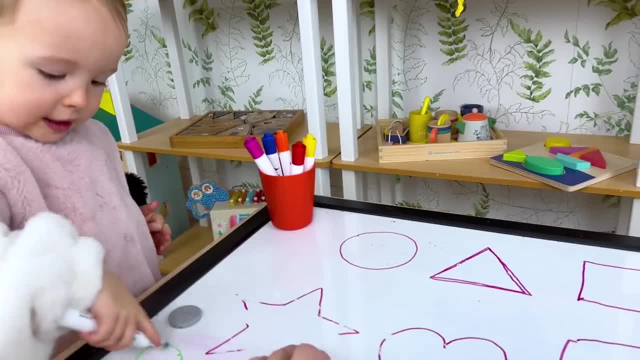 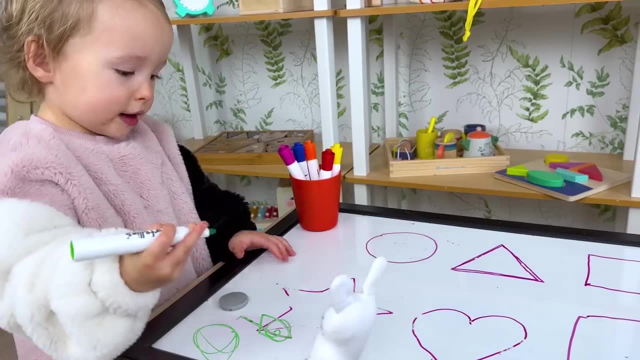 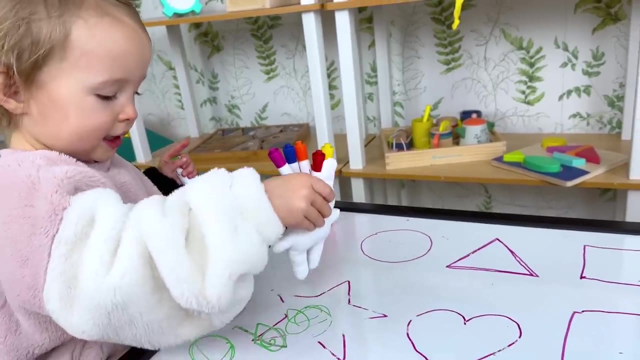 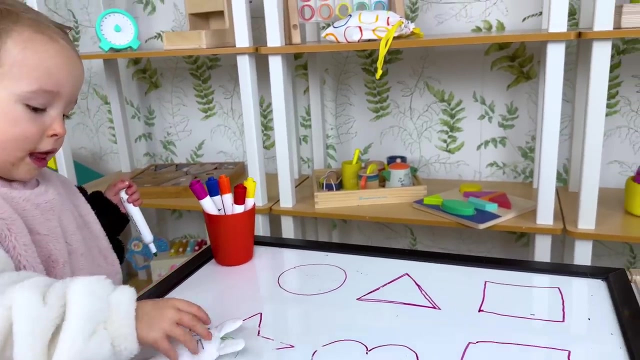 Yeah, let me help you. take this off. You're very welcome. What shape are you going to draw? Ooh, Do you know how to draw a circle? Oh yeah, You want to sit in the circle there, Bunny-O. 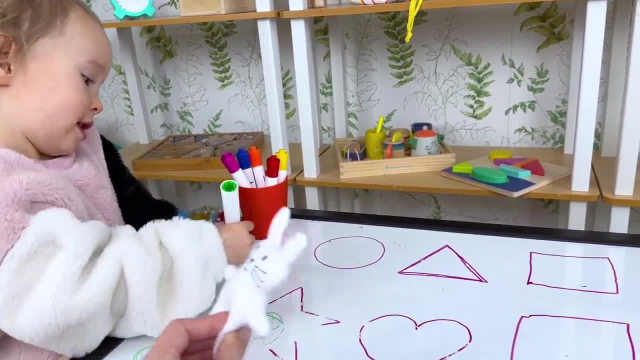 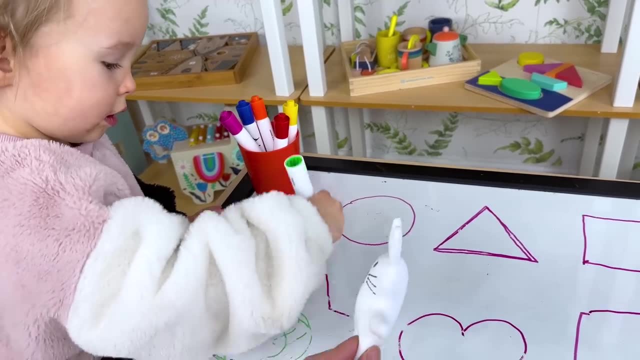 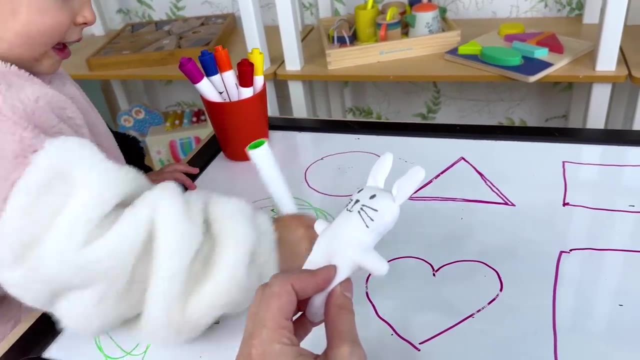 Peasy-O, do you know how to draw a happy face? Yeah, Yeah, will you draw it for me? That's a good mouth, Good nose, Good hair. Aww, Cute hair, tie Pretty Two. How many more shapes we've got. 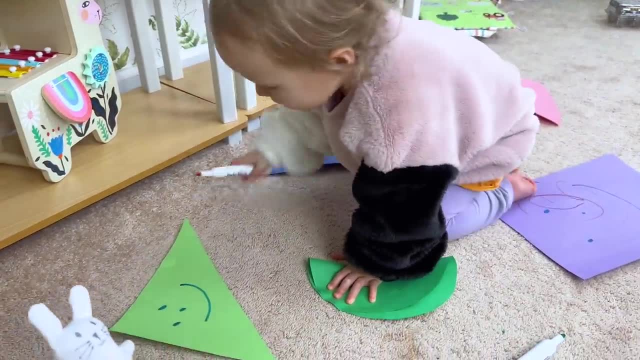 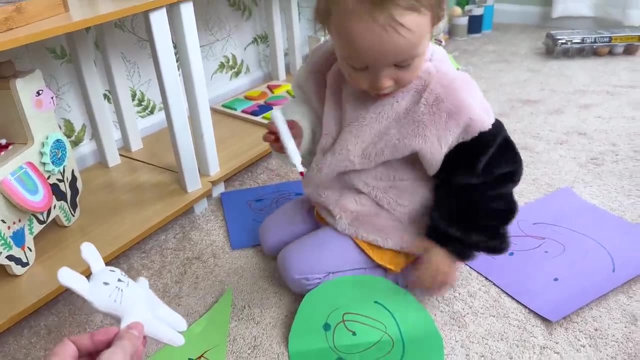 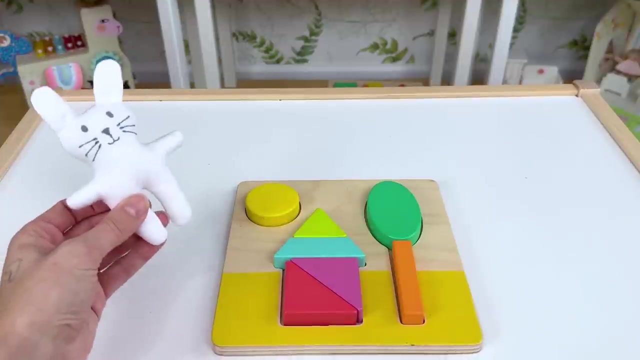 One, two, three, four, five, That's many. Now, what shape is this Peasy-O Triangle? That's a good triangle. Have you seen the heart? Oh, wow, Let's help Bunny with this puzzle. Let's look at all. 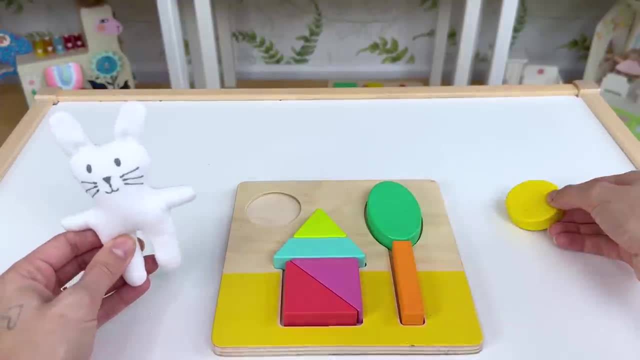 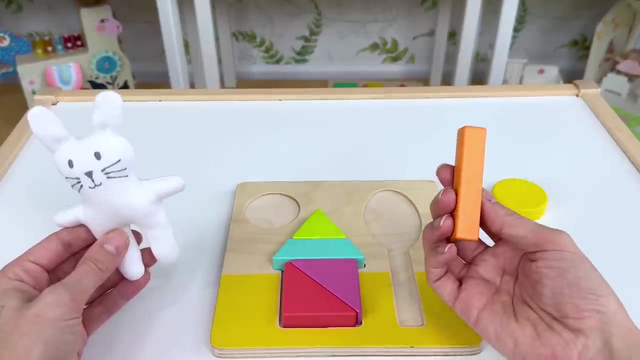 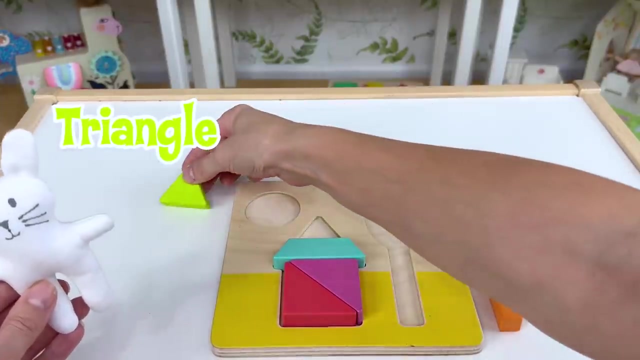 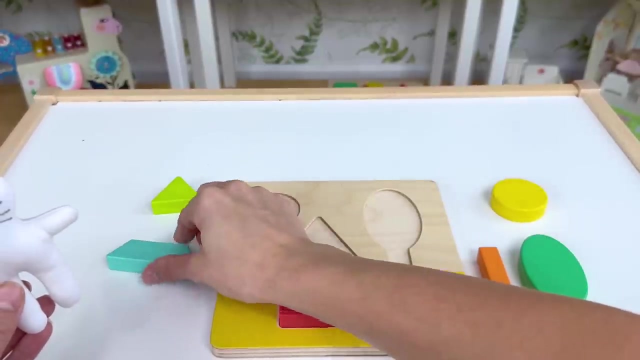 the shapes We've got: a circle- Ooh, I like circles as Bunny- An oval. A long rectangle stick. A little green triangle- This one's called a trapezoid, It's got different sides and four corners. A pink triangle: 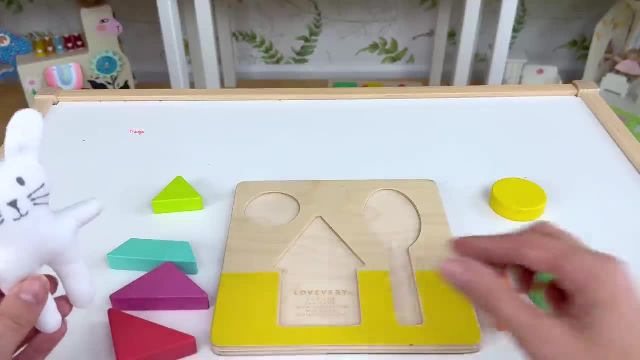 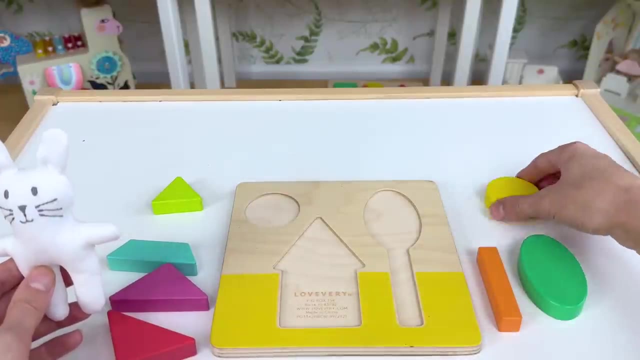 And a red triangle. Now let's put them back in. Let's see, We've got a little tree, a house and the sun. Hmm, Do you see a spot for the circle Right here? Let's put it in. 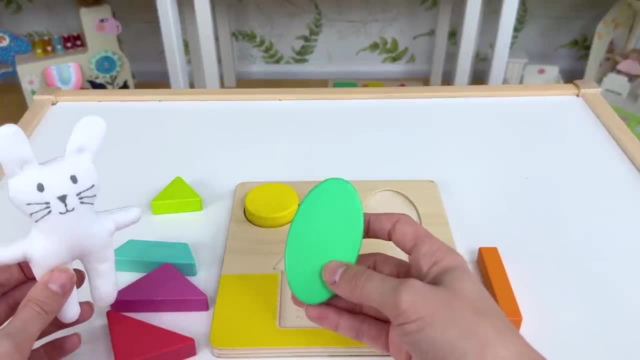 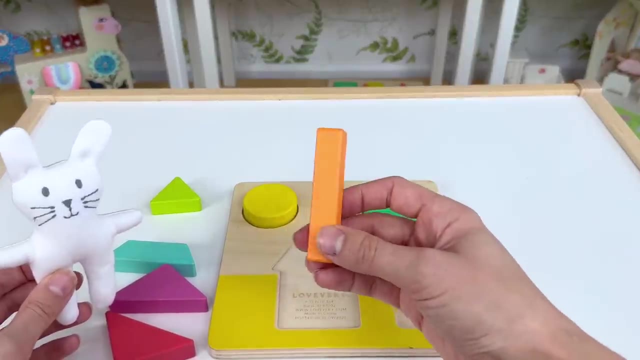 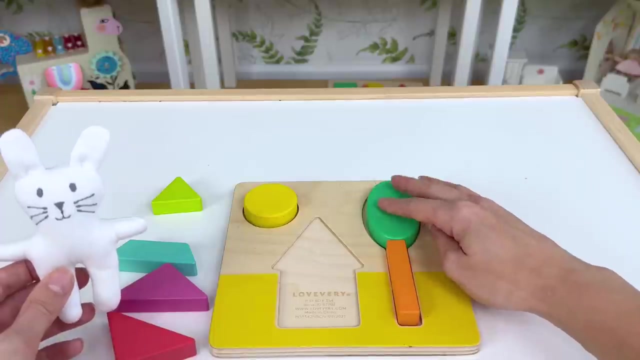 How about this oval? Do you remember where this was? Hmm, Oh, this looks like a shape for oval, but slowly in. How about this orange long rectangle Right here, as the stem is the bottom of our tree? I guess it's the tree's trunk. 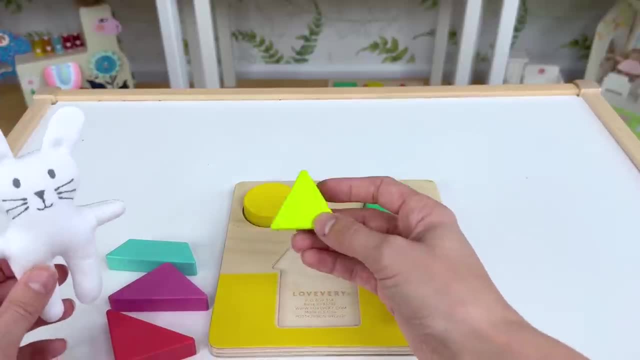 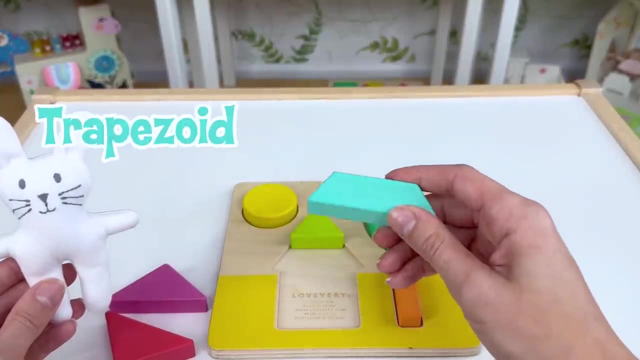 Let's see next. How about this little triangle? We'll put it at the top of the house, at the roof. Now we've got this trapezoid for the bottom of the roof And this looks like a square, but I 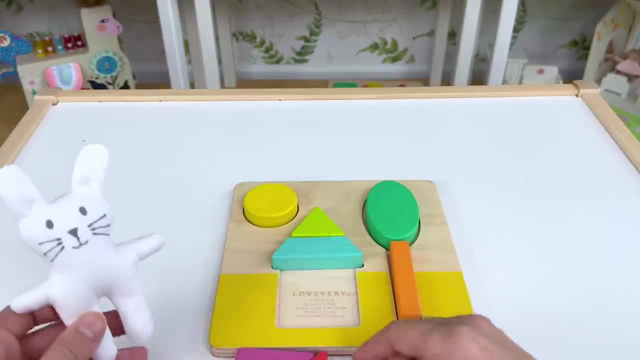 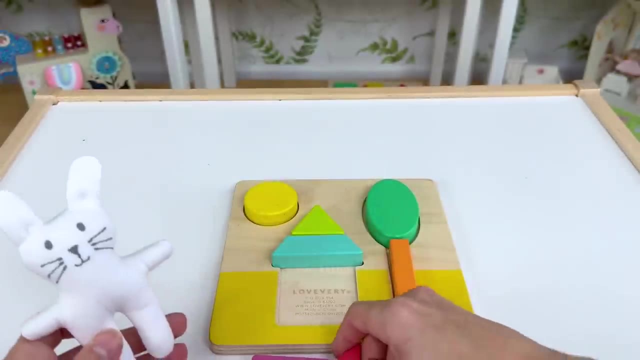 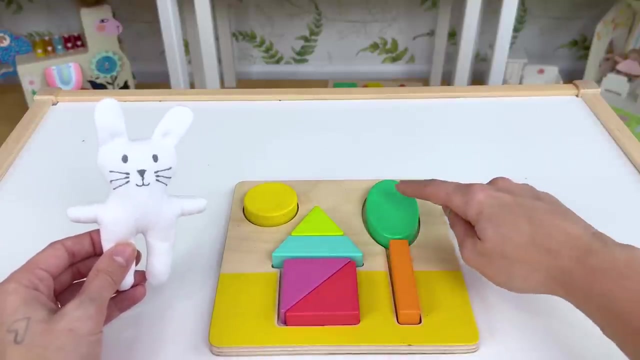 only have two triangles. Hmm, Oh well, look at this: When these triangles are together, they make a square, So let's put one triangle in and another triangle in. Oh wow, Now we've got a house, the tree with the trunk and the sun. 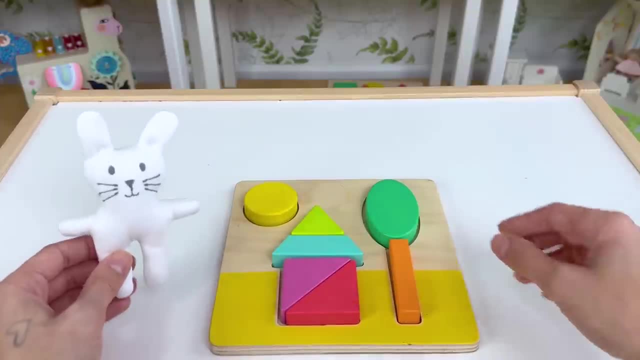 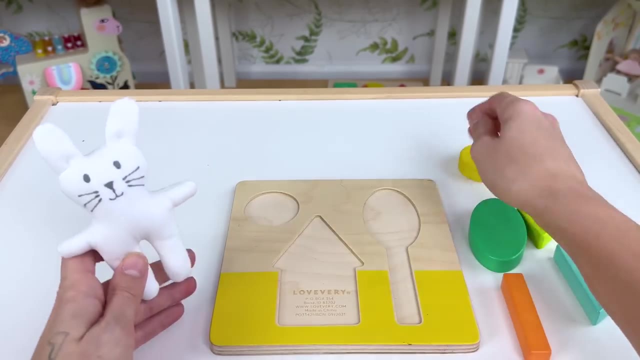 all made out of different shapes. Wow, Great job Bunny. Great job you for helping us. Another great thing about shapes is that you can make different stuff with it. So first it was a house and a tree, but it can also be a boat. 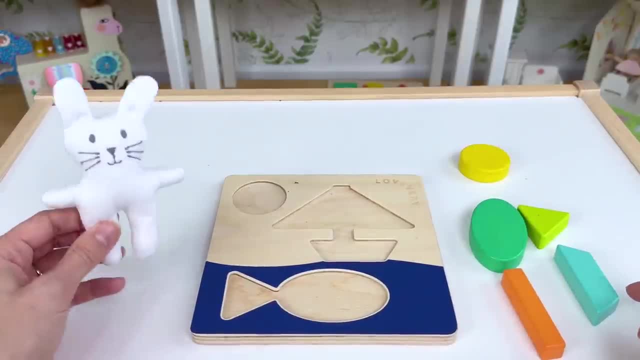 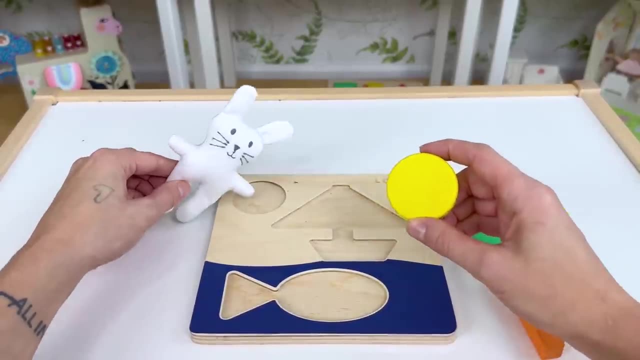 a fish and the sun. Let's see if we can help Bunny put these shapes in. All right, Do you see a spot for the circle? Bunny says: yeah, yeah, right here, Here you go, Bunny. All right, Bunny. 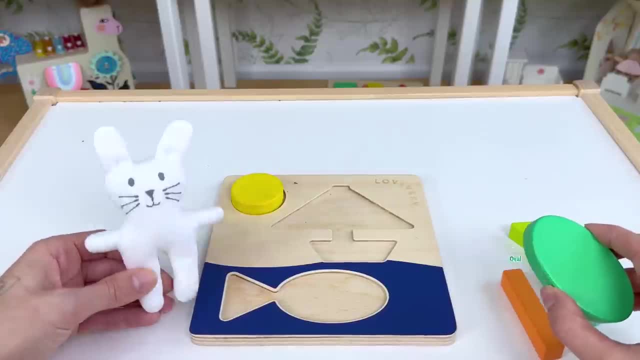 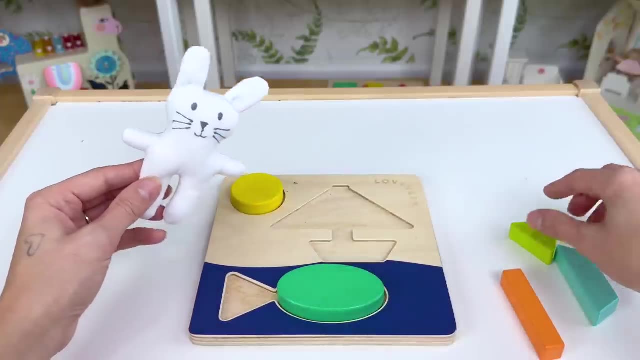 Do you see a spot for the oval? Hmm, This looks like a triangle. Hmm, Oh, right here, right here, right here, Here you go, Bunny. Oh, what about the fish's tail? Oh, maybe a triangle. Yeah, 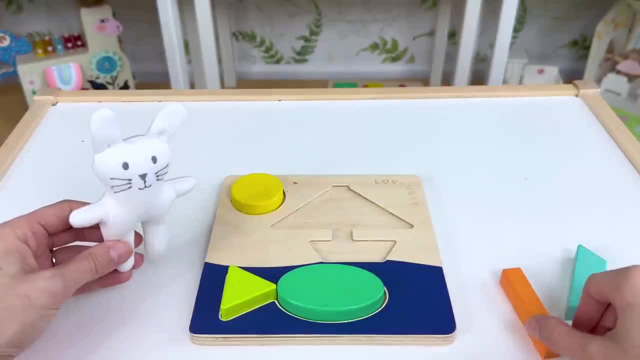 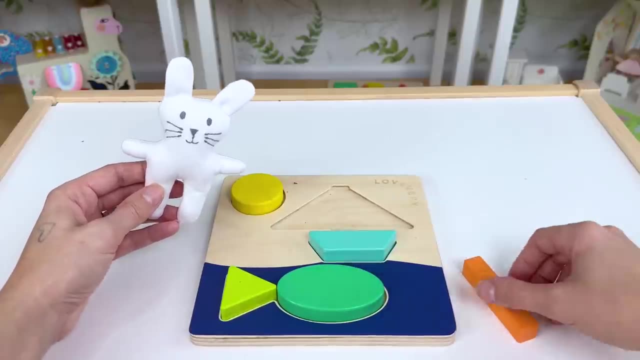 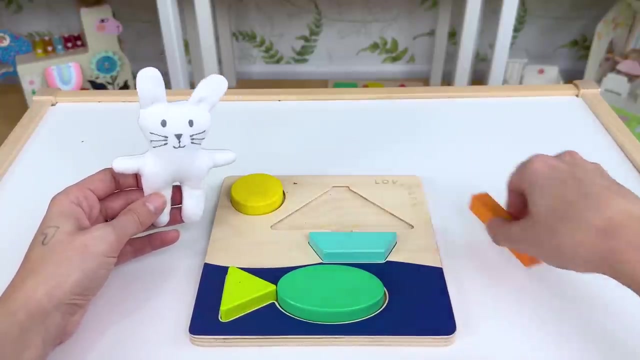 Bunny, good idea, We'll put it in. Let's see Now. the bottom of this boat looks like this trapezoid. Let's see if it fits. Hmm, How about this rectangle? Doesn't seem to go. Maybe let's try a triangle first. 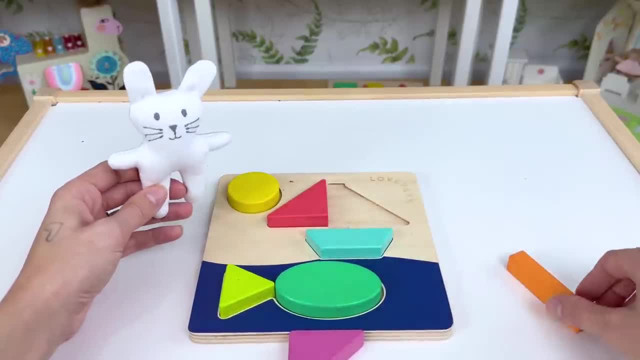 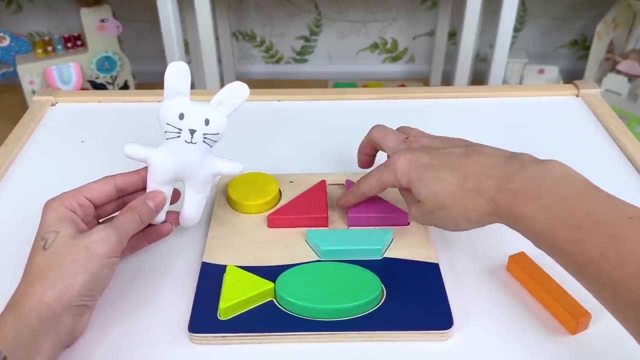 How about this one? Let's put it to the side here. Okay, Bunny, Looks like the other side, maybe could fit a triangle too. That's not working. Let's see Turn, turn in And the rectangle up top. 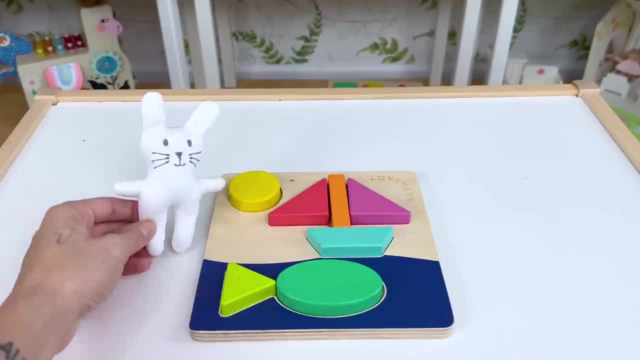 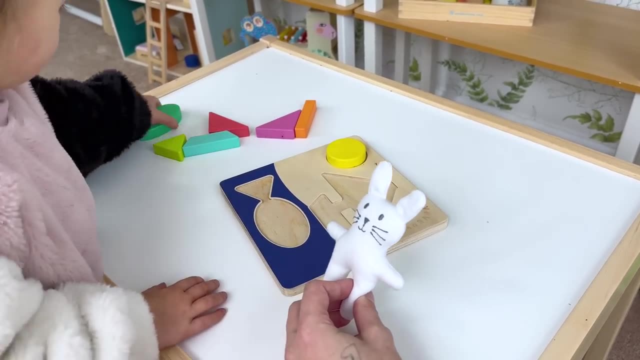 Wow, Bunny, great job putting the boat, the sun and the fish together. Thank you for helping me. Will you help me with this puzzle? Where does the fish go Over over here? You got an oval. What else? A triangle. 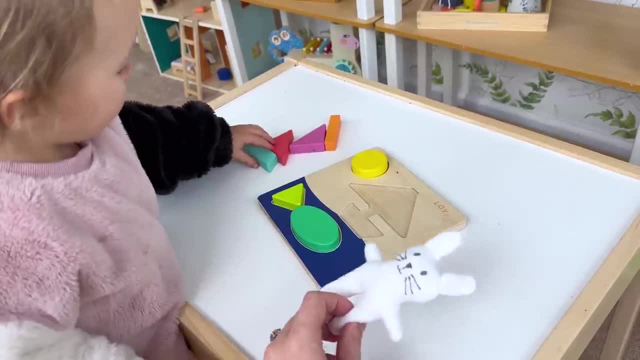 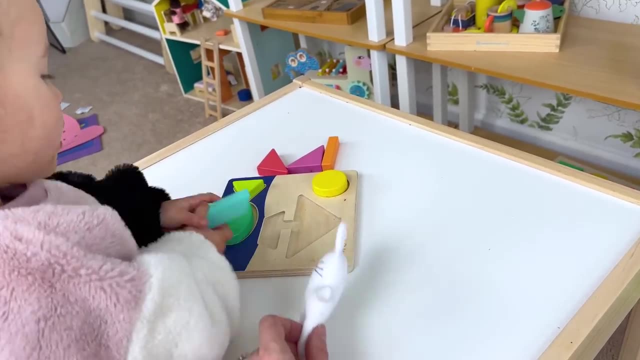 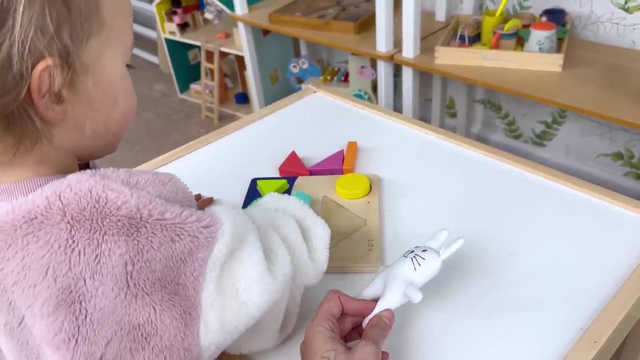 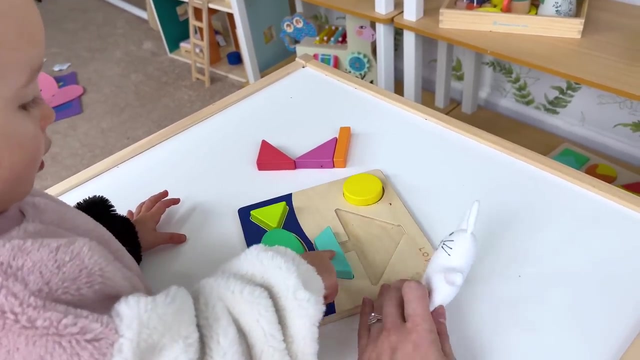 In the back, Oh, in the back, like that, like a tail, And Oh, turn it. I like that, Turn it over here. Oh, pretty Yeah, boat, That's the bottom of the boat, I like it. Now, where do the triangles go, Paisley? 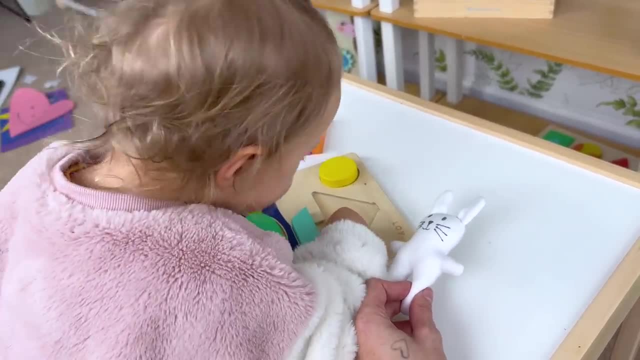 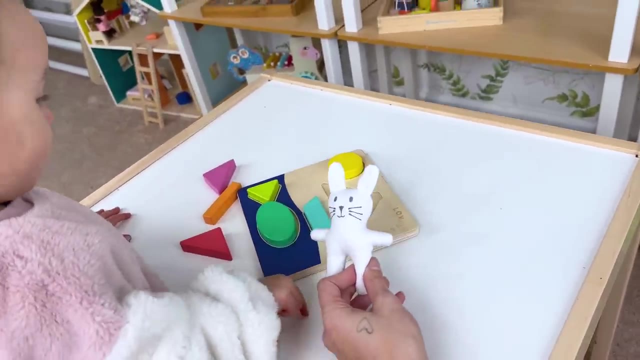 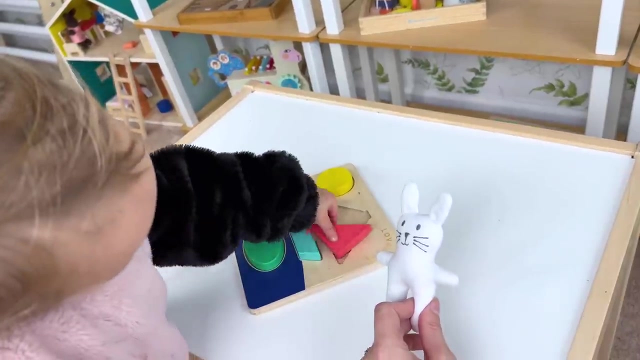 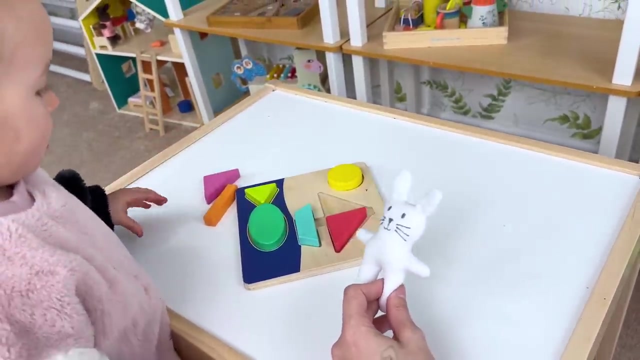 Oh, hmm, It's in the bottom boat over here. Oh, that's the bottom. How do I put them in? Try doing it this way. Oh, that way. Slowly do that. Oh, slowly in. I like that. What about the other? 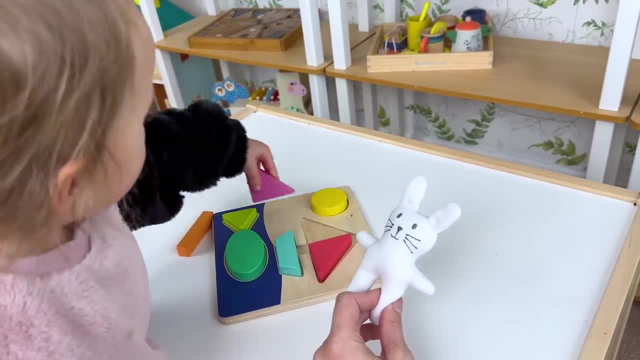 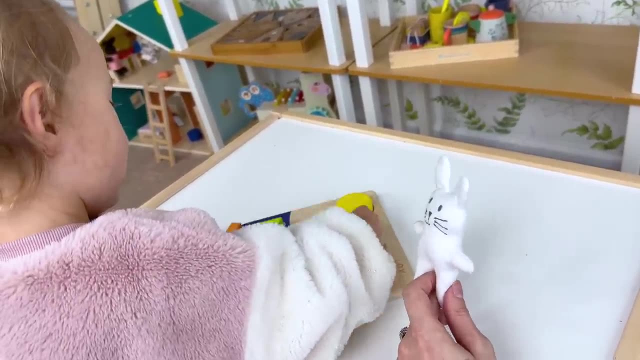 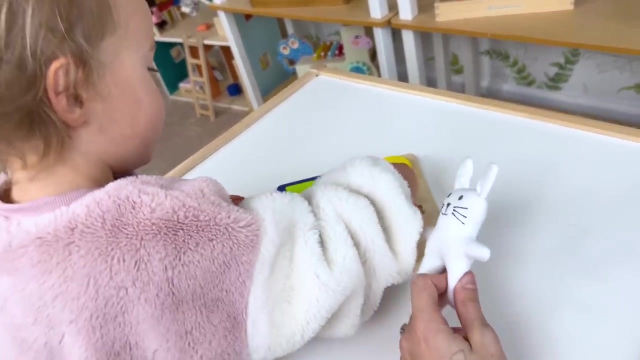 triangle, Bottom, bottom. This way: Top to the top, Oh, top to the top, and bottom to the top, Bottom, Oh, bottom, Oh, okay. Well, what about that orange piece? Where does that go Over here, Oh? 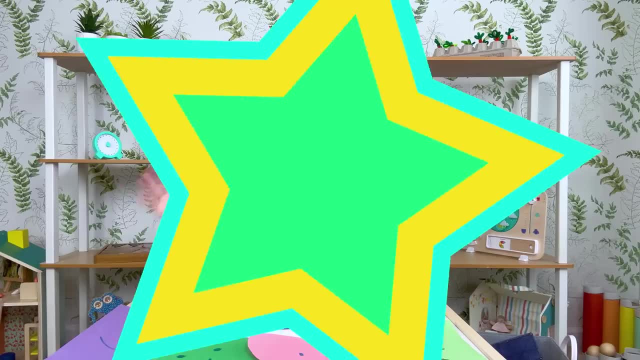 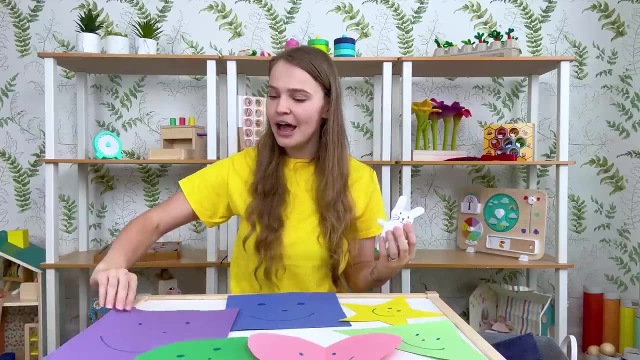 wow, Thank you for helping me put all the shapes in Paisley. Oh wow, This was so much fun. Thank you so much for helping me and helping me to learn all about the shapes. Now we know what a rectangle is. 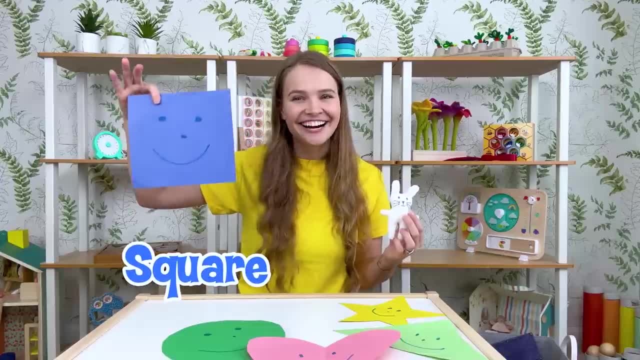 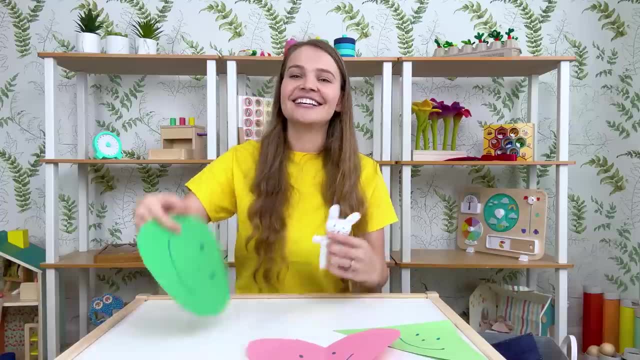 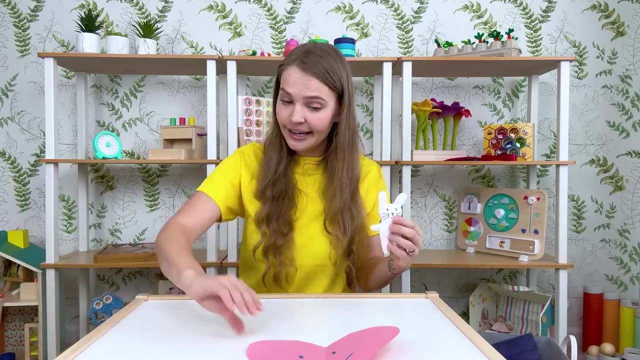 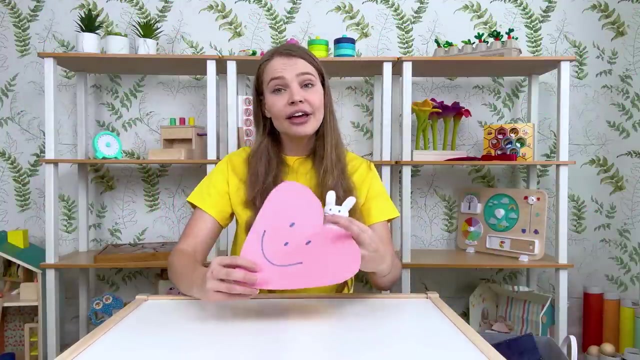 We know what a square is, We know what a star is, We know what a circle is, We know what a triangle is And we know what a heart is. And this is a little heart card for you, because I'm so thankful that you're playing with me. 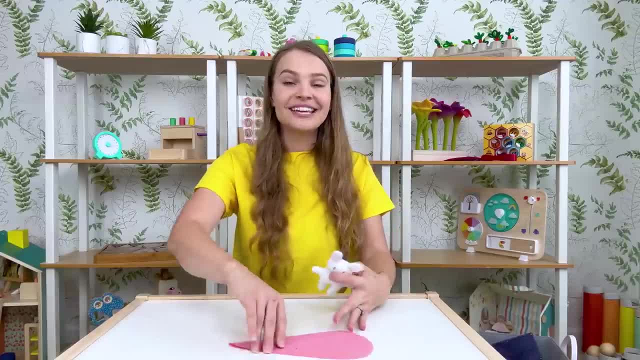 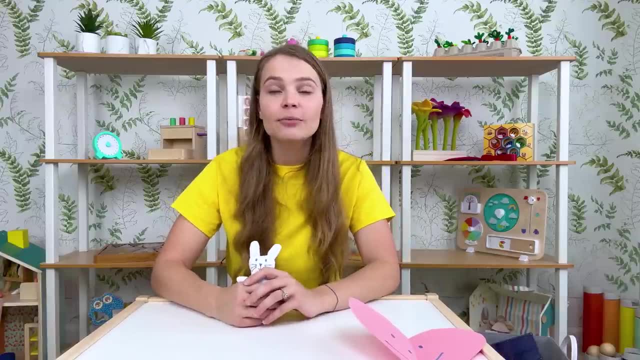 and you spend your time with me And I think that's really cool. So here's a heart card for you. Here you go. Thank you so much for playing with me and for learning with me. I love learning and I love playing with you. We did a great job helping.